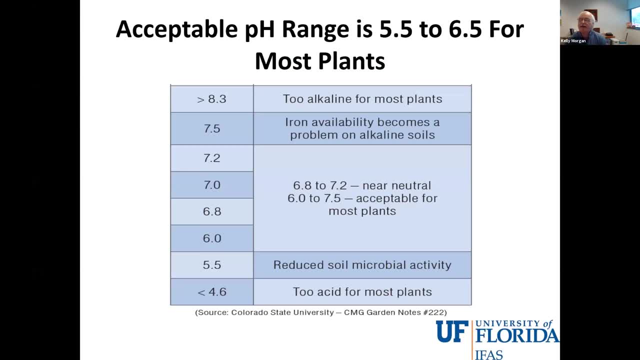 I got it So, as most of us know that most crop plants the acceptable range of pH might not be planned. Most crop plants will have a if we don't have enough pH. pH is somewhere between 5.5 and 6.5, something just short of neutrality, And you can see there. 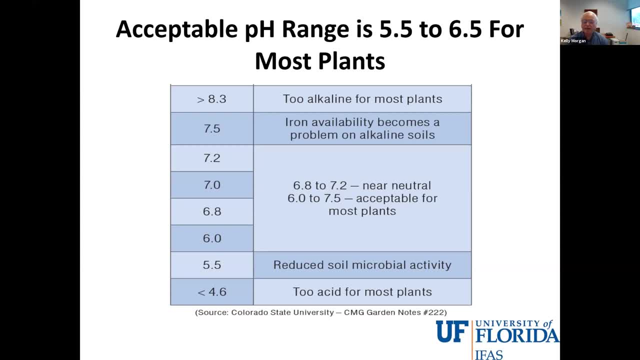 that. the reason for that is that the nutrients for plants are most readily available in that range. As you go towards the bottom of the scale, more acidic, lower pH. it's too acidic. The nutrients become bound to the soil in various ways, And we'll talk about that. 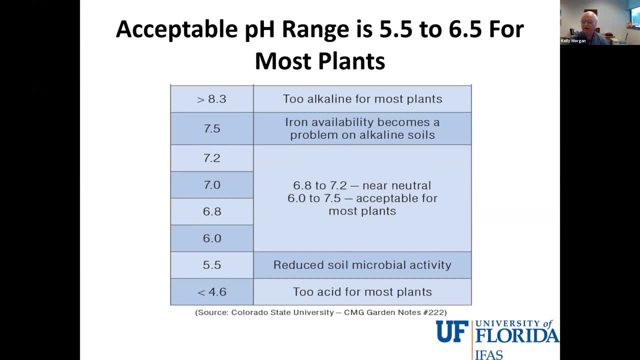 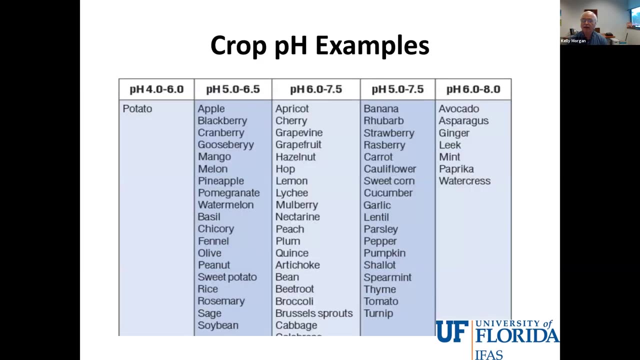 As you go up in the scale or higher pH values, it becomes alkaline, And the same is true, but in a much different way. So we'll explore all of these things. going through the talk today, I found this example of recommended soil. 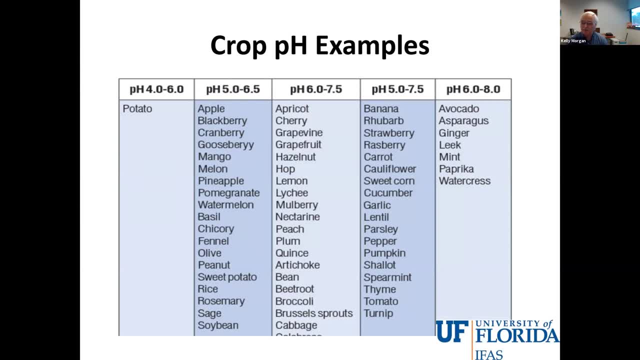 pHs for various crops And, as I mentioned before, most of them, you can see, are there in that upper 5 to 7 range for majority of crops grown throughout the country. There's a few exceptions to that, some that like it a little more alkaline, such as avocado and asparagus, and some that 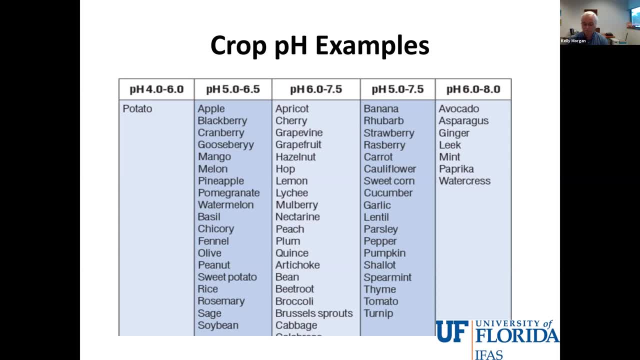 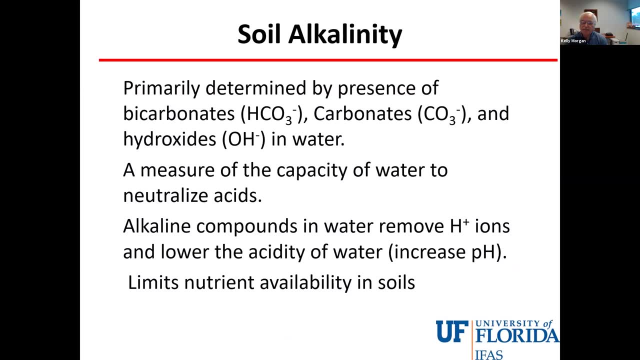 like it a little more acidic, and that's primarily potato. I'll concentrate mostly on alkalinity And that's the bigger factor in Florida soils, particularly in South Florida. Our soils are becoming more and more alkaline, primarily because of our source of water, But this is true throughout the state where water. 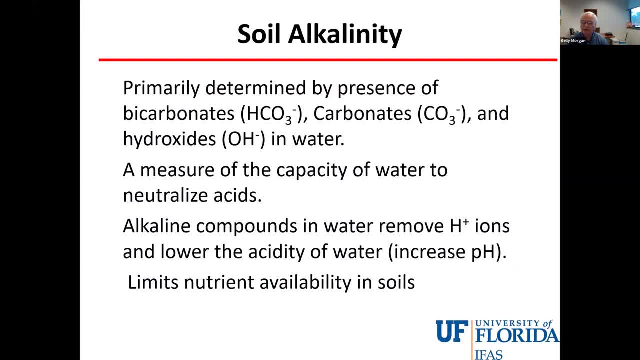 from limestone aquifers are used for irrigation. Now, if you're using surface water, this isn't as important, But a lot of our irrigated agriculture is now coming from deep wells down into the limestone, And along with that water comes a lot of bicarbonates And this makes for alkaline. 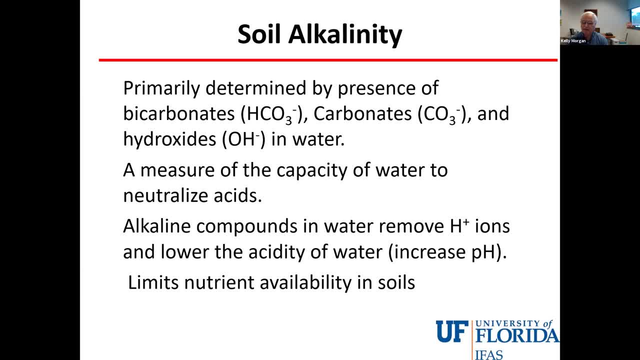 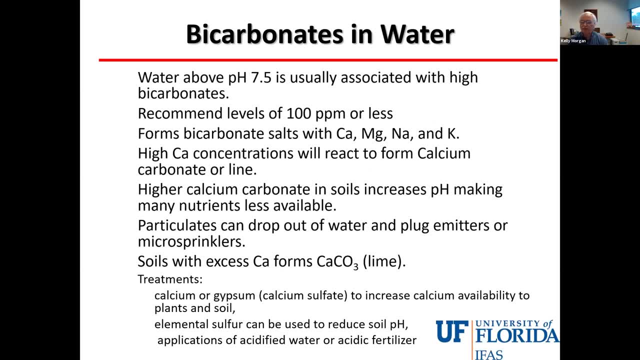 soil alkaline water and it causes the soil pH to increase. If you're water, if you're irrigation water is above 7, certainly if it's above 7.5, it's usually associated with bicarbonates. You should have your water tested. Recommended levels are typically in the 100 parts per million. 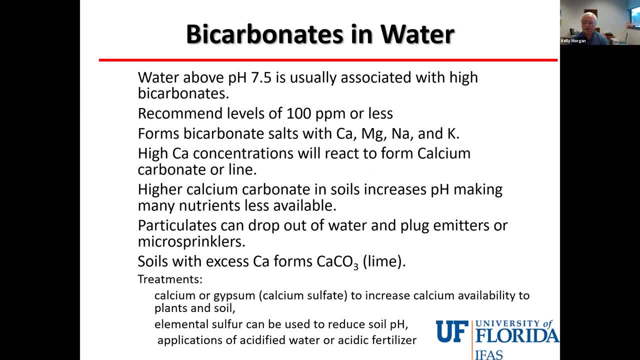 of bicarbonates or less. if you test your water through testing labs, The form of bicarbonate salts typically are calcium, magnesium, sodium and potassium, So you'll see high bicarbonates, but you'll also see high amounts of these four nutrients in your water. 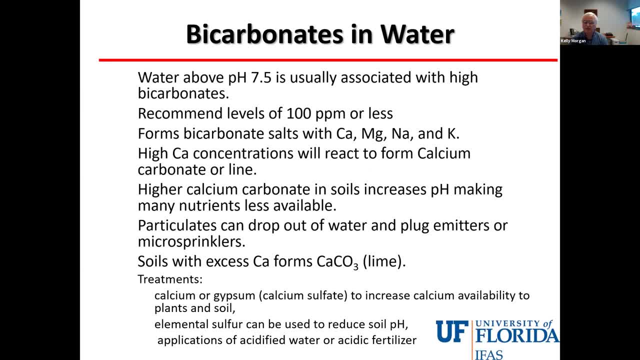 And as we go through the discussion today, you'll see why this becomes important, Because the pH of your soil is increasing slowly over time and you need to bring that back into that productive range of 5.5 to 6.5 for most crops. So that's why this becomes important. So that's why the pH of your soil is increasing slowly over time and you need to bring that back into that productive range of 5.5 to 6.5 for most crops. 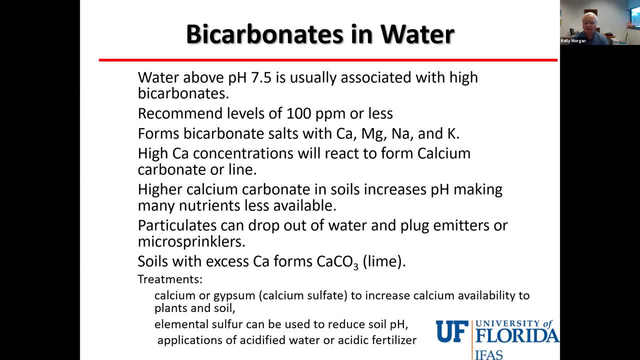 So that's why this becomes important, So that's why the pH of your soil is increasing slowly over time and you need to bring that back into that productive range of 5.5 to 6.5 for most crops. And there are several ways of doing that: either through applications of 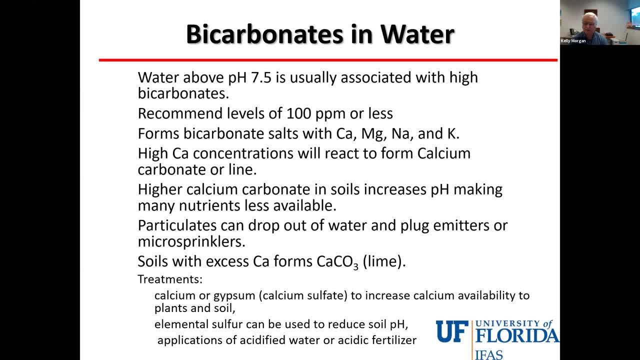 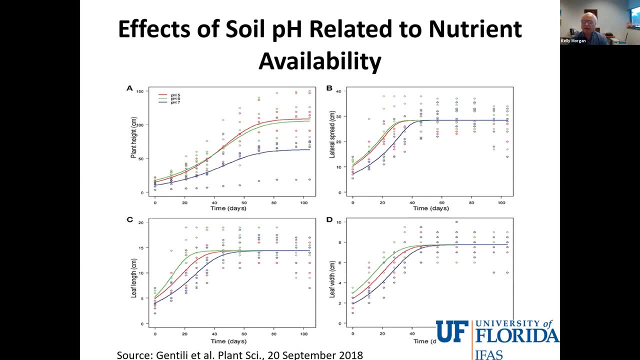 lime or gypsum if your soil is too acidic, or sulfur and other acidifying fertilizers if your soil is too alkaline. Just to run through a few of the implications of a high pH- this graph here- the plant height has decreased. If you look at the information on the internet, there was a study looking at the effect of crop height- bean plant in this case- at different pHs. You can see that as you get to a neutral pH- the blue line- the plant heights decrease as through the production cycle. 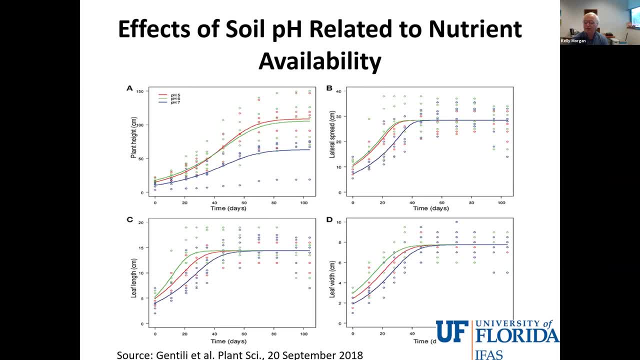 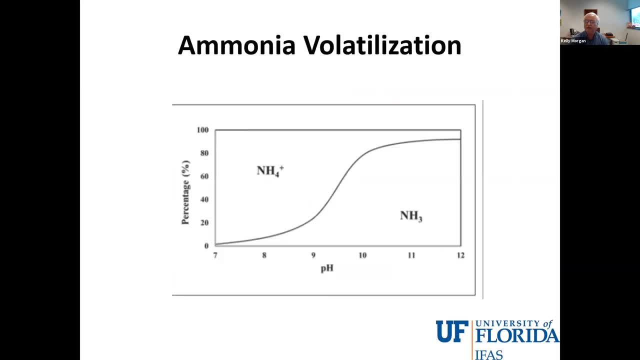 Initially that's true on lateral spread of the plant, leaf length and survival. Initially that's true on lateral spread of the plant leaf length and survival and leaf width. the crops just don't grow as well at that higher pH. 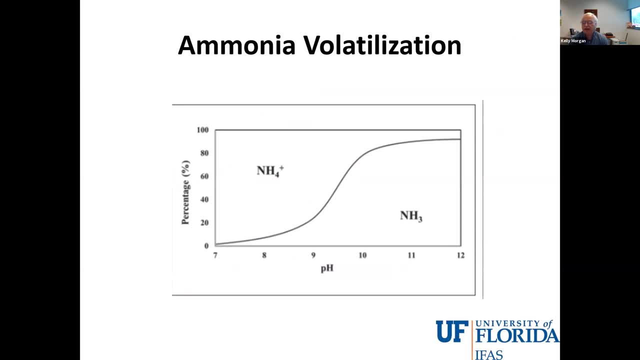 Some of the reasons for this is that you have different impacts on your fertilizer components. If you're applying an ammonium source of fertilizer at a low pH, your fertilizer stays in the ammonium form. Once you cross neutrality at seven and you increase the soil pH, the ammonium turns to. 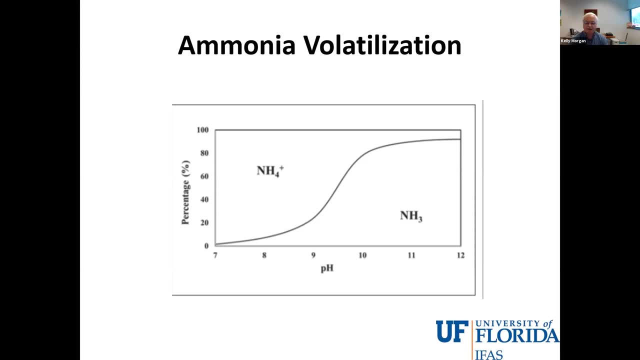 ammonia and that can volatilize through our soils. our porous soils, Our sandy soils allow the ammonia to release into the atmosphere and you're losing your nitrogen source at that point. Not recommended to apply only an ammonium form at a pH above seven. 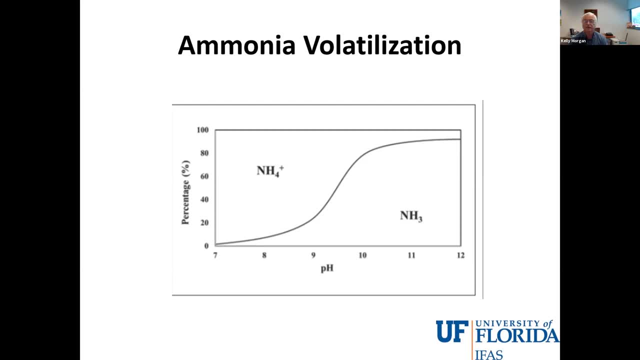 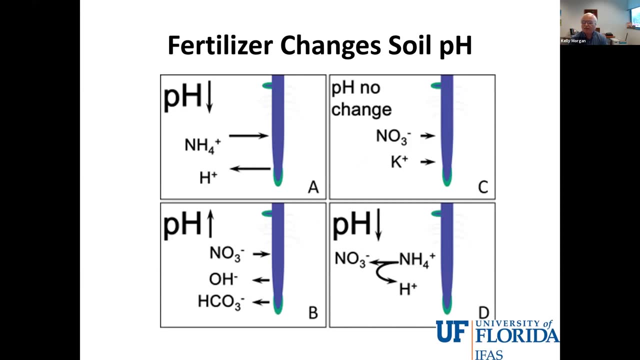 So this has to be taken into consideration with our recommendations. pH has a great effect on the uptake of fertilizer components. In this graph you can see that the illustration there is of a root And then if you have an ammonium source, roots take up that ammonium source. 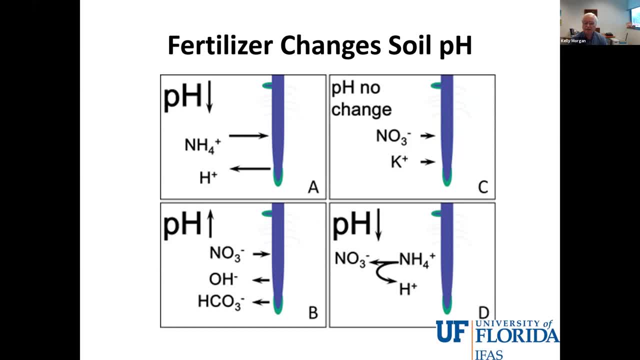 It has to expel a hydrogen ion to do that, to balance the nutrients, to balance the charges. This is very important. The root must account for its charges. So if it brings on a positive ion, it has to expel a positive ion. 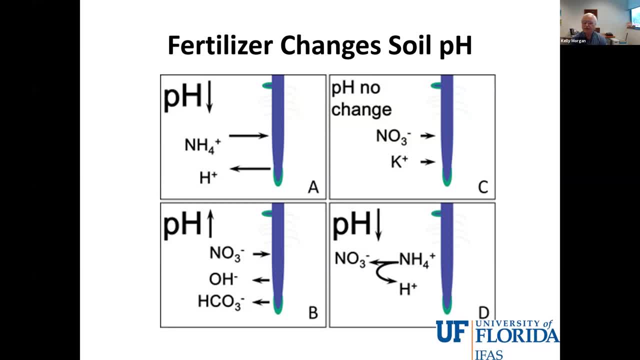 So by expelling the hydrogen it causes the soil pH And then by expelling the nitrogen it causes the soil pH. So this is the way you can take the nitrogen source and see how far it can go If you have a combination of nutrients like in panel C there where you have an anion. 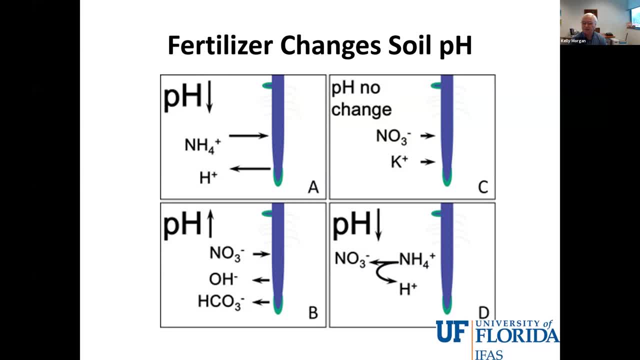 and a cation, then there's no net change because there's no net, no addition of hydrogen to the soil. If you go down to panel B, where you're looking at where they're at, they're not really- You have ammonia, I mean nitrate, going into the soil. 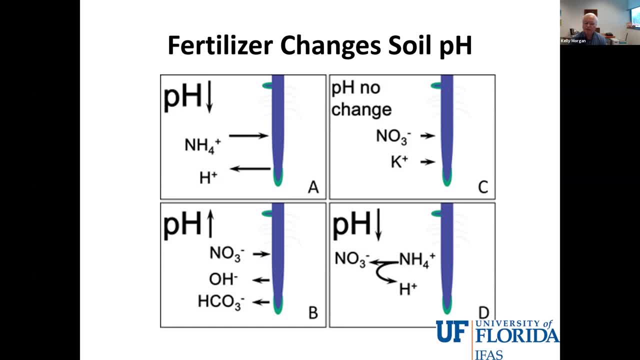 You have hydroxide or carbonates coming out of the soil, out of the roots, and your pH will increase. So what you apply as your fertilizer source has a great impact on the pH of your soil And that, as we'll see a little later on, will influence how your fertilizer changes your soil. 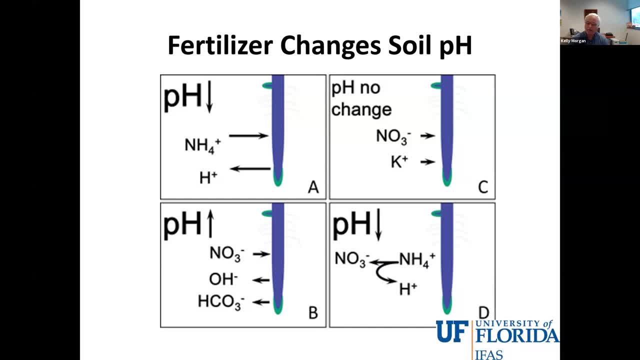 And even going from an ammonium source, as in panel D, from an ammonium source of fertilizer, to a nitrate source, which is something that's unavoidable in our soils. There are compounds that you can apply to fertilizer to reduce the rate at which ammonium is converted to nitrate. 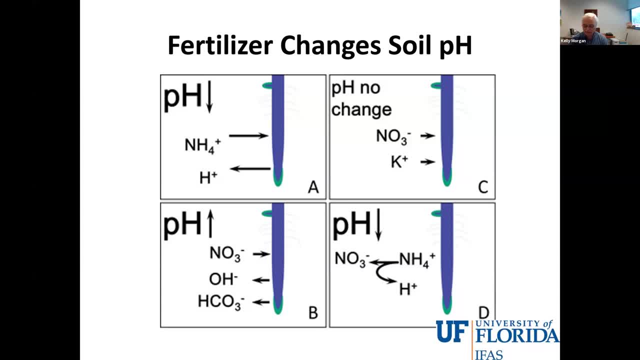 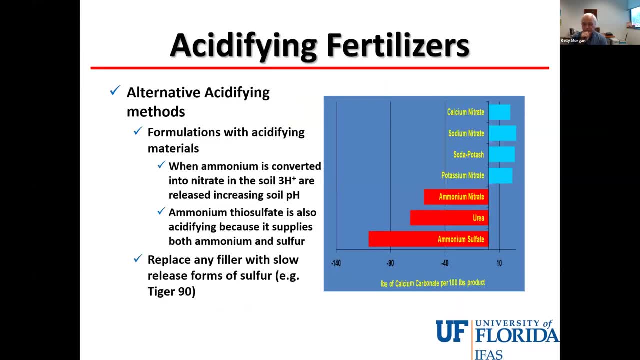 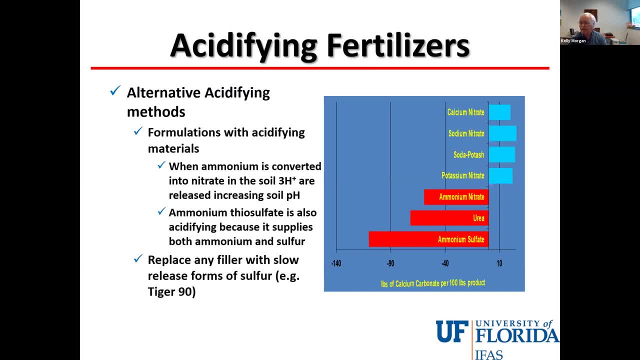 So you see the blue bars at the top. Those are. Those are alkaline-producing fertilizers: calcium nitrate, sodium nitrate, potassium nitrate. those all tend to increase soil pH. Ammonium nitrate, urea, ammonium sulfate- those all 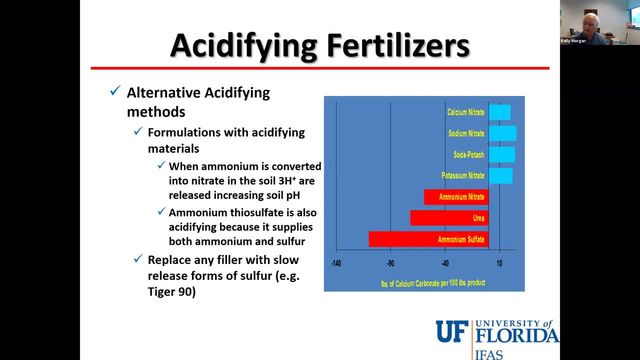 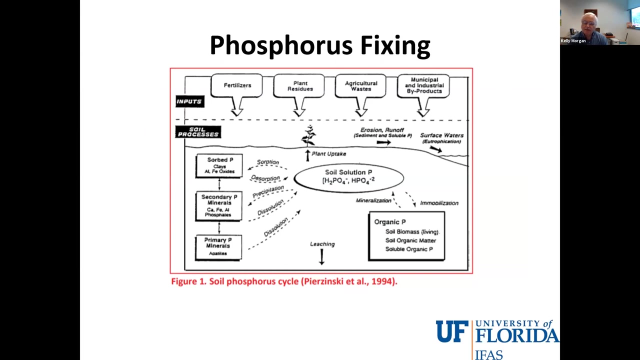 reduce soil pH And you can see by the lengths of the bar. ammonium nitrate acidifies the excuse me. ammonium sulfate acidifies the soil much more than the other two. One of the important things with soil pH is phosphorus, And that's a controversial. 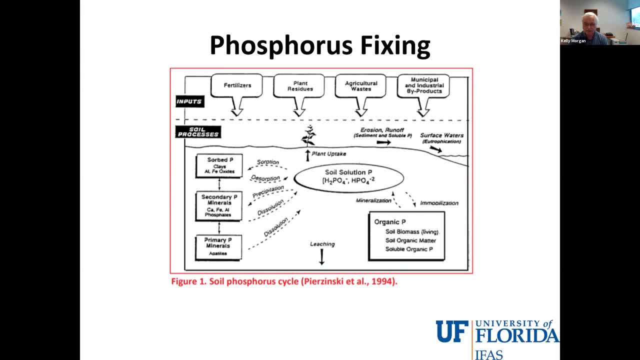 topic right now. as far as our recommendations are concerned, We're using malic-3, as our extractant for soils, to determine phosphorus amount in soils. Because it's an acid, we may be extracting more phosphorus from the soil than is available to the crop plant. 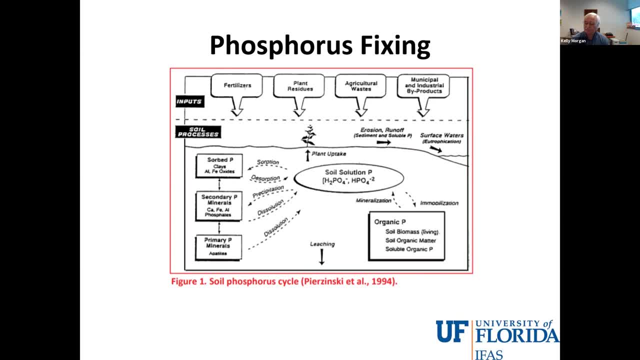 And that is illustrated in this diagram. Can you see my cursor there? This oval represents soluble P that has been applied to the soil And that is available to the crop plant. That can be taken up by the crop plant in the form of phosphorus. But if you have highly acidic or highly alkaline soils, several things can happen. 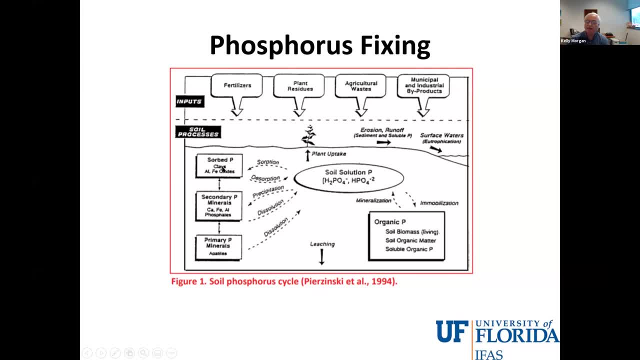 Over here you see sorption of phosphorus by clay, by clays which have iron and aluminum oxides associated with them. The phosphorus can't absorb onto the clay And over time they will desorb. the amount of phosphorus in the soil goes down. 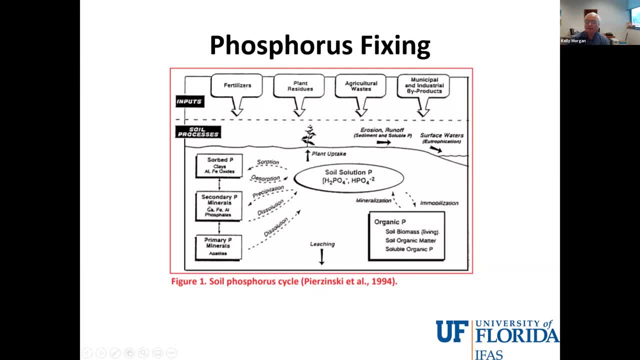 Same thing for minerals such as calcium and iron and aluminum that are free in the soil. You'll have a precipitation of phosphorus, depending on the pH of the soil, And then, as the phosphorus solution goes…phosphorus in the soil solution goes down. 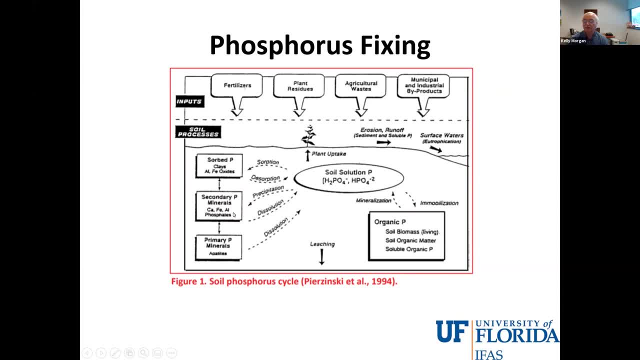 you'll have a desorption of phosphorus from those precipitates back into solution. Typically, the arrow is much stronger towards precipitation than it is for dissolution, but it depends on the soil pH and the amount of phosphorus that's in the soil. 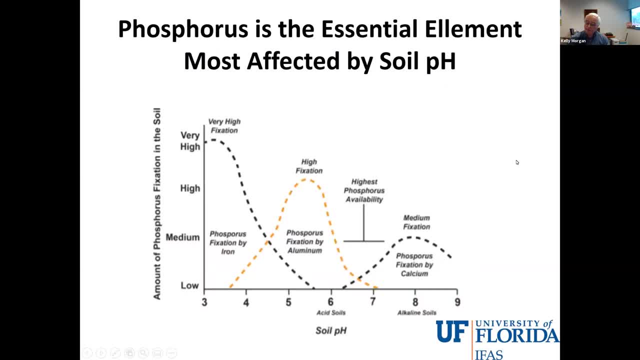 And we'll go into those in just a moment. So, looking at fixation of phosphorus in the soil, we have the pH continuum down here at the bottom, going from pH of three to nine, from acidic soils to alkaline soils And at a neutral, near neutral pH. 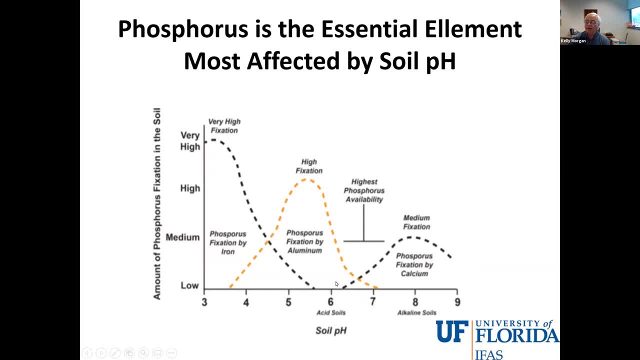 just below neutral in the six to six five range. that is the highest point at which phosphorus stays available in the soil. So if you apply phosphorus in your fertilizer to a soil that's at a pH of approximately 6.5,. 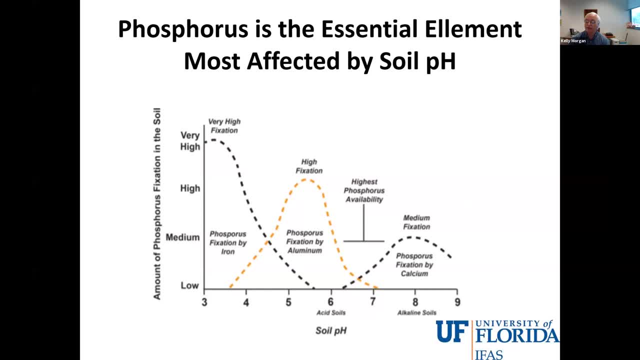 it will stay in solution much longer than if your pH is more acid or more alkaline than 6.5.. As you go through the pH in an acid soil, the yellow graph here illustrates fixation of phosphorus by aluminum. So as you go down and the highest fixation, 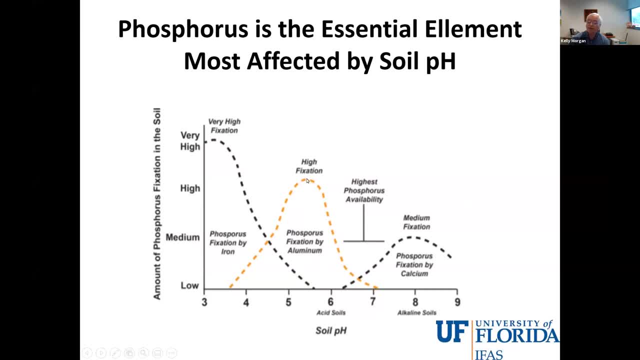 is at about 5.5, the phosphorus is being fixed by aluminum- either free aluminum in the soil or aluminum that's associated with clay. It's fixed, it's taken out of solution and it's no longer available until the amount of free phosphorus in the soil goes down. 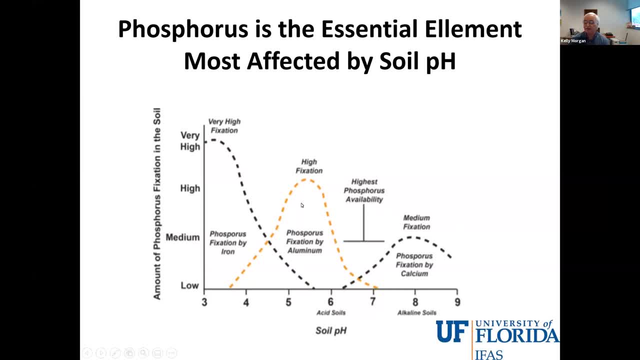 Then you can have some disassociation and phosphorus will go back down. That's the bottom line. go back into solution. If you have soil pH much lower than 5.5 and you're approaching 3 to 4 pH, which is unusual, then your fixation is primarily in the form of iron. 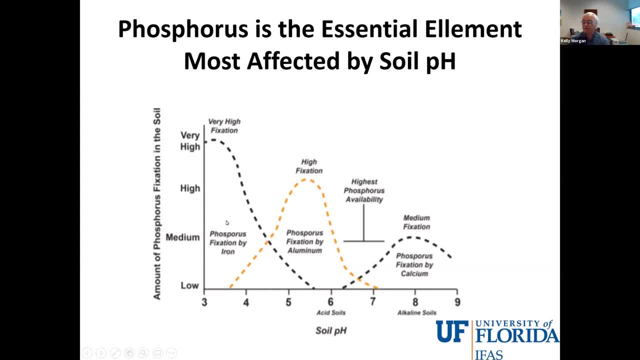 Iron very readily fixes phosphorus at these lower pHs and bringing that phosphorus back out of the precipitate and into solution is very difficult. The similar thing, but for a different reason, happens at a higher pH. So as you go from a pH of 6.5 up into 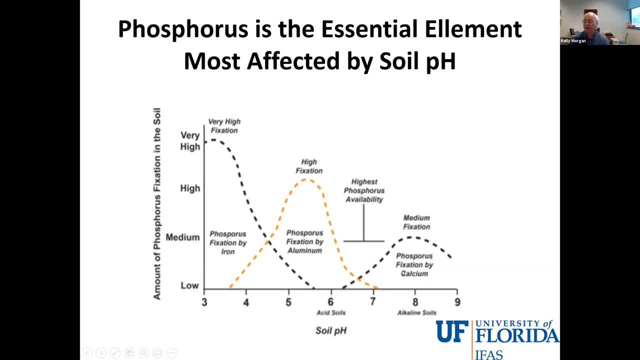 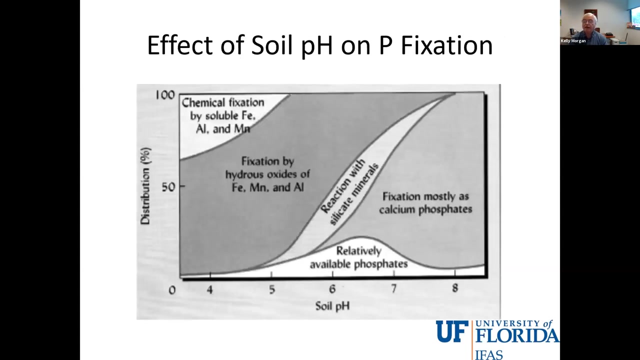 the low 7s and 8, you have fixation from calcium And as the time increases that pH becomes higher. That precipitate becomes much more solid in the soil and very difficult to go back into solution. This is just an illustration of the same type of effect You have. 6.5 is 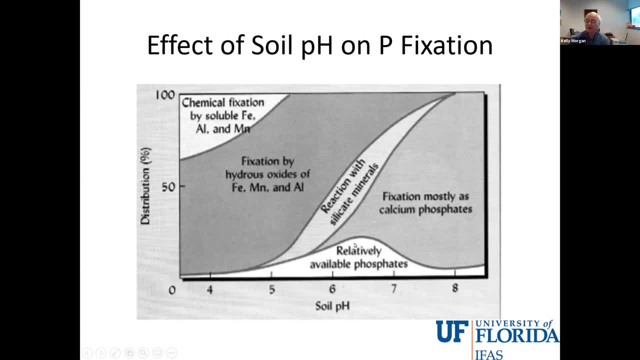 where you have readily available phosphates. Then as you go down it's fixed by 6.5.. By primarily iron and aluminum. manganese enters into that as well. And then you have chemical fixation as you go below 5.5, or 4.5,, excuse me, And there the fixation is. 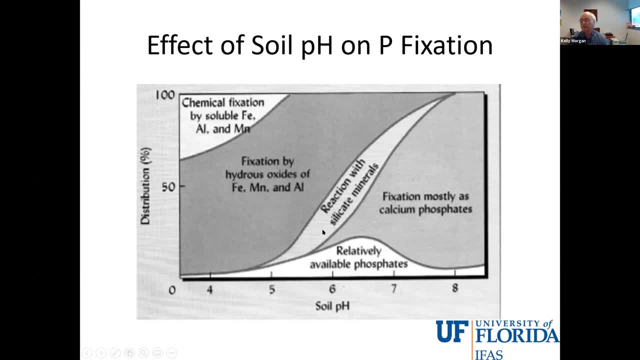 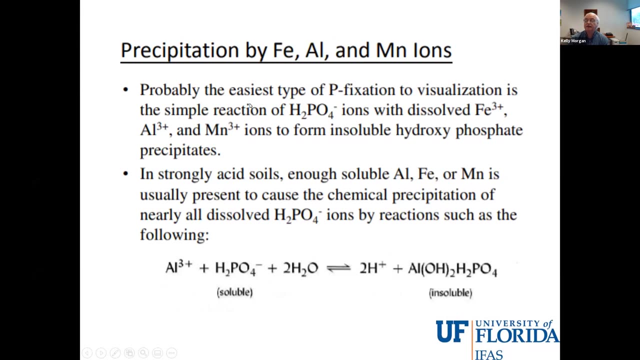 much more strong and very difficult to go back into solution. Same thing occurs with calcium, on the other end, as you go above 7.0.. And this is just illustrates that You have fixation of the H2PO4 that you would be adding. 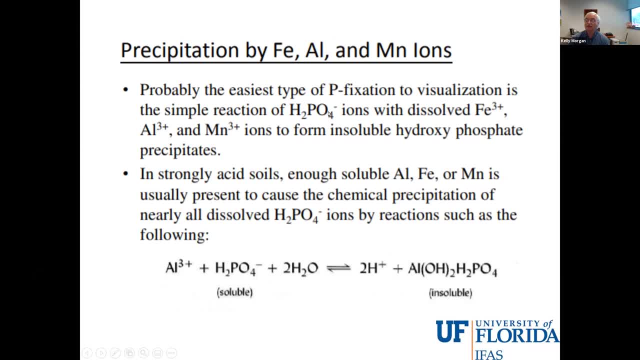 to your soil as a form of phosphorus fertilizer. If you have free aluminum, excuse me, free iron, in form of plus 3, aluminum plus 3.. Manganese plus 3. These will form precipitates with the phosphorus and will become insoluble. 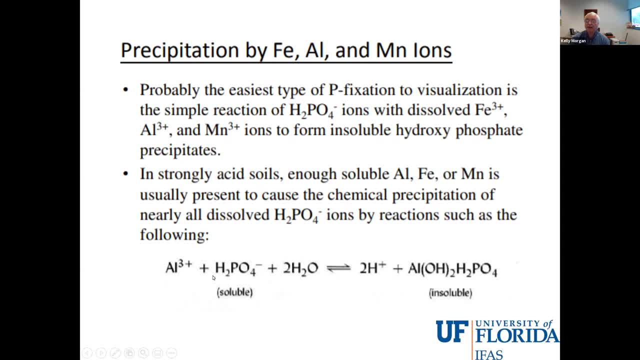 hydroxyphosphates- And you can see the chemical equations down here below- Going from a soluble phosphorus in the form of a fertilizer along with either iron or aluminum, and that reaction goes to the right And becomes insoluble. Only if you bring this soluble form down does it go back the other. 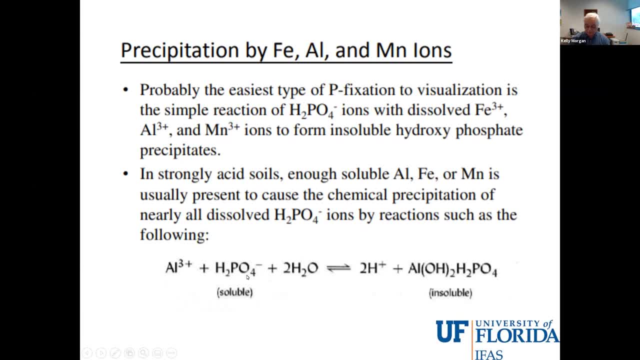 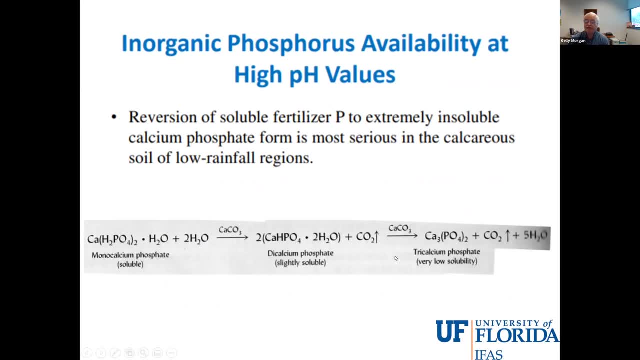 direction and become soluble again At high pH. you have a very similar reaction. But here you have to have calcium carbonate in the equation, So you would have phosphorus in your solution And then you would have in your fertilizer. It would combine with calcium. This compound is soluble, Has water. 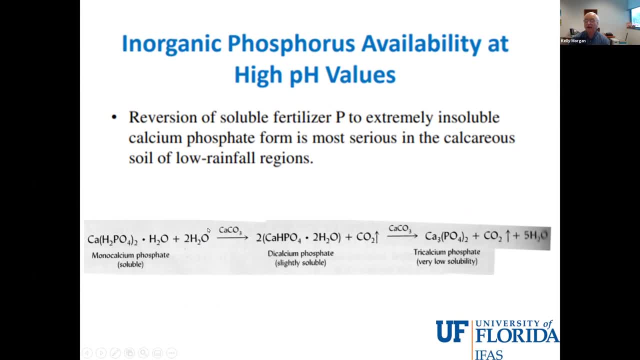 associated with it. But at higher pH, where you have calcium carbonate- such as in South Florida- associated with this, it goes to a slightly soluble form And then a very low soluble form, And that's why it's very difficult to go back. Yeah, Yeah. 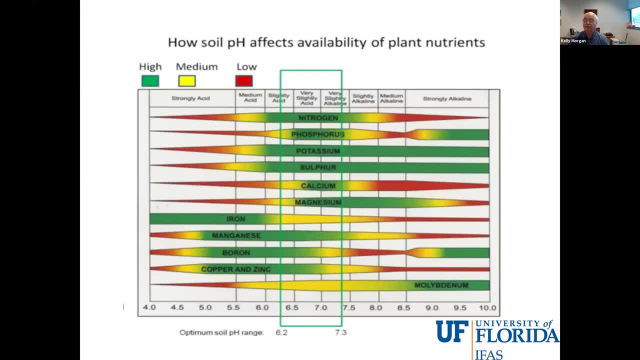 I think we can go back to the other question here. Sure, So we're just going to talk about the chlorinated hydrogen. The chlorinated hydrogen will be in the same form, but it will be in the same form throughout the entire process. 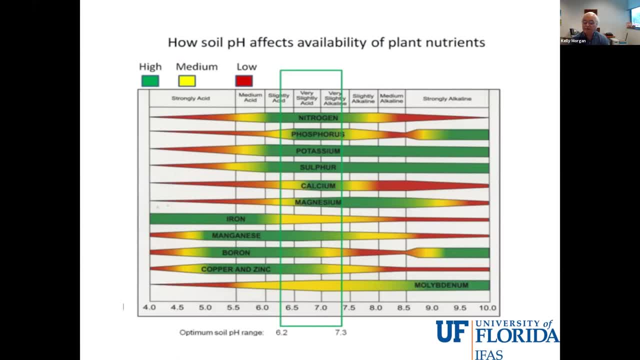 But you're going to have to go back in the other direction just by lowering pH. The other reaction that happens as far as nutrients are concerned with pH is the availability of micronutrients. We've talked about macronutrients so far: Nitrogen, phosphorus, potassium- not so much. 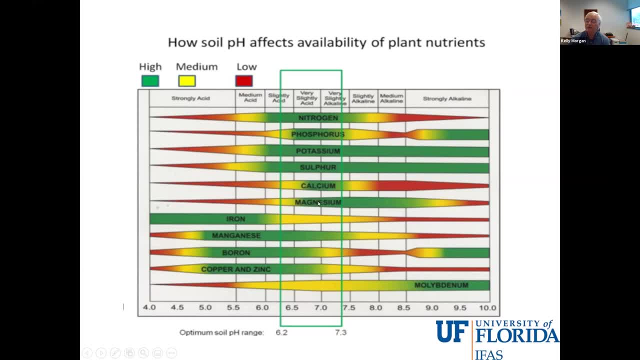 pH related Or sulfur degree magnesium, are more available in this mid-six to seven range. That's where you want to be with your soil pH. But as you look at some of the micronutrients- iron, manganese, boron- 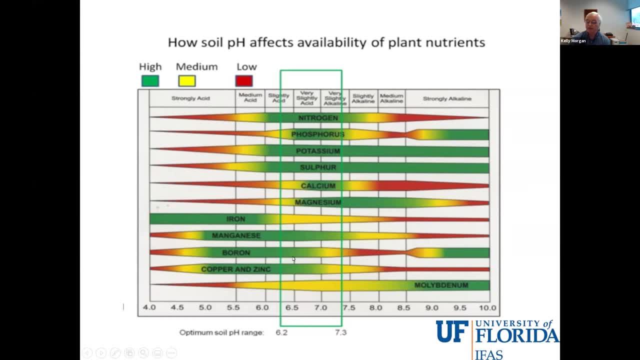 copper, molybdenum, zinc, others. if you stay in this pH range of mid-sixes to seven, you're at the tail end of their availability. They're less soluble here. They're only marginally available. Their availability is much higher at 5.5. And that's why we stretch the pH of most. 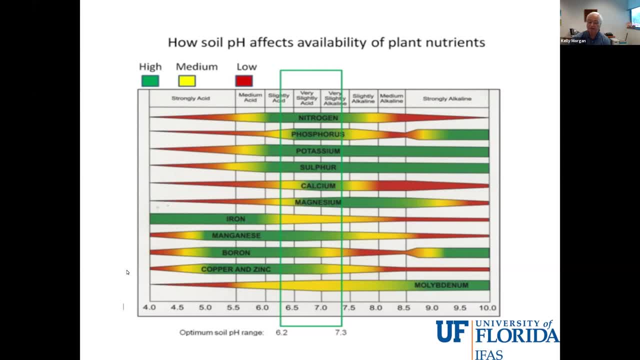 soils most crops Down to that 5.5 or six range to try to get these nutrients. So even if you're at near neutral, you need to be a little closer to 6.0 to be successful with your crops. Molybdenum is an 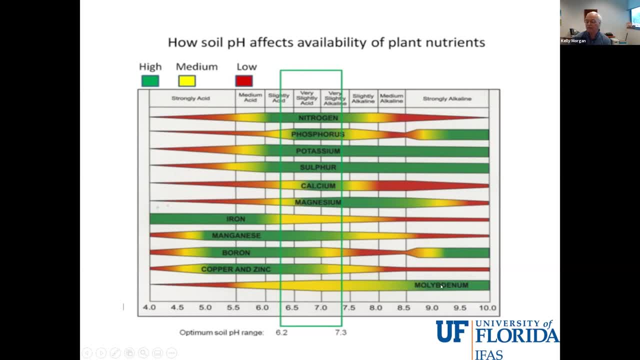 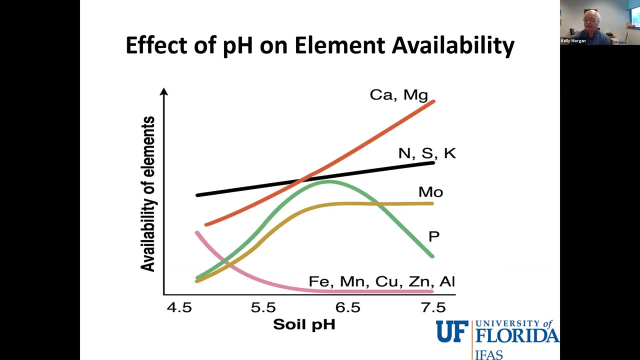 outlier. It becomes more soluble with high pH, But typically in Florida soils we don't have molybdenum deficiency issue, except for a few crops, And so this is just a graph of that same information. Looking at soil: pH, the calcium, 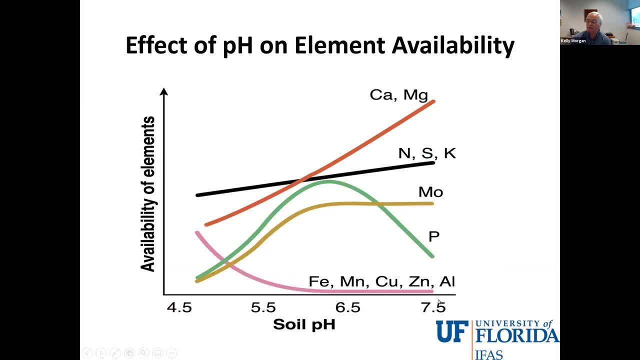 and magnesium continue to increase as you approach a pH of 7.5.. Same thing with nitrogen, sulfur and potassium: It increases with pH, but never goes low with lower pH. But these micronutrients, that's what we're looking at, And so this is just a graph of that same information. 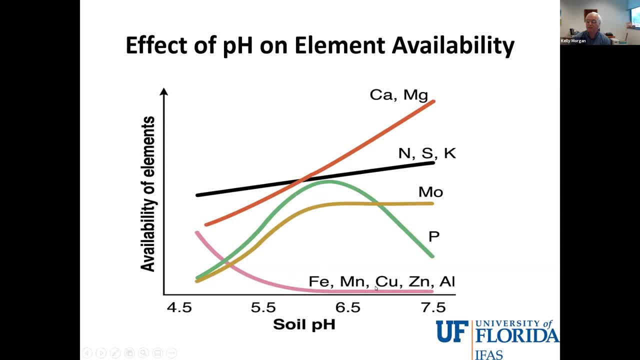 That's where one of the problems are with pH and why you need to be aware of the pH of your soil. Phosphorus, as we've illustrated, has an acceptable range somewhere in the 5.5 to 7 range, and less available at the extremes. 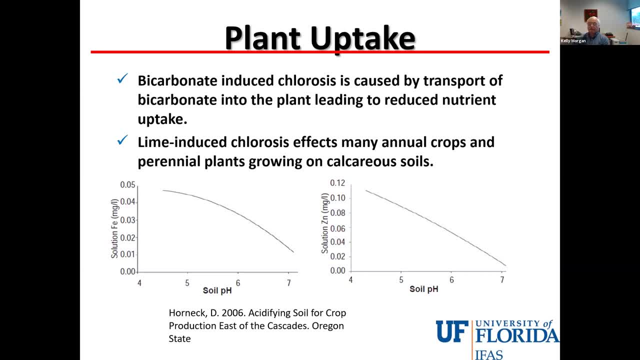 So how does this affect soil pH, Our plant uptake, How does it look as far as what we see in crops? And this is just an illustration of that. looking at soil pH, they determine the solution of iron from fertilizer in the soil, and as you go. 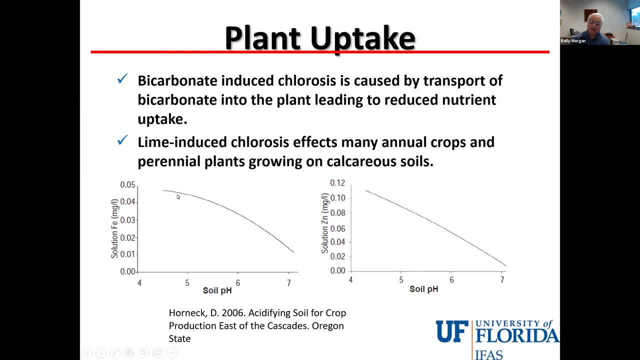 down in pH, iron becomes more available. So again, you wanna be in this mid-5 to mid-6 range, preferably for these micronutrients. Same thing with zinc: As you go down in pH you increase solubility. 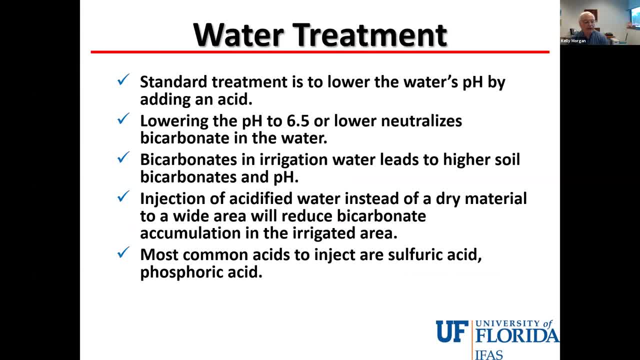 Now, one thing that we have looked at in several crops is how do we treat our soils- And this will assume that the crops are being irrigated from well water, either from drip irrigation in the rows or micro sprinkler for citrus- And we want to determine how do we treat. 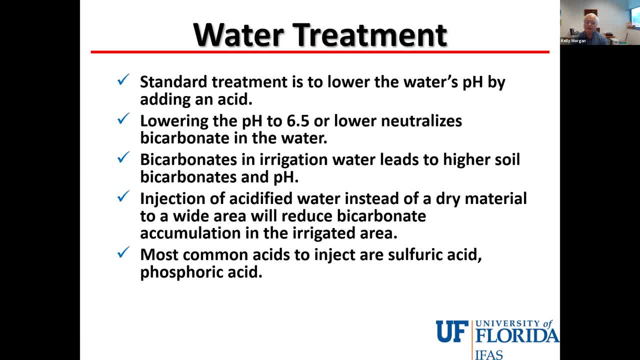 the water in order to affect pH. if we're not going to look at applications of lime or sulfur to affect those, What we have found is that, if you can acidify your soil, in most cases our water starts at a pH near neutral to approaching 8 pH. And then, if you acidify that water by addition of sulfuric acid or 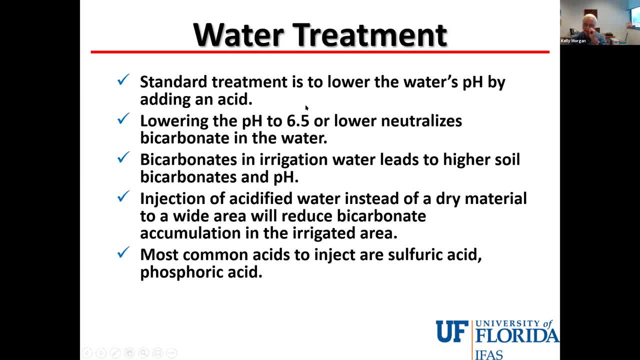 other acids. nitric acid is another one. You can lower that pH to about 6.5, and you affect the bicarbonates in the soil, in the water and in the soil. So these bicarbonates in the water are reduced, The pH is reduced. We have some citrus growers reducing their pH as low as 3.. 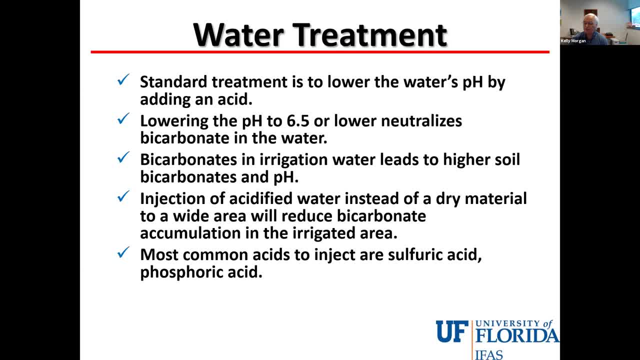 This doesn't impact the soil greatly or the tree. You would think that if you're irrigating with water at a pH of 3 or 4, that you would be causing damage to the tree, But typically our pHs in citrus groves are high enough- in the upper 6s- to. 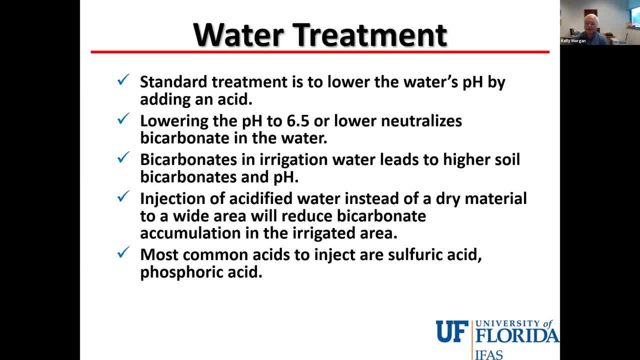 low 7 range, that that neutralizes the acidity of the water and brings that water down to that 6.5 level As it goes through the soil. So the effect, the overall effect, is to reduce bicarbonates that are already in the soil. 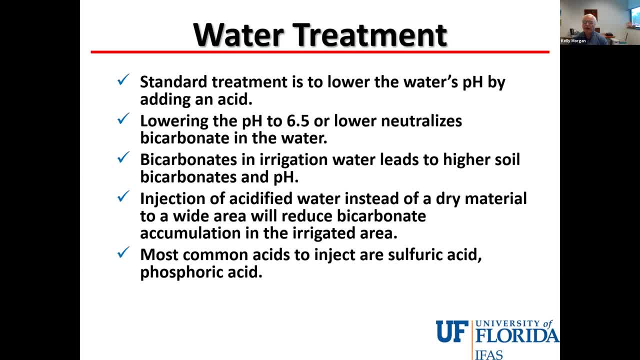 causing the soil pH to be above 7.. And over time you can reduce the bicarbonates. The bicarbonates will be reduced to CO2, and they would come off the soil as a gas. And you can reduce that pH or, excuse me, increase, reduce the pH, excuse me from. 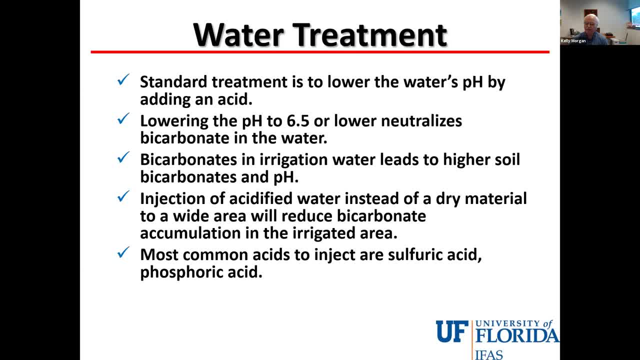 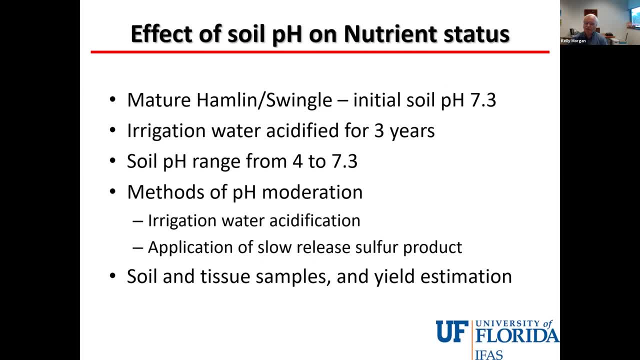 low 7s bad down to that 6.5 range that you want to be in your citrus grove. So to illustrate that we we did a study on soil pH to look at nutrient status. Here we had a Hamlin Orange with initial soil pH of 7.3.. 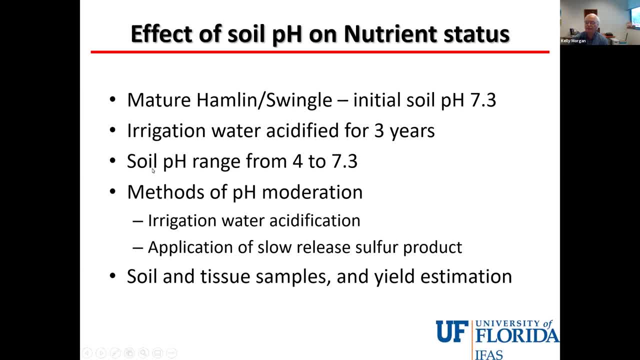 We irrigated With acidified water for 3 years. We had several Several pH of water, from three to six, and the target pH for this was to reduce the pH down to something between four and seven. We looked at the amount of the acidification of the water. we looked at bicarbonates and 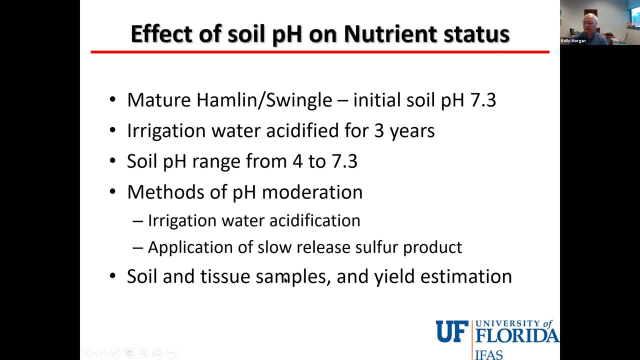 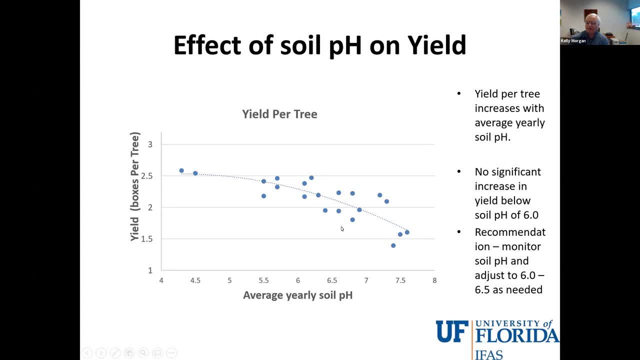 we looked at soil and tissue samples to illustrate availability of these nutrients and then, finally, their effect on yield. We did a survey of citrus groves and we found that yield of citrus is dependent on pH, strongly dependent on pH, And as you go to more neutral or above-neutral soil, you're going to see that the pH is. 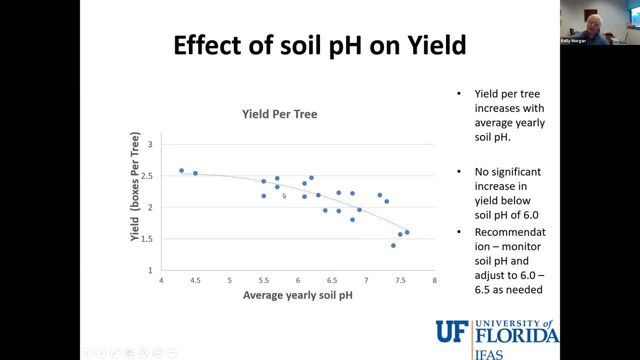 lower The soil pH is, the yield declines, and the opposite is true. As you get pH near that 5.5 level, you're pretty well maxing out your yields. So this is why we started the study to determine how we can reduce our pH- soil pH- from 7.5. 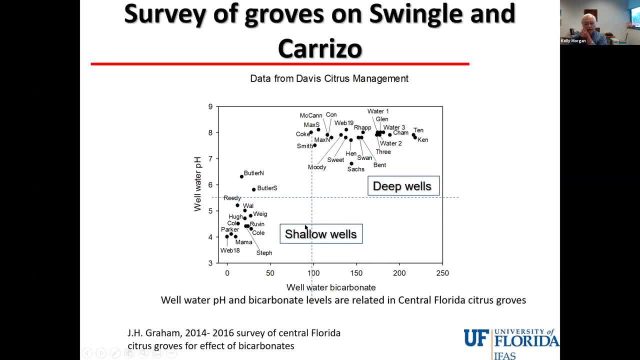 back down closer to 5.5.. We also looked at- We looked at root availability for uptake at these different pHs and we discovered that the higher pHs- pH over 6.5, were all associated with deep wells water from the. 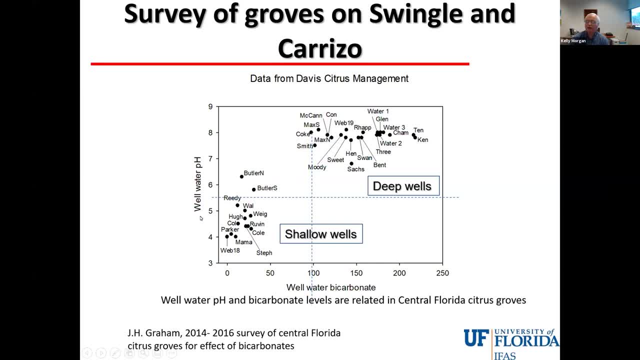 aquifer And those are the well water pHs, So they had a pH between 7 and 8 pH. If you were using shallow wells, not in the aquifer, Not in the aquifer, Not in the aquifer, Not from the aquifer- 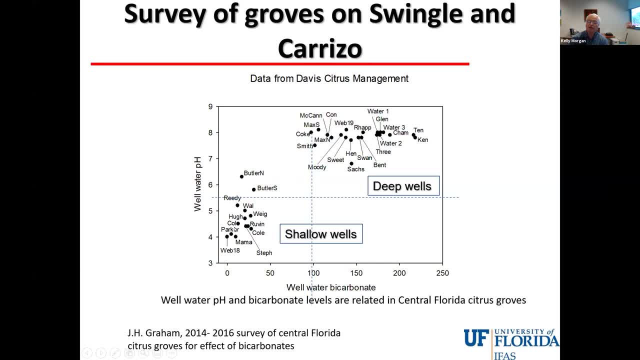 The pH water was from anywhere from 4 to 5. on the acid side, The bicarbonates. as the water becomes more acidic, there are fewer bicarbonates in the water, and the opposite is true: As the pH went up, there were more bicarbonates. 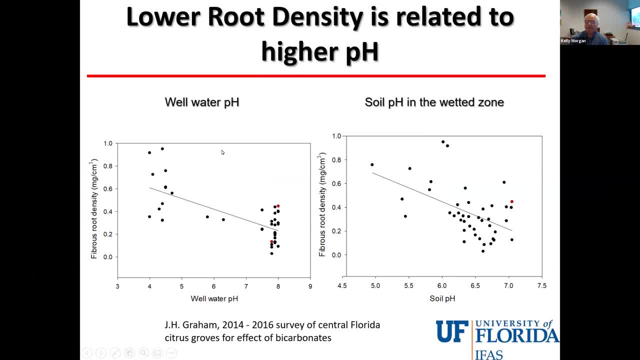 This effect was highly visible on the fibrous roots, the roots responsible for nutrient uptake. We found much lower root mass at higher pH than we did at lower pH. This was directly related to well water pH as well. So in the study we had, 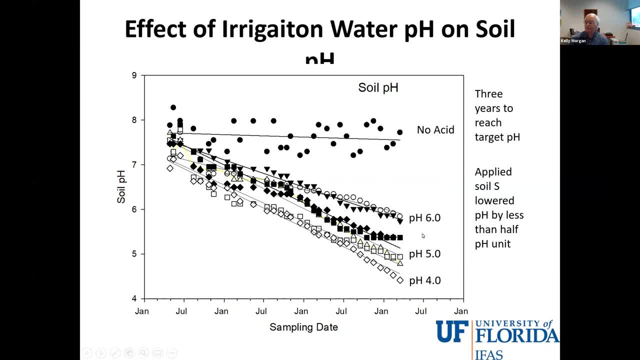 In the study. In the study we had, In the study we had, We had four different ranges where we had the pH of the water as it occurred naturally. We had a range of pH of 70 to upper sevens And then we had a target pH of 6 for the water for three years, 5 for three years and then 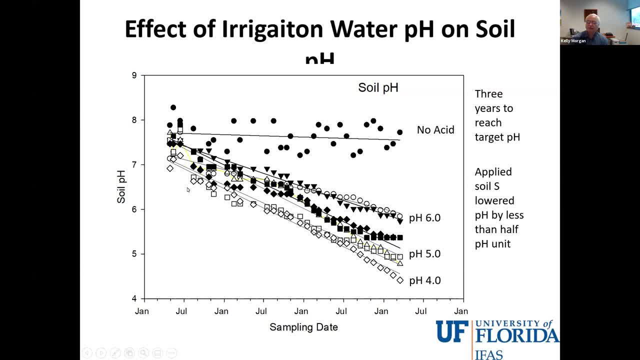 down to 4 for three years. You can see that it took a substantial time, from January of one year to June of the following year, before we got the pH down to our target levels. Somewhere down in there. Somewhere down in there. 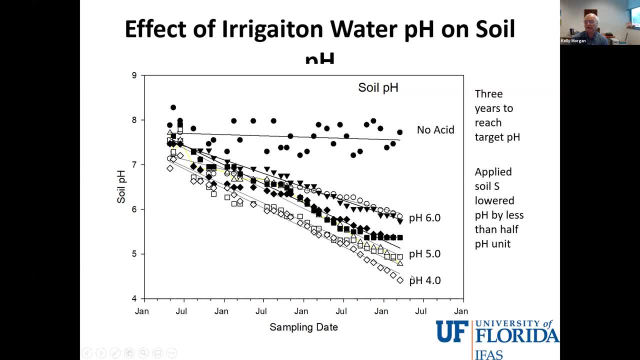 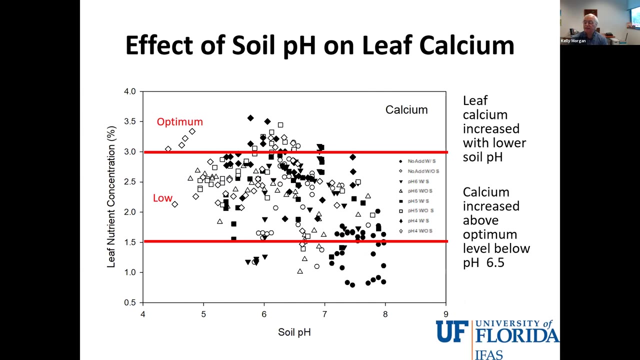 Somewhere down there the four range uh at a ph of four and about five for a ph of five. so it took much longer than we we thought but just by acidifying the water to get uh, this reaction of lowering our soil ph, but it did uh over this just two year period of time and uh, just as as an example i have. 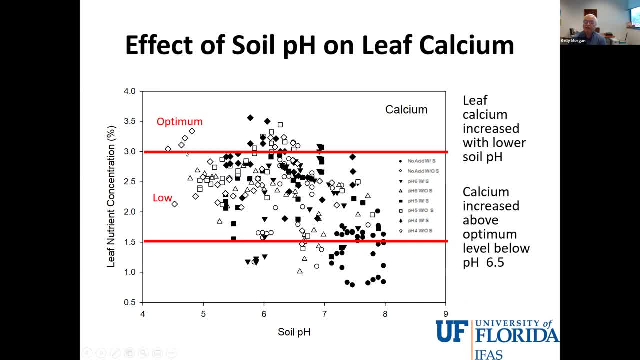 calcium content. here the red bars indicate the optimum level of leaf calcium for citrus. between these two optimum would be above this. this red bar low would be between those two bars. and you can see we only got into the optimum range at about a ph of six as we went lower in ph and higher in ph. 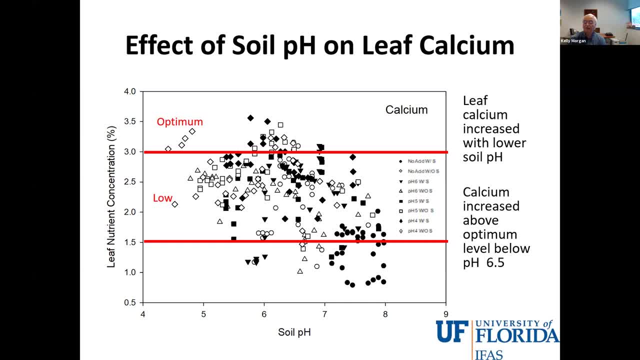 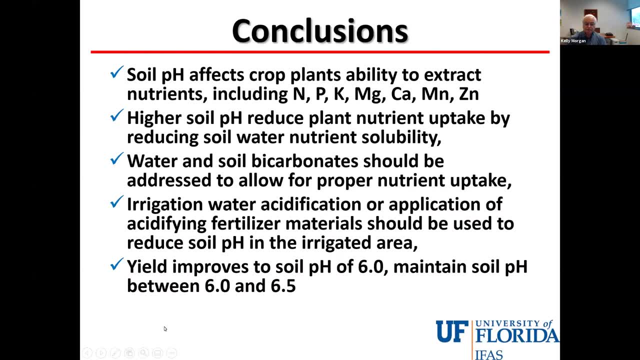 so we had uh, about a ph of six. so we had a lot of uh nutrient availability in our soil but the nutrient availability was not as great and we had difficult maintaining optimum ph in our soil. so the conclusion of this, of this talk today, was just to look at ph and the effects of ph. 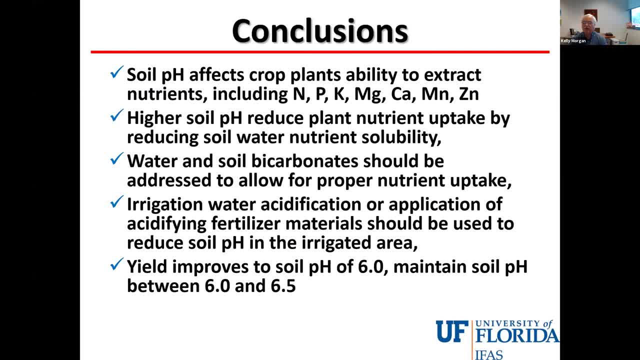 on our nutrient recommendation. we're all aware of ph. we've been telling growers for years to look at their ph, but we don't necessarily tell them why they need to be doing that. they don't necessarily look at their ph. we can give these examples now to our growers and provide that information to them. 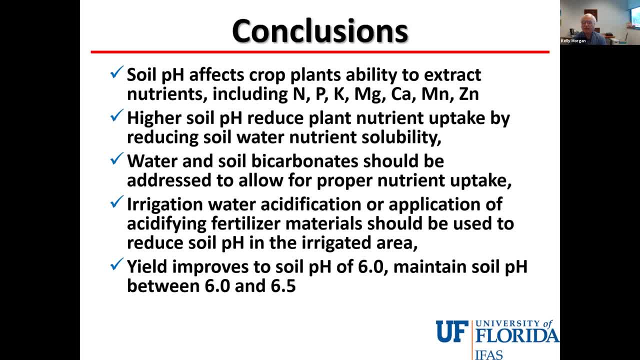 that, yes, you do need to provide a ph of a ph, soil ph in the range of 5.5 to 6.5 to maximize the availability of these nutrients, the ones you see here: nitrogen, potassium, phosphorus, magnesium, calcium, manganese and zinc primarily. others as well, iron being one of them. the higher soil ph reduces plant. 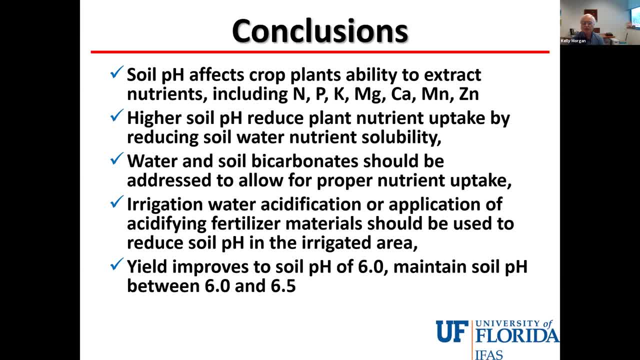 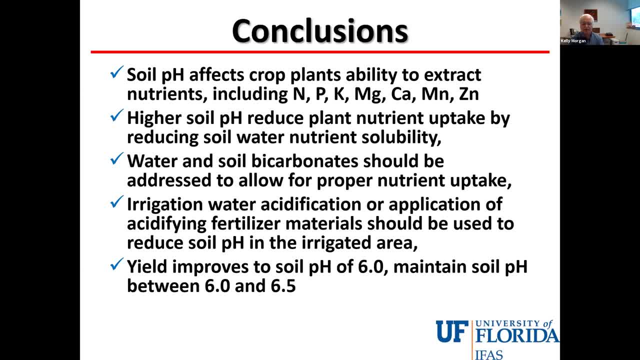 of the soil or acidification of the irrigation water. you can drive off those bicarbonates and produce a lower soil ph and then yields increase, particularly in citrus, as you improve soil ph and maintain that between 6 and 6.5. so i'll be glad to answer any questions you may. 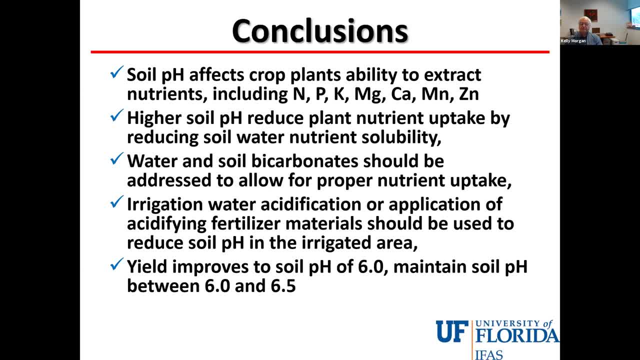 have. thank you, dr morgan. we have one uh comment in the chat box past recording. okay, so that's from emily. um, we do not have any specific question from the audience. um, i would request an audience. so if you have any question, please type your question in the chat box and i will. 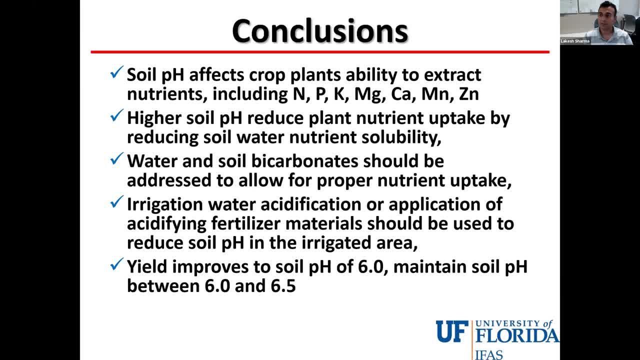 ask that question to dr morgan for your answer. um, um, so i think, uh, people might be typing. so, dr morgan, i have a question about it. um so, when the ph changes, the phosphorus availability changes and, uh, there is a past, i mean on the on. 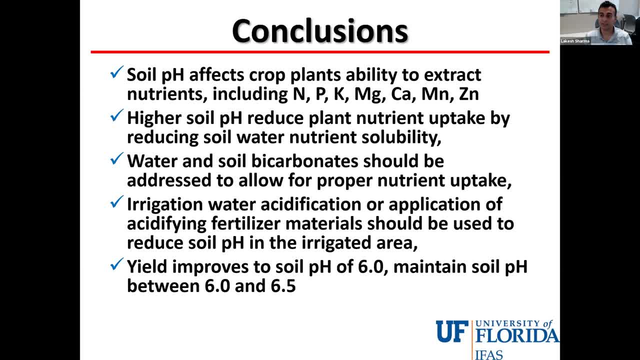 the alkaline. alkaline soils it's a calcium, but on the acidic soils it's mostly aluminum and iron. when, when it is fixed- uh, does that are? phosphorus is unavailable for the, you know forever, or it could be it could get back. so is it a reversible or irreversible kind of a process? but both reactions are reversible. 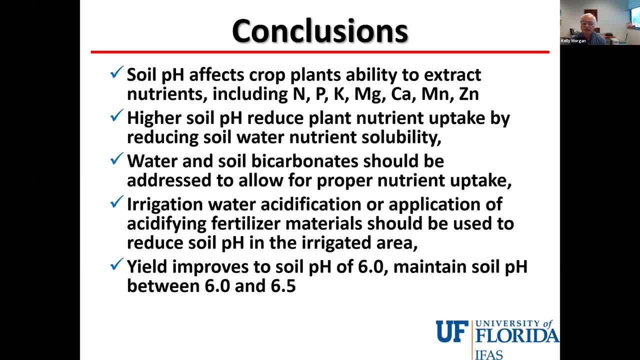 it's a solubility uh. it's a solubility uh problem at that point as, as you go higher in ph, the calcium makes phosphorus less soluble. it precipitates, precipitates out with that. precipitate can become soluble again if the pH goes down or the phosphorus concentration in solution goes down. 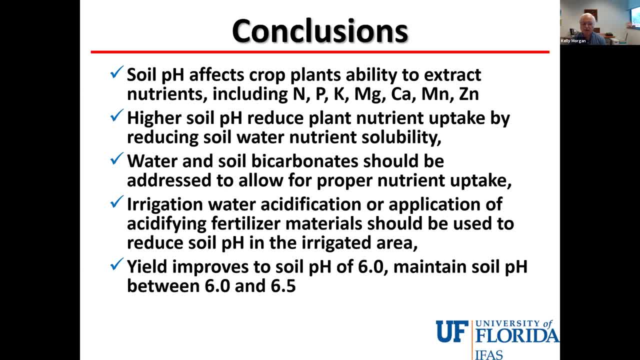 It can become soluble. Same thing at low pH: If you have free aluminum and iron, it precipitates out, but then can reverse as you increase your pH. Thank you. Thank you for this answer. All right, we have a question here: How common is it for the growers to manage irrigation water pH to achieve these optimum ranges? 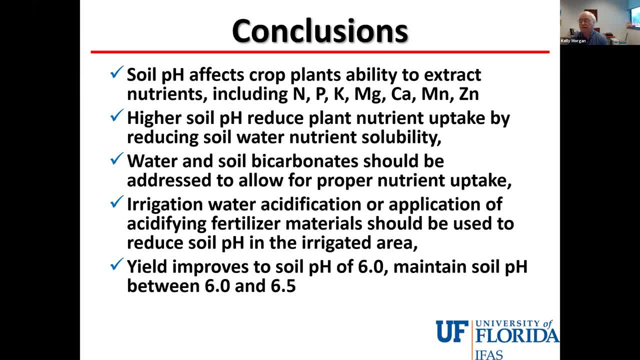 In South Florida it's very common We've talked to. you know we've been recommending water acidification for citrus and vegetable production for a number of years now And almost all growers acidify their water and most vegetable growers do now. 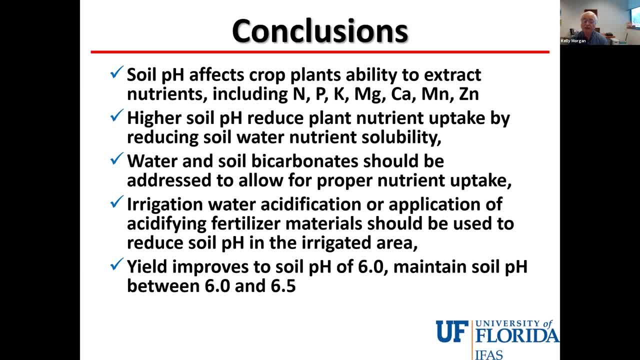 They didn't begin to begin with. So this is a relatively new change, but one that they have done just in the past, say five years, Thank you. Next question is: what is the cost of irrigation water acidification? It varies on the starting point: how alkaline your water is. 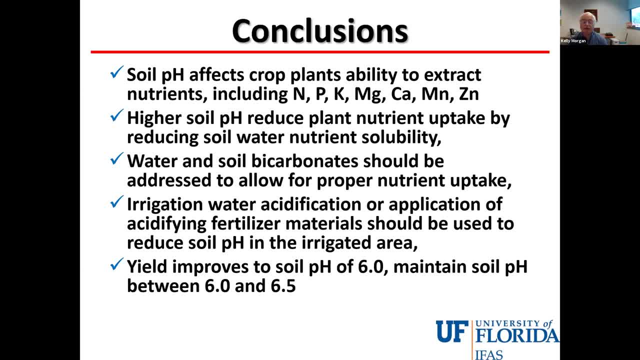 But it can vary. It can vary from a few hundred dollars a year in citrus to somewhere approaching $1,200 to $1,300 per acre. So it can be quite expensive if you start out with very high soil pH and very high water pH. 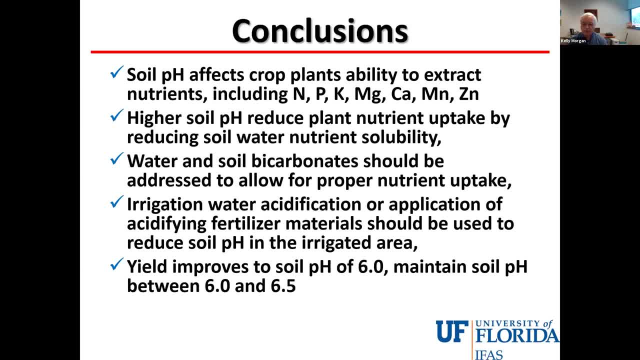 So most growers typically shoot for a reduction in pH down to about six. Because what we found is, if you maintain good soil water content at a pH of six, it doesn't matter so much what the pH of your soil is, Because the nutrient availability is then tied into the pH of the soil solution or the water that's there. 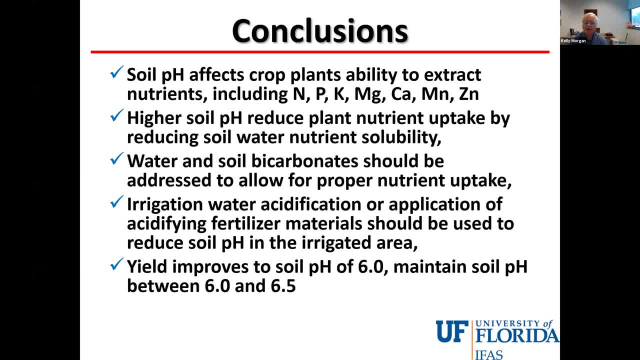 If you allow the soil to dry out between irrigations, then your pH could go up, Your pH of the solution would go back up and your nutrients would become less available. Thank you, We have a question on economics. So what is the economics of reducing bicarbonates in water and soil? 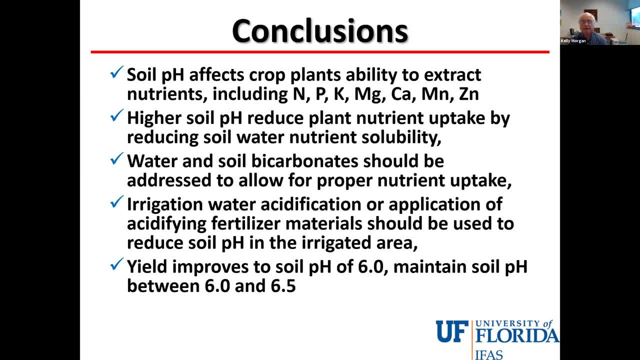 Well, what we have found is, as you reduce the bicarbonates in the soil- and this can take many years- the soil pH reduces, goes down. So if you start off with a pH in, say, mid sevens and acidify your irrigation or directly acidify your soil for a number of years, 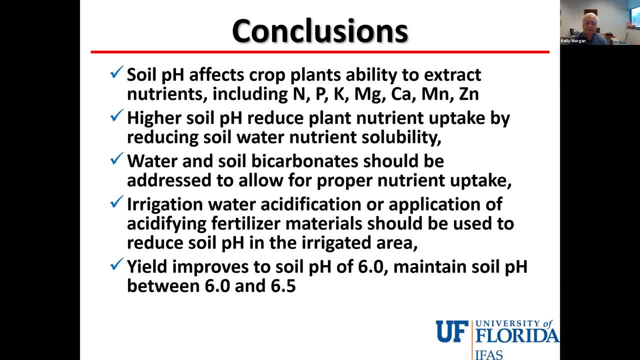 you can be in that pH range of six to 6.5, on a fairly steady state at that point, So you can reduce the acidification of your water And the cost of acidification would go down dramatically. Thank you. So there's a question on the quick test. 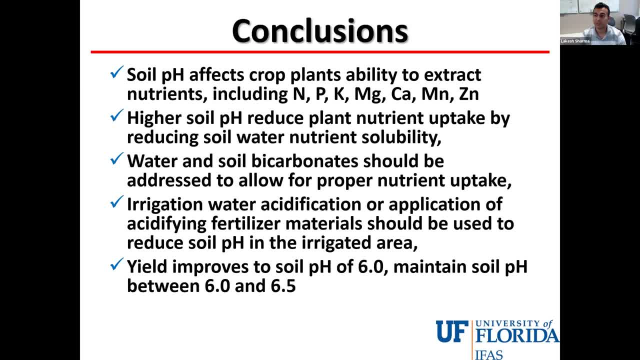 How do you recommend the grower monitor their soil and water pH Via lab or is there any quick, reliable test to determine it? There are. We have recommended to growers that they measure the pH with a pH meter. You can buy handheld pH meters that are reasonably reliable, not one you would want in your lab. 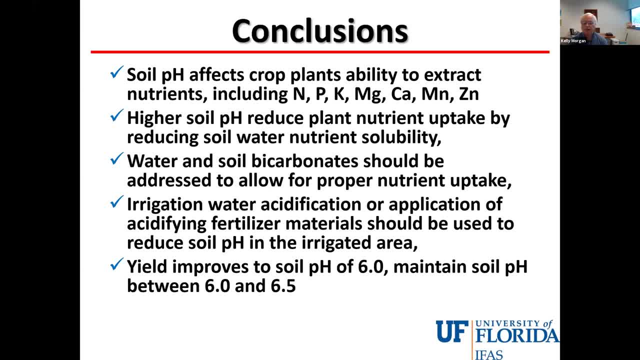 but one that will give you a fairly accurate measurement of, say, plus or minus, a tenth or two of pH unit, And that would cost maybe $100 or $200.. And so we have growers that routinely collect water out of their emitters- their irrigation emitters- after it's been acidified, and take the pH of their water. 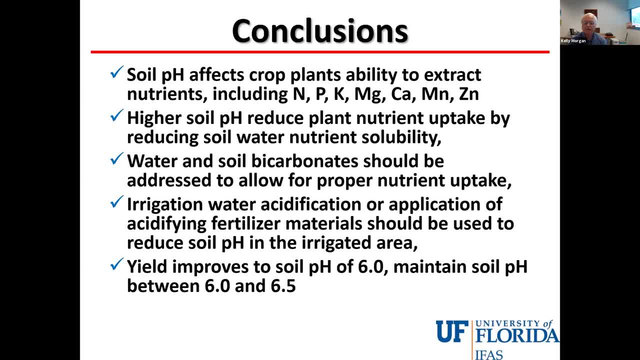 And they can adjust the acidification injection to their water to get the point that they want. Okay, there's a follow up question, Kelly, on the cost of irrigation water acidification. So we have a question. that's a follow up question. 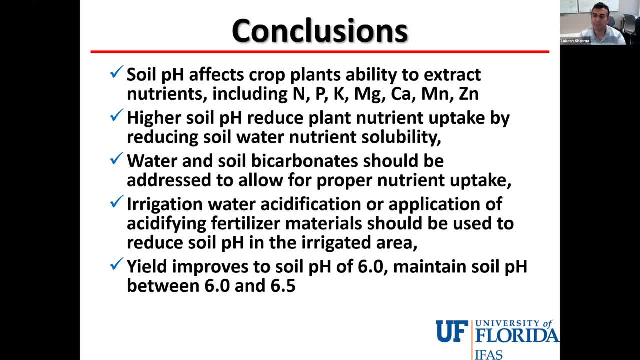 What's the problem being noted by the growers using this method, which means acidification of irrigation water? I'm sorry say that again. So what are the problems being faced by the growers using the method of acidification of irrigation water? There are a couple substantial problems. 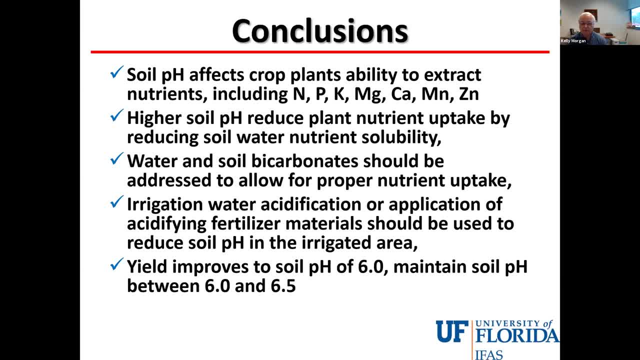 One is the cost of the injection. equipment can be very expensive Because you're injecting an acid solution, So you're talking about stainless steel pumps, stainless steel injection points, So that could be expensive. The other is the solution you're injecting. If you're injecting sulfuric acid or phosphoric acid, they are quite corrosive. 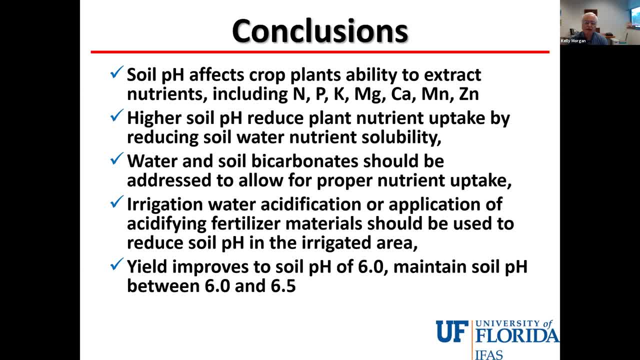 That's why you have to have stainless steel pumps, But they can be dangerous to the person applying them. They can be dangerous to the acid as well. There are products that is a combination of urea and sulfuric acid. One product name is called infuric. 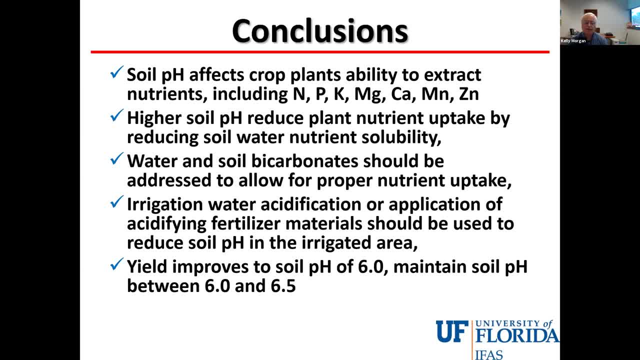 And by adding the urea. it's still highly acidic but it's safer. It doesn't cause the damage to the skin that some of the acids do And most growers are using that. Plus, it's a source of nitrogen to the crop. 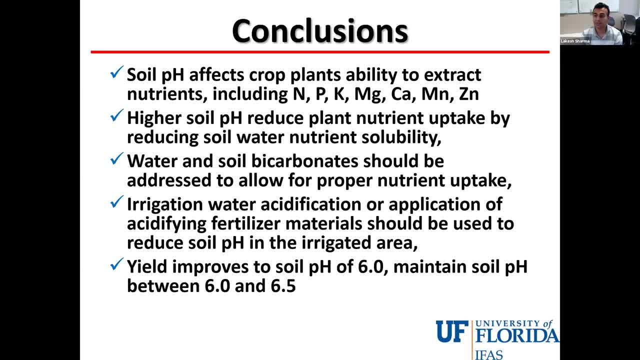 Great Thank you. Does IFRS have any document that gives information about adding acid to irrigation water? Yes, there's a couple good EDIS documents on acidification. All right, Several years ago, horizontal wells were installed for irrigation. Could they be an alternative to avoid high bicarbonate aquifer sources? 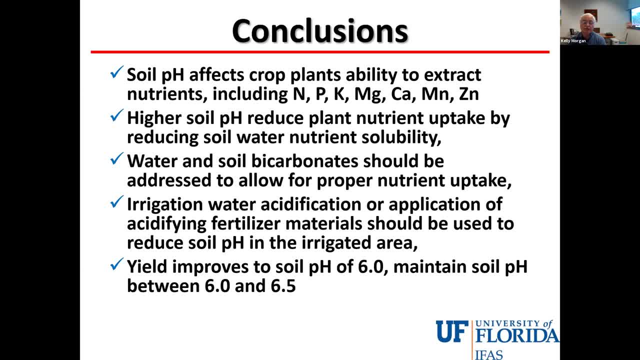 We've not tested those, But yes, I think they would be. They would not be getting water directly from the aquifer And in some of the situations- the farm here on the research site being one of them, we use shallow wells less than 100 feet. 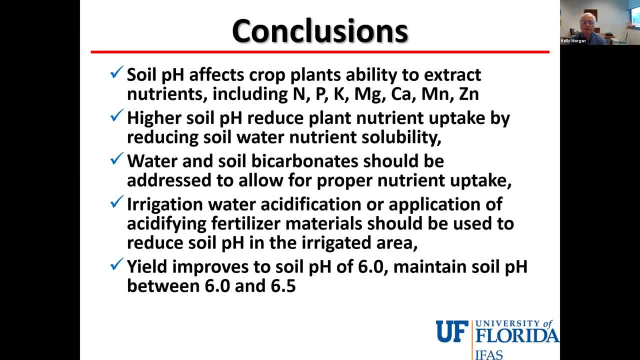 And we don't have the alkaline issue, the bicarbonate issue. if you have relatively shallow wells, You get a reduced flow, of course, because you can't take that much water from the wells at a lower depth. But yeah, if you can take water from a horizontal well, I think that would reduce your need for acidification. 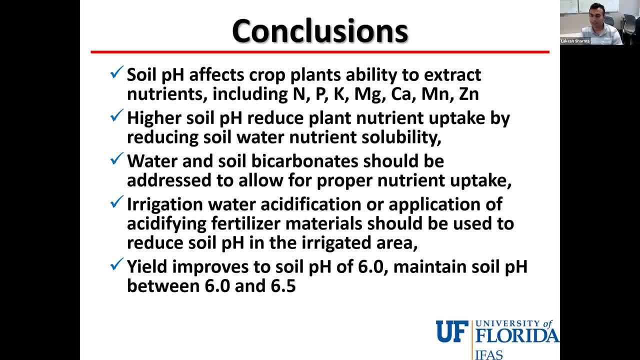 Thank you. Okay, Last question: Does this acidification help keep the emitters clean? It can. yes, That is one side effect of it. What typically happens- the reason you get a lot of clogging- is that you'll get these bicarbonates. 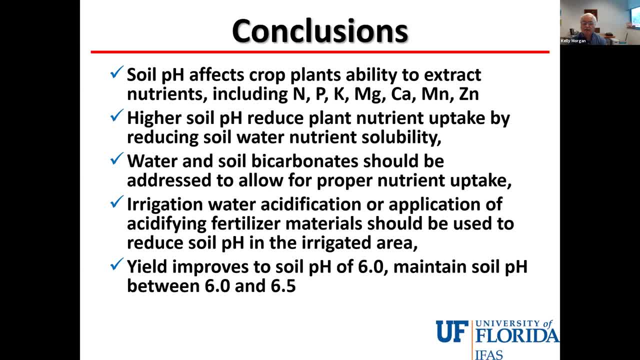 These bicarbonates coming in the water And then they precipitate out at the emitter, causing a hardening or hard deposit at the emitter. That's very difficult to get rid of, But the acidification will cause those precipitations not to form and can keep your emitters cleaner. 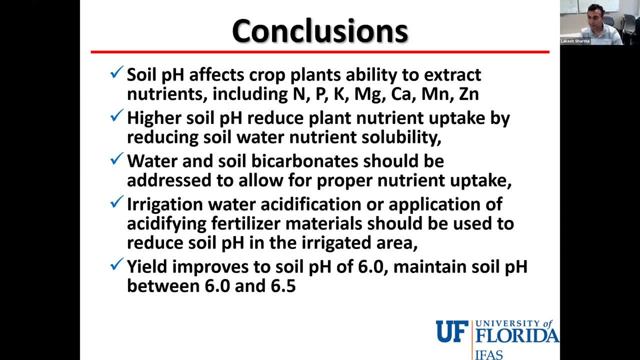 Okay, I think Dr Dukes actually shared Edith's publication in the chat box on clogging, irrigation or fertigation. Okay, We can take one more question. How does pH change in well water seasonally or throughout the year? 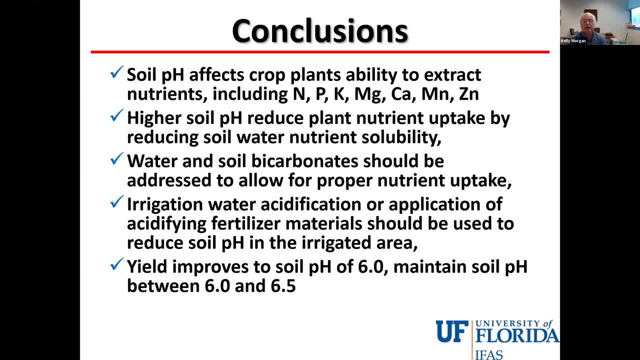 It does change, seasonally rather, And that's why we encourage the growers to monitor the pH of their water. If the pH goes down, the bicarbonate level goes down, They can reduce the amount of acid that they inject, And the opposite is true. 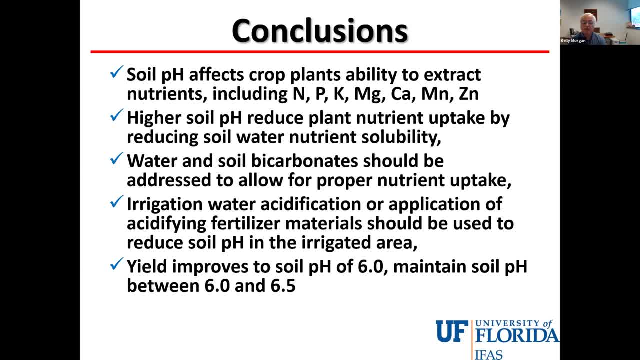 If it goes up for some reason, they need to apply more. So they should have a target pH in mind and try to maintain that target pH. The reason it would go up and down is just because of rainfall. Typically we see lower acidity and bicarbonates in the rainy season than we do in the dry season. 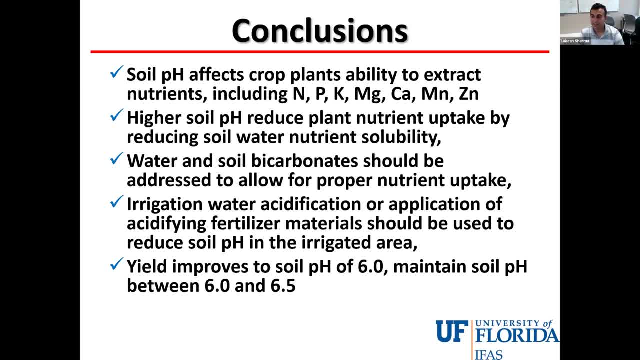 Okay, We are still getting some questions. We have three more minutes for you. Dr Morgan, I'm thankful to you for answering all these questions And I'm glad that our audience is asking all these questions. How effective is ammonium thiosulfate in mitigating high pH problems? 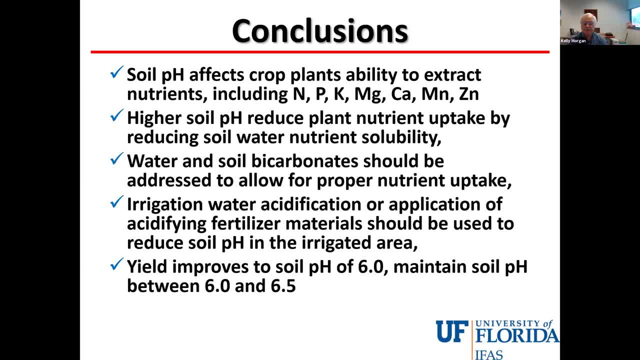 Well, it depends on your starting point and your crop. It can be very effective. We have tested that product And it can bring the pH down half a unit or so, depending on how much you're putting out and what your starting point is. 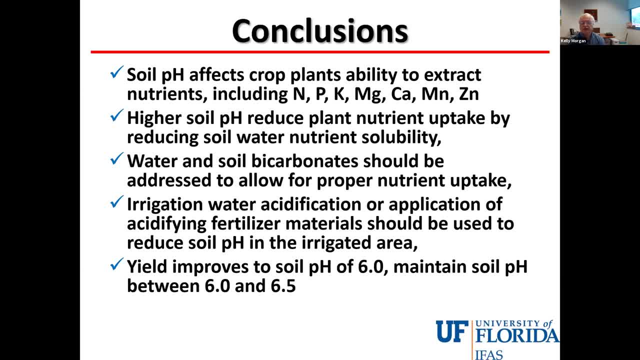 But it can reduce your soil pH. Dr Morgan, I have a follow-up question. Is it ammonium sulfate? It's been in the literature that it's four times more acidic than any other nitrogen source. Would that be more? Would that be more helpful, or people are already using it? 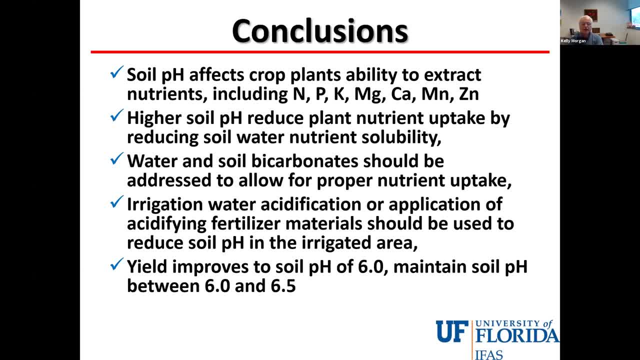 To acidify the soil Soils. Yep, Yeah, It's one that is recommended for high pH soils. If you want to use your fertilizer as an acidifying agent, that's a very good one. Thank you, All right, We have another speaker lined up. 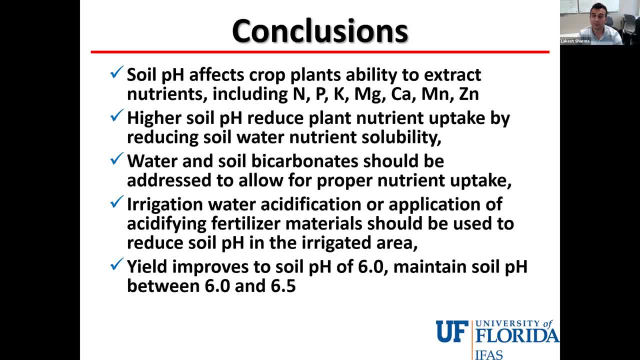 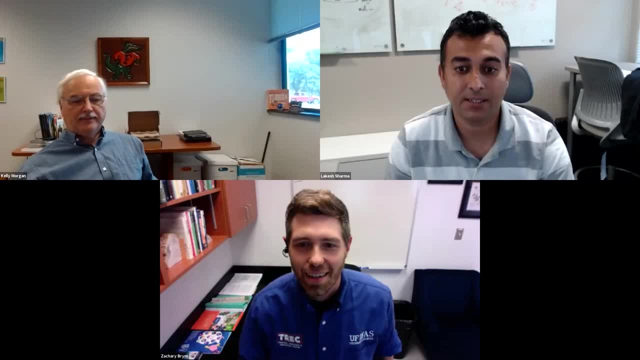 We still have a couple of questions for you. Dr Morgan, If you hang until end of the session, we would ask you these questions. And now, if you stop sharing, then I will invite Zach to share the screen. Dr Brim is-. 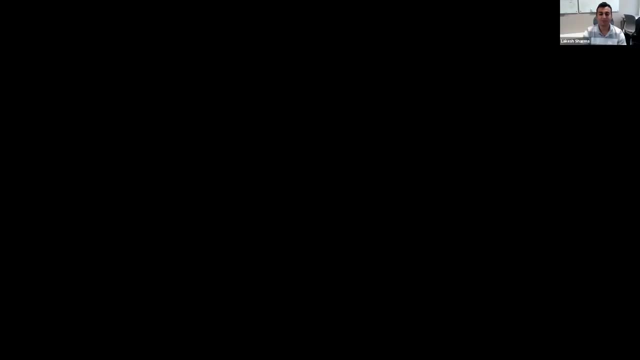 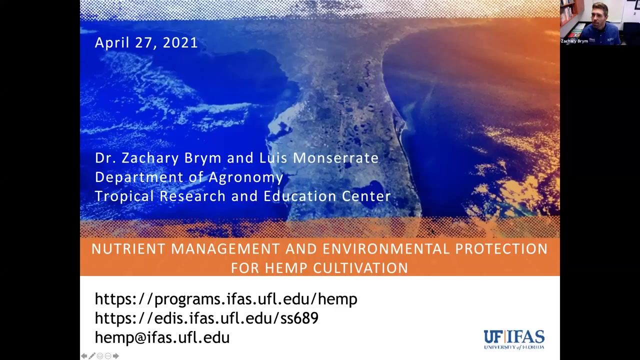 Good afternoon everybody. All right, Here we go. All right, Thank you. All right, All right, Okay, All right, All right, Thank you. That should do it Living the dream. All right, Hey everybody. 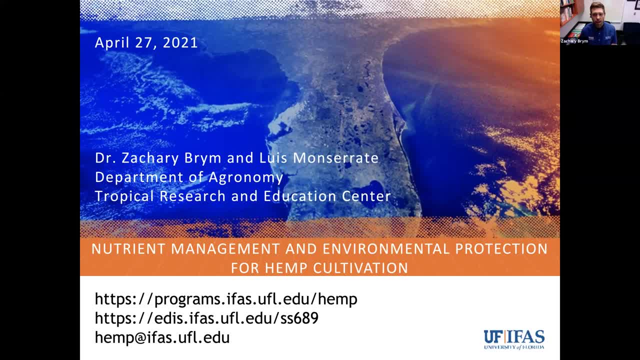 So I was asked to come and present an update on the information for industrial hemp And I will come back on several of these resources later on. just to give you a sense of some of the information that's available on our website and this fertilizer guidelines document. 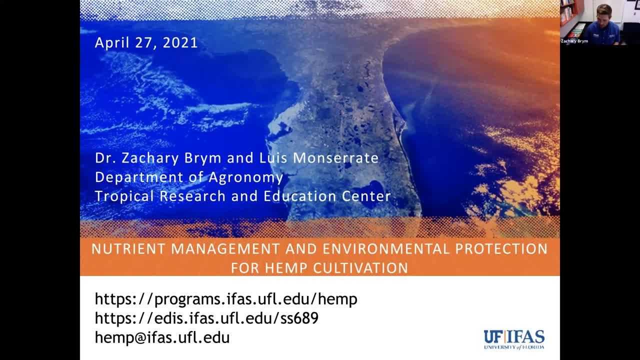 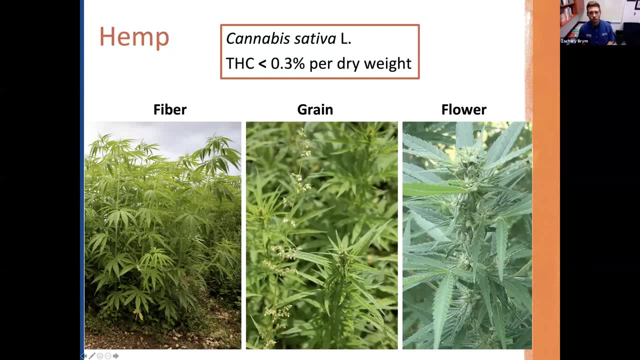 we posted to EDIS last year as well. Let's see. So this is as good of a place to start as anywhere. hemp, as it's defined, is botanically cannabis sativa, So the same plant as marijuana. However, the legal distinction is one of chemistry. 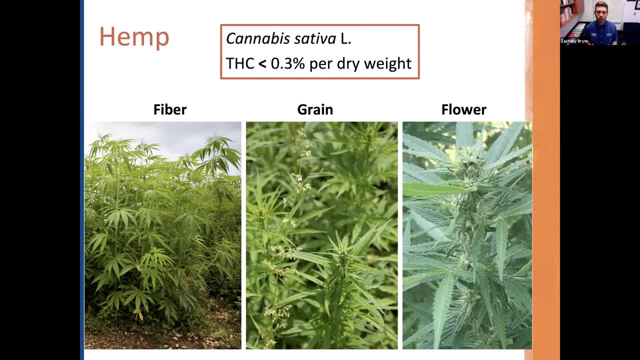 So THC, Delta-9 tetrahydrocannabinol, must be at a concentration that does not exceed 0.3% to be hemp. So below the 0.3, you have hemp, above the 0.3, you have marijuana. 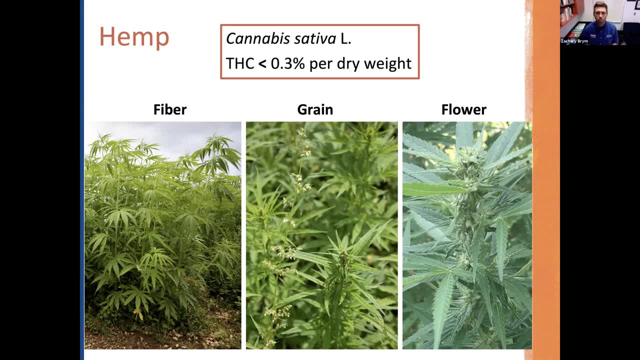 And so one of the one of these things that hemp farmers are going to need to be concerned about and mindful of is ensuring that their plants do not exceed this threshold. I don't get into that much today, but certainly by way of a definition. 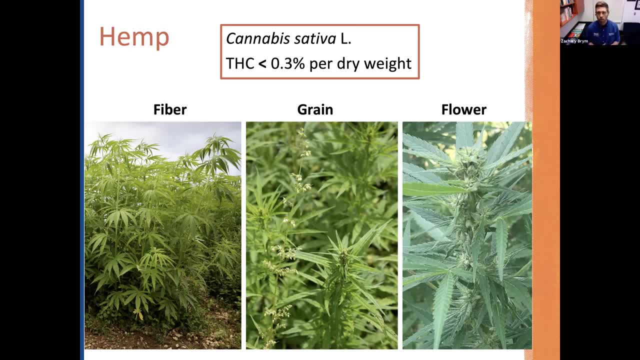 and the plants that we're talking about here. it's really important. Another distinction to make is the multiple cropping systems and products that can be a result of hemp cultivation, So I break them down into these three. Each one really is a separate cropping system. 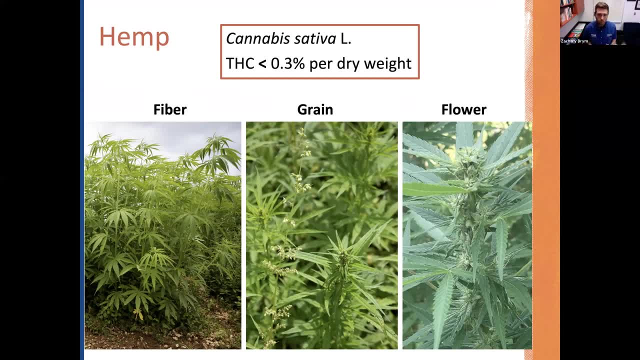 based on seasonal timing, fertilizer management, harvest and the like. So fiber is the first one here in the picture on the left. You are putting these at exceedingly high densities. Some folks will tell you three quarters to a full million plants per acre that you're working to achieve. 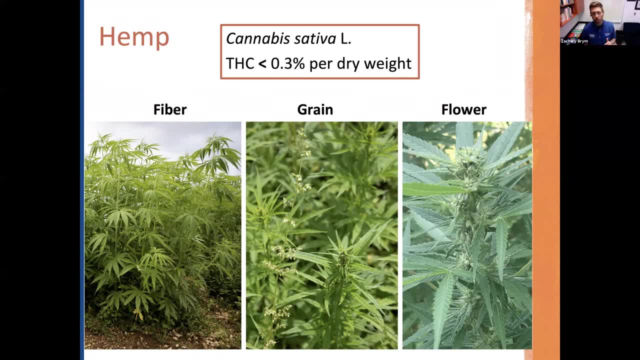 These fiber plants are harvested just before flowering to collect the stems. The second here in the middle is grain production. So one of the interesting botanical features of the hemp plant is that is dioecious. There are male and female plants in a population. 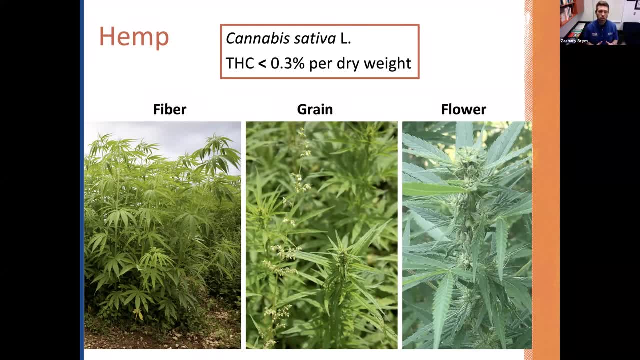 And so, in order to get grain, you want both of those. in the field, You allow the males and the females to produce flowers. The pollen, which is wind dispersed, moves from the males Into the females and produces the seed on the females. 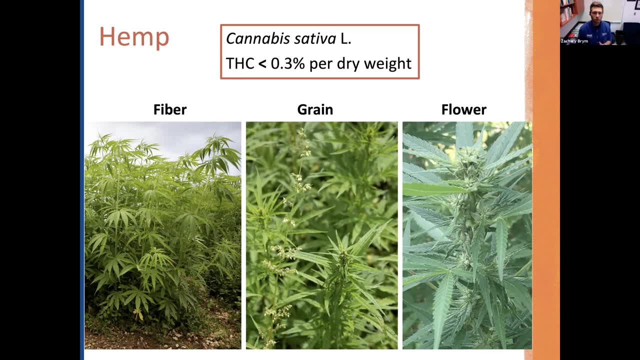 That's harvested as the seeds are hardening. The third cropping system which generally most folks are interested in, modern cultivation, is for flower production. These varieties are high in cannabinoids, So cannabinoids that are not THC, So THC less than 0.3%, but higher in O2.. 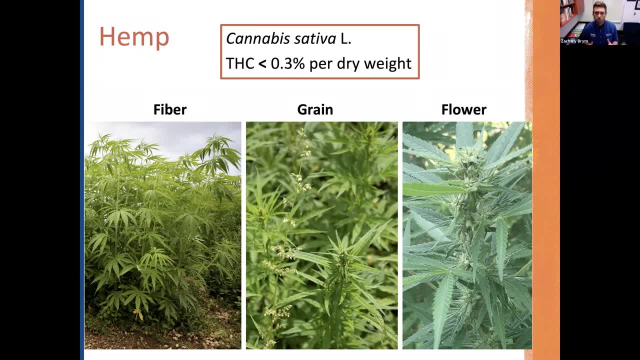 Other cannabinoids, such as cannabidiol, which is CBC, or cannabigerol, which is CBG. Now, an interesting component of this cropping system is that the trichomes associated with the flowers and the leaves in those inflorescence stems 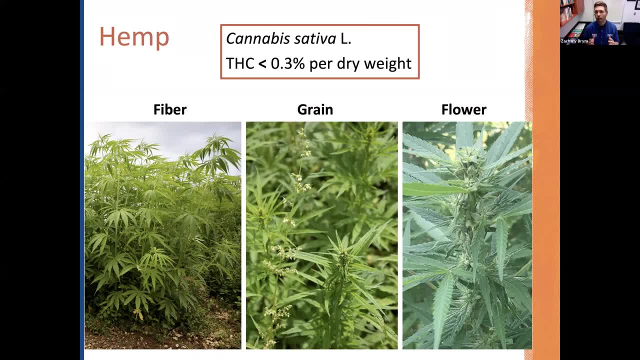 produce the highest concentrations of these cannabinoids. In order to continue producing cannabinoids, you want to avoid pollination, And so the flowers are un-pollinated, the grain systems are pollinated, And so it sort of poses an interesting challenge for the hemp industry, with some neighbors looking 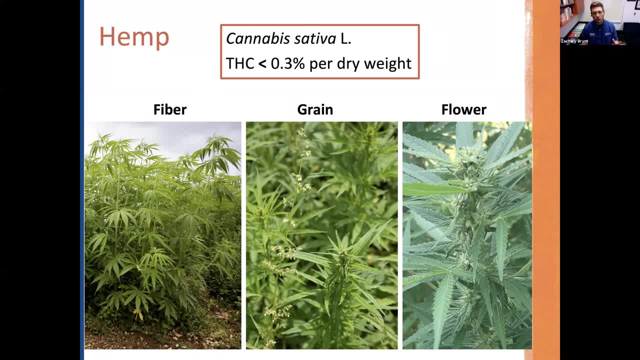 to put pollen in the air and others looking to avoid it. The cannabinoids are also tend to be transplanted- Plants that are clonally propagated and transplanted in the field- and much smaller densities. If they're transplants, you're going to be putting them out. 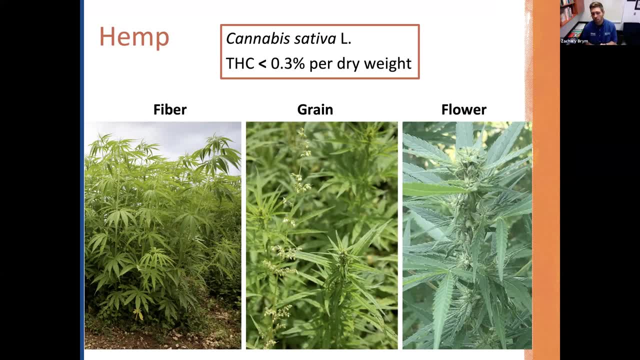 somewhere between 1,200 and 2,500 plants to the acre. There are some cannabinoid varieties from seed and those maybe make a density of 20 to 20,000 plants an acre. So what's the status of hemp in Florida? 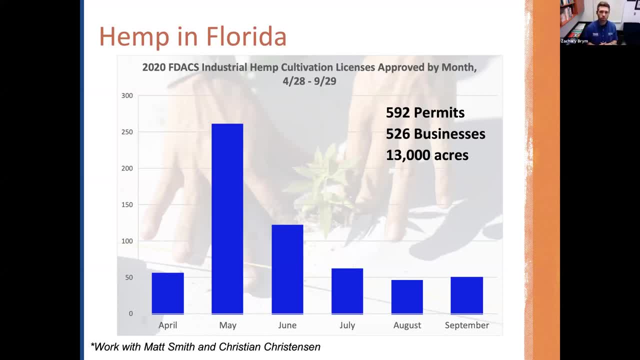 Well, the commercialization of hemp and licenses to private farmers. these numbers were initiated in 2020 with the Florida State Hemp Program. These numbers, of course, are already outdated, but this is our sort of summary for 2020.. So it was late April that those first licenses 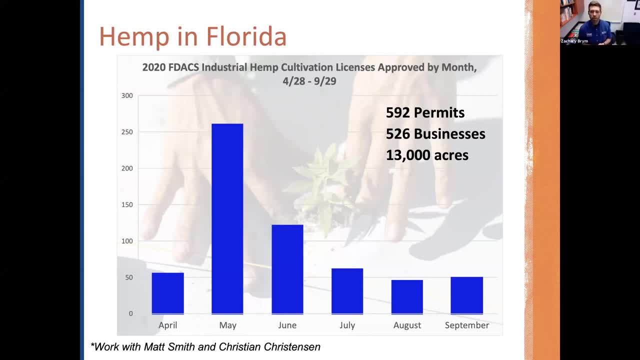 were available and you can see that folks really jumped at that opportunity. By the end of the summer growing season, in September, there were almost 600 permits For just better than 500 different businesses accounting for 13,000 acres By the end of the year, let's say turn of January, February. 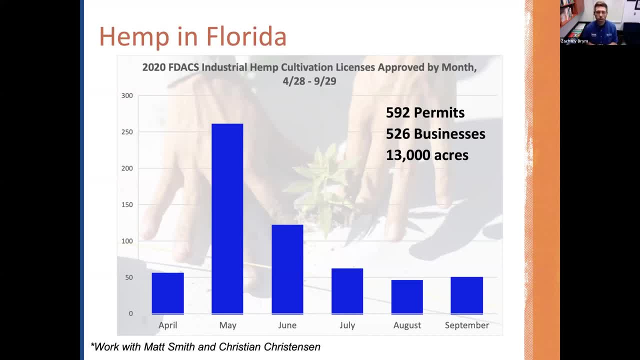 this number had already increased, maybe 21,000 acres. Also, reports that I'm hearing from FDAC suggest that maybe 1% of that acreage is actually planted and harvested. So from my understanding, from my knowledge, lots of folks have licenses, but we're still trying to do it. 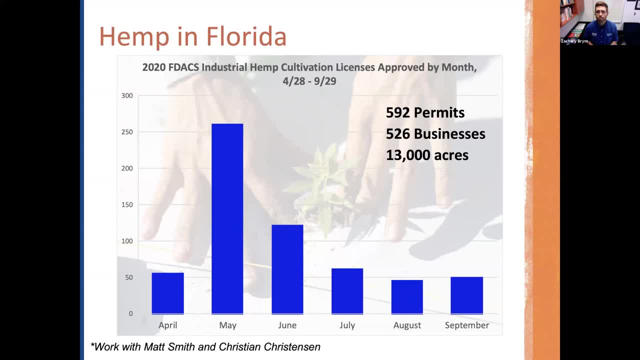 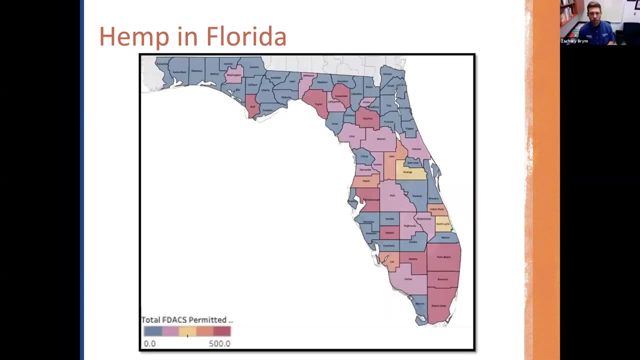 So we're still sort of feeling out the acreage that's actually active in the state. I'd like to acknowledge some work with extension folks at IFAS, Matt Smith and Christian Christensen, for helping me collect this information. These are those numbers put out on the map. 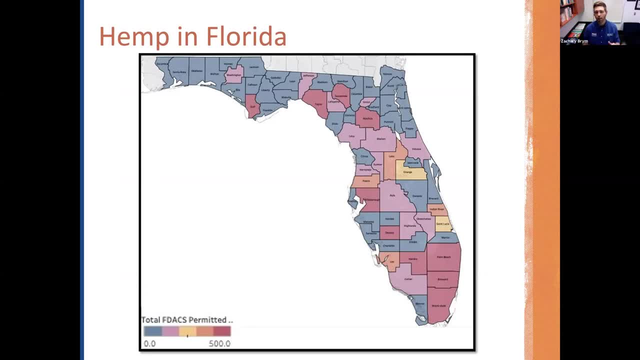 So we see 500 acres or better per county common in the Southern part of the state And and several other counties with large acreages permitted as well, but also sort of not quite ubiquitous. We'll be following up with this information multiple times throughout the year. 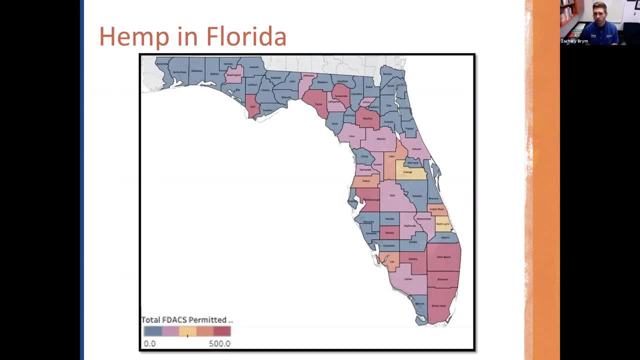 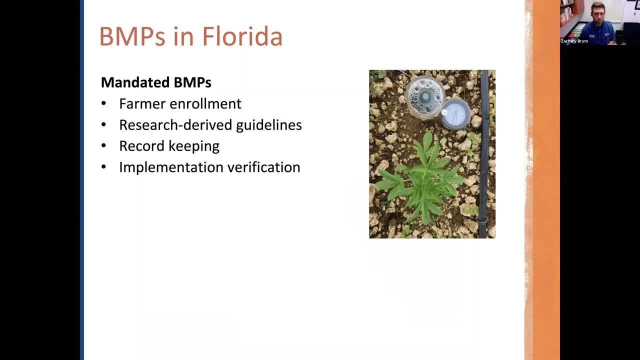 just so we can keep track. The takeaway is that hemp's here as far as a commercial opportunity. farmers are getting licensed. Exactly which farmers are going along planting a crop, being successful with that crop, It's still to be determined Now, as these farmers are getting set up. 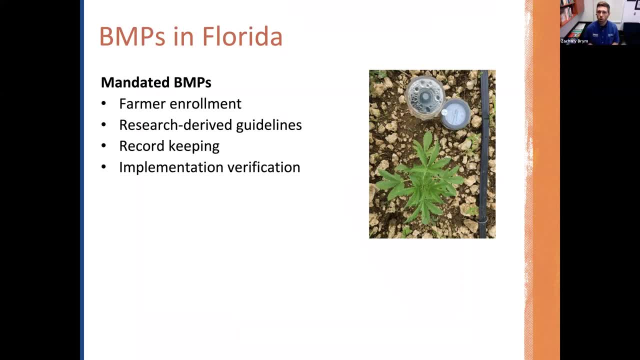 getting their licenses. they're also required to be enrolled in the BMPs program through the state, And so I just wanted to take a minute here. And in many ways, hemp is a new crop. Hemp is a different crop to many others of the established crops in the state of Florida. 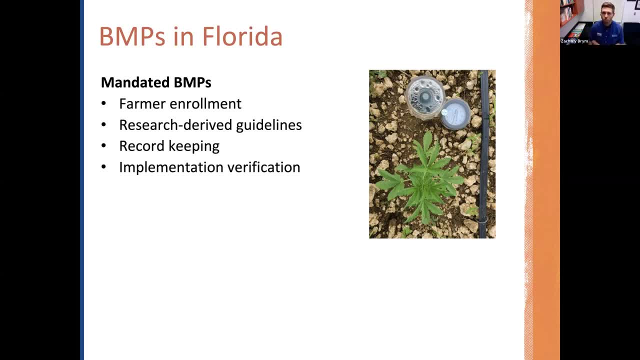 But sort of worth walking through how hemp is the same and hemp's different. So hemp is an agricultural commodity in the state of Florida, which puts it under the regulation of the Florida Department of Agriculture and Consumer Services And that ultimately puts this crop in any land. 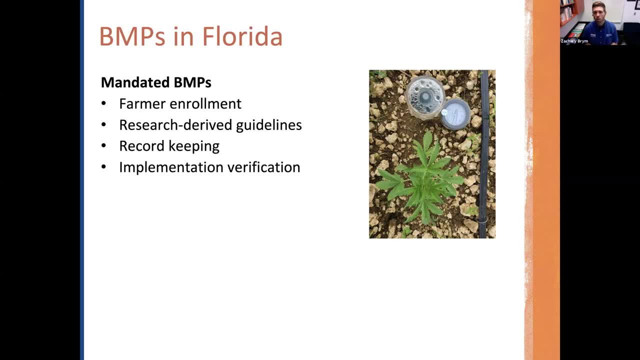 in agriculture under these BMP mandates. So farmers have to enroll in the BMPs. BMP manuals and guidelines as they come out of the university are expected to be a research derived research specifically from Florida And along with following those recommendations and guidelines, the farmer is expected to keep records. 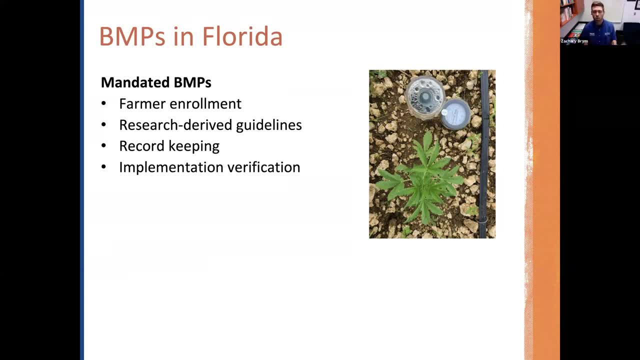 so that they can keep track of what they're doing And also when the state comes along and looks to ensure that they're operating in compliance to their BMP enrollment, they can do that through the records and implementation verification. So just a couple of points to emphasize. It is expected that hemp farmers are enrolled in the BMPs. 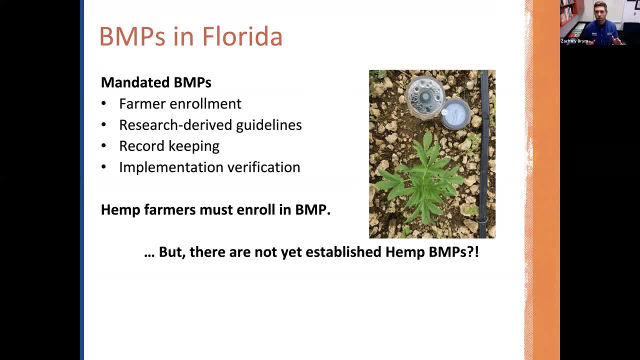 but there aren't really established hemp BMPs for the state of Florida. We, as the university, got out with our first planting in 2019 and that was a variety trial, a planting date trial 2020 came along, our first attempt at some fertilizer research, and you'll see the results of that here. 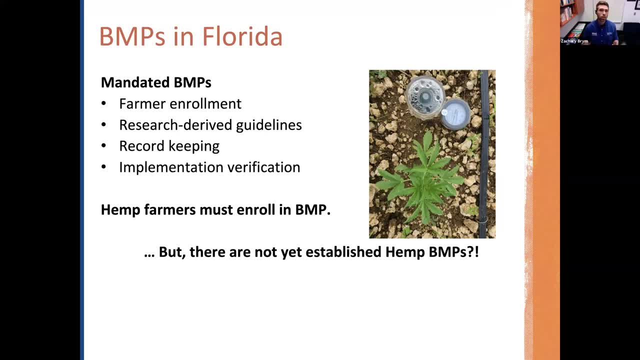 In order to have a recommendation out of the university, you need to have research, and so we're kind of in a chicken or the egg situation. We do have some guidelines that are out based on research from other states, but this is an ongoing and important sort of situation to keep up to date on as the 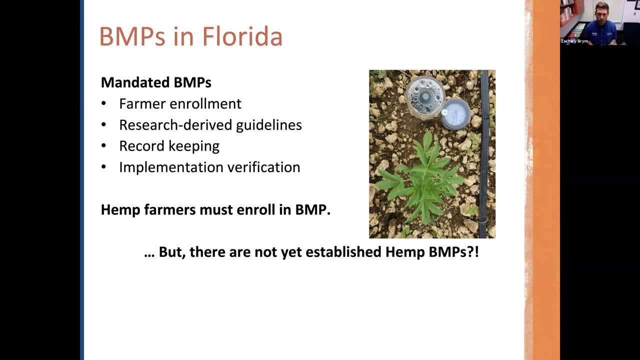 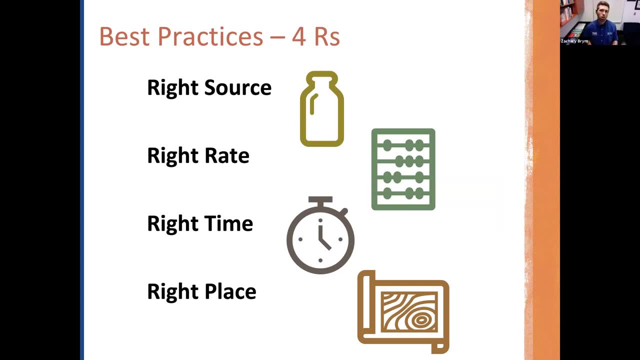 research out of the university continues to get established as our information continues to get out there. So it's really important to be working with your FDACS agent on your enrollment And be thinking about these really basic principles in order to be appropriately managing your nutrients on farms. So these are the four R's. you'll see these in the vegetable manual and 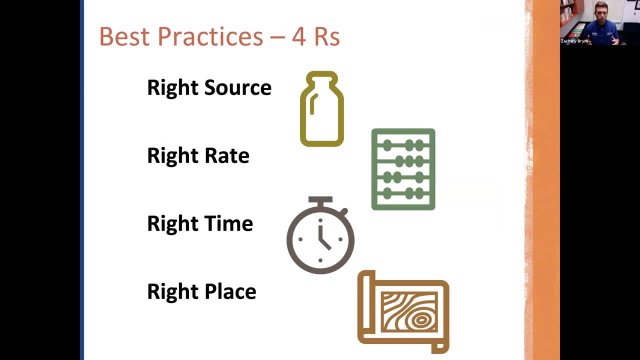 the citrus manual. Really, anytime someone's working to describe best practices in fertilizer management, we're talking about these four R's. So the right source, the right rate, the right time, the right district, the right следующая, the right rate, the right time. we're talking about these four R's. The next one is the factory. We're talking about the one year and the other. so just the right source, the right rate, the right time, the right time, the right produce, the right natural environment, the right fertilizer management. So we're talking about four R's. So you look for the right tradicional interventions and the right 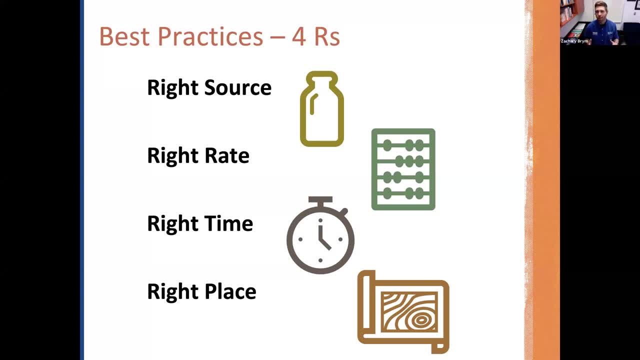 process and the right application And you'll hear from the agriculture department the right time and the right place At this time. these are sort of the best approach to fertilizing hemp, just by being mindful and ensuring that you're being a good steward of that environment, of the 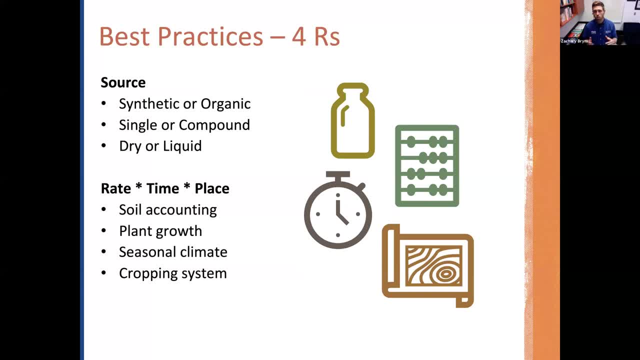 water quality. So just because this is such an important topic, I wanted to take an extra moment to describe some of these things. So the source: you can ask yourself: is it best for my farm, best for my environment, to come from a synthetic source or an organic source? That'll depend on. 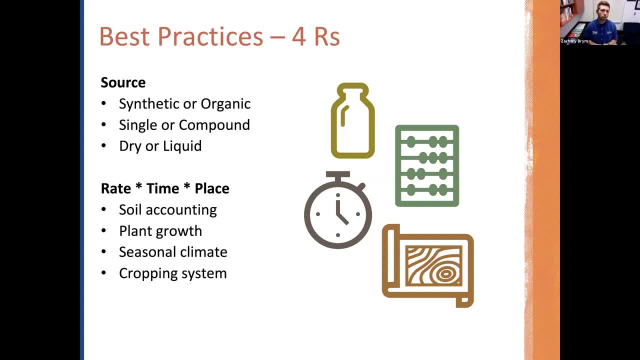 your farming system and your long-term goals for your farm, If the source of fertilizer is going to be a single compound, for instance nitrogen, or if it's going to be compounded across multiple. So you'll commonly see fertilizers that are mixtures of nitrogen, phosphorus and potassium. There again, 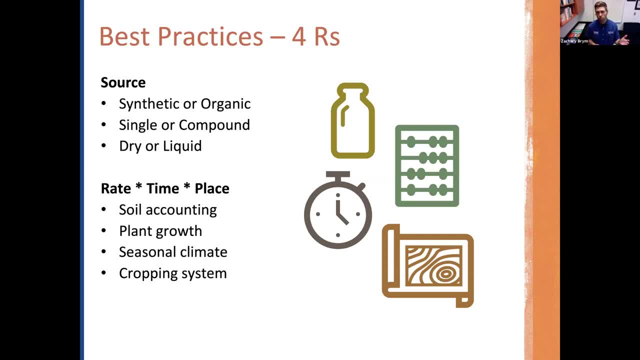 based on your system, based on your crop, you'll ask yourself whether or not it's best to apply as a dry source or a liquid source. So we don't necessarily have a whole lot of answers specifically for hemp about how to be doing this currently, but it is important to be thinking. 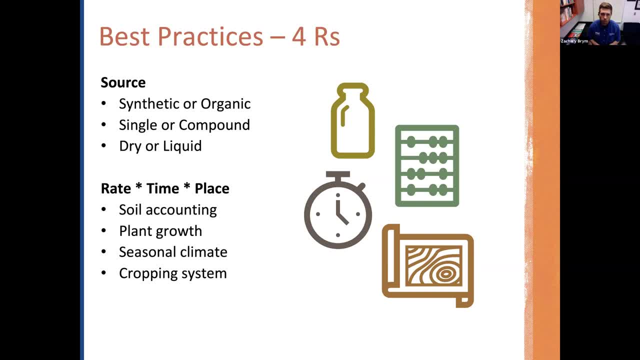 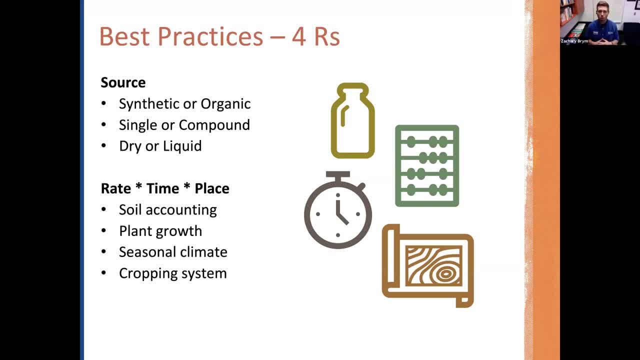 yourself these sorts of questions. So what is the fertilizer? excuse me, what are the nutrients existing in your soil? So can you account for the nutrition in your soil, for the organic matter in your soil? How does this relate to the plant growth? So it's probably not a good idea to be. putting a lot of attention to the organic matter in your soil. So how does this relate to the plant growth? So it's probably not a good idea to be putting a lot of attention to the organic matter in your soil, So how does this relate to the plant growth? So it's probably not a good idea to be. 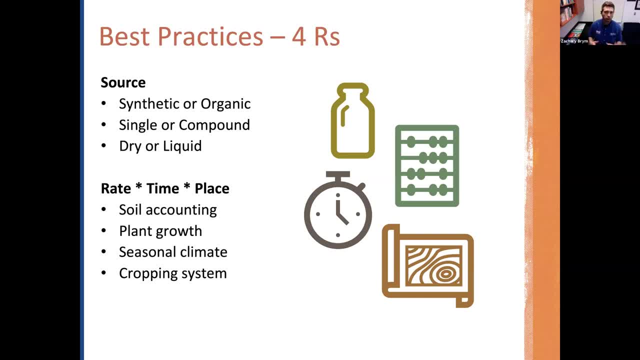 putting a lot of attention to the organic matter in your soil. So how does this relate to the organic matter in your soil? So how does this relate to the organic matter in your soil? So you're putting on a whole bunch of fertilizer months before your crop goes in the ground. 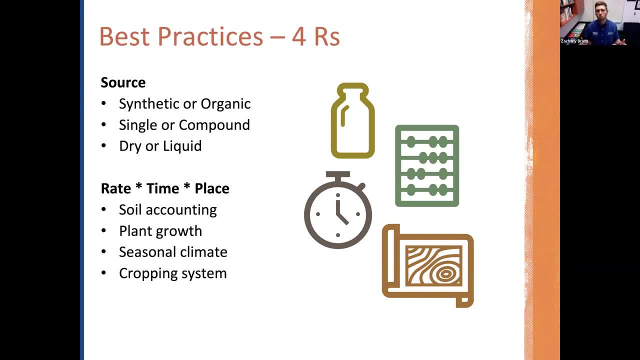 it's going to rain and the fertilizer is going to be leaving the soil before your plant has a chance to take it up, So making sure that you're timing that up. Small plants probably need less nutrients than big plants that are putting on flowers, for instance- another sort of aspect to 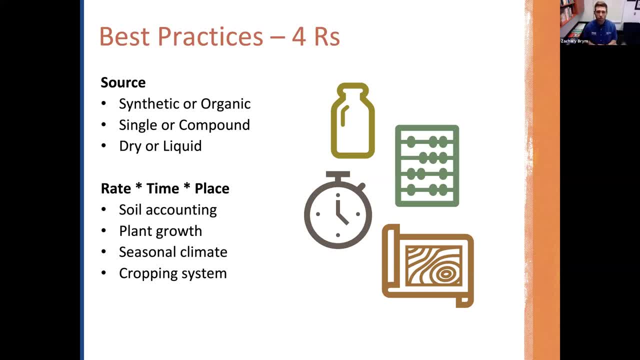 be considerate of Also. of course, these things will change by season. The dry season is going to be a much different scenario than the wet season, So it's probably not a good idea to be putting a little nitrate in that fertilizer- And I mentioned that several times. the cropping system: 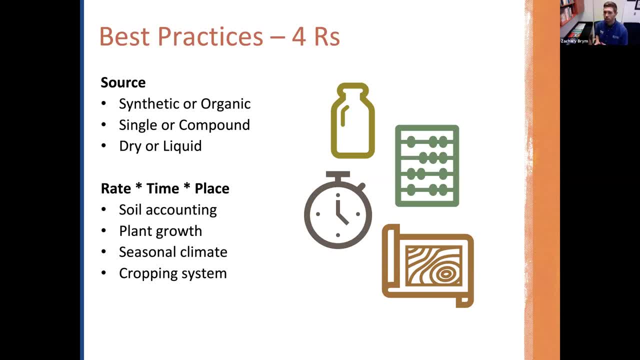 that you're choosing, nutrient management is going to be different in a fiber system than it is in a in a flower system, And so just to like summarize and sort of put this on the nose, for for what a good four R's in the hemp space with the lack of information that we're dealing with. 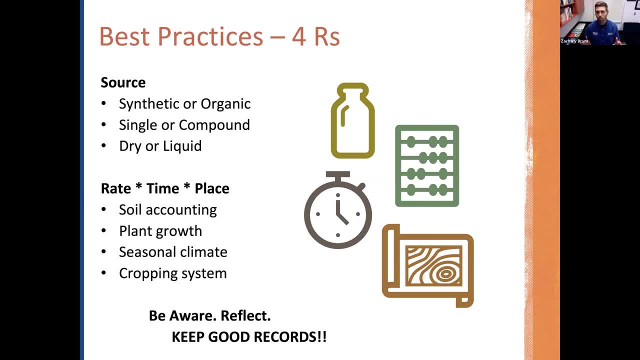 these days. Be aware of your, your crops, be aware of your farm, take extra time to reflect on the nutrient management process and drop it off on a tone chart now and then you know you'll have a good apareance in kind of almost any single safety settler on the dude in the container at 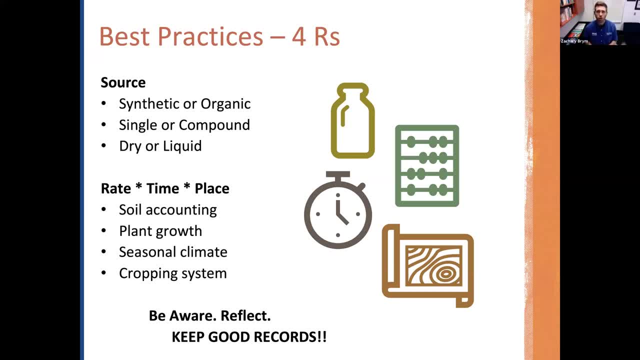 your intuitions right, Then you know. once it turns into something like you, then you just know the world you're working it off. So consider any detail you're looking to point out. want to management. I'll go through some information that you can draw from in that reflection. 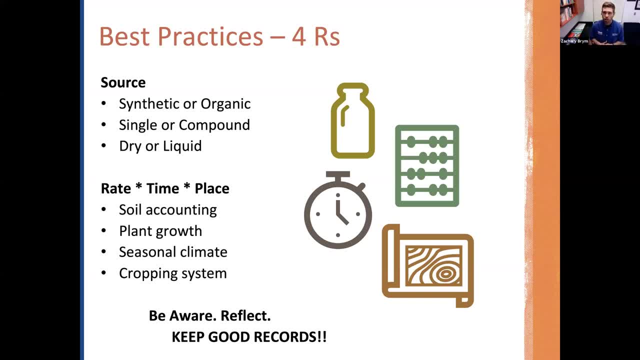 You could also do it by observing your plants and how they respond to very different nutrient applications. Definitely can't hurt to go slow with a little bit of land as you're getting started in the industry And as a data scientist, as a scientist who's interested in information. 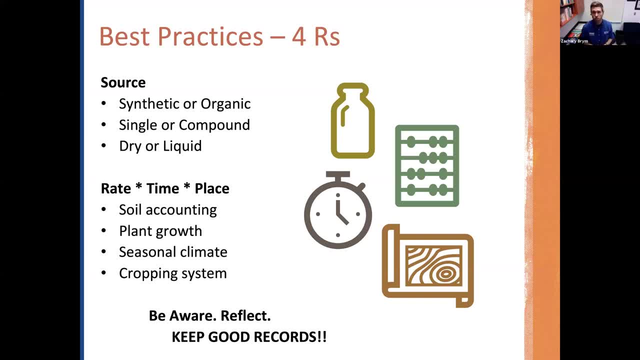 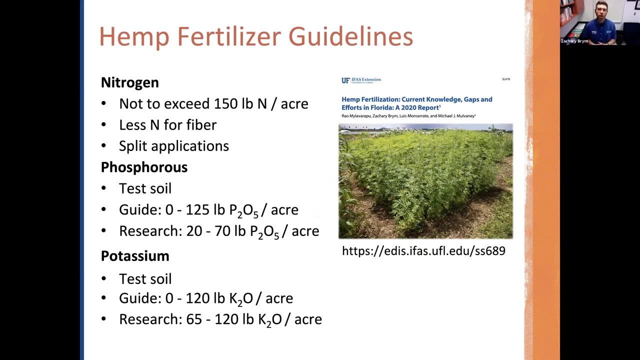 and record keeping. of course, I'm going to say: keep good records so that you can reference them, but they'll also be critical in having a good experience with your FDACS inspector. So we were able to put something together based on existing research from around the 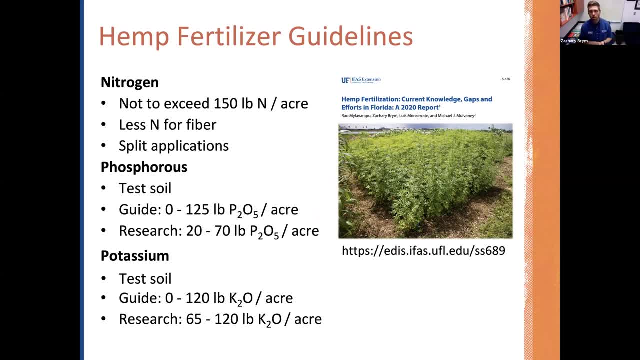 world, not from Florida, but from around the world. And I'd like to recognize my co-authors on this document: Raul Miller-Arapu, a graduate student of mine, Luis Monserrate and collaborator Michael Mulvaney. And so what we did was a broad literature search of hemp nutrient research historically. 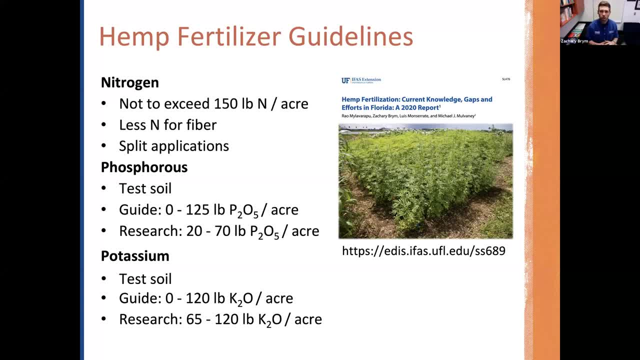 And we also reached out to folks in other state analytical soils labs to see what their recommendations were in those states and kind of how that might inform our approach to Florida. And so to be very specific about the words that I used here, these are our guidelines. 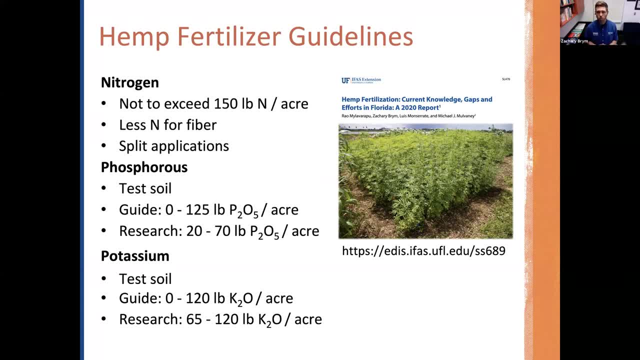 This is a report of our findings. preliminarily, We are working on the research that would end up being more appropriate as a recommendation. So just to read through here the slides: Nitrogen: Not to exceed 150 pounds of nitrogen per the acre. This is something that we have. 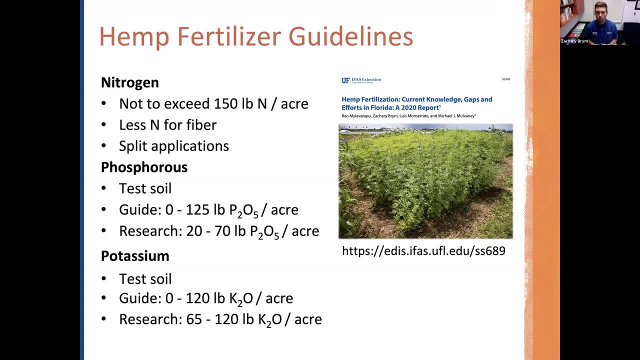 seen in the research. They want to know more about it. What's the percentage of nitrogen? that I'll show you. But also, if you over apply the nitrogen specifically for fiber crops, for instance, we've seen that the hemp crop will take up extra nitrogen. They call it luxurious uptake. 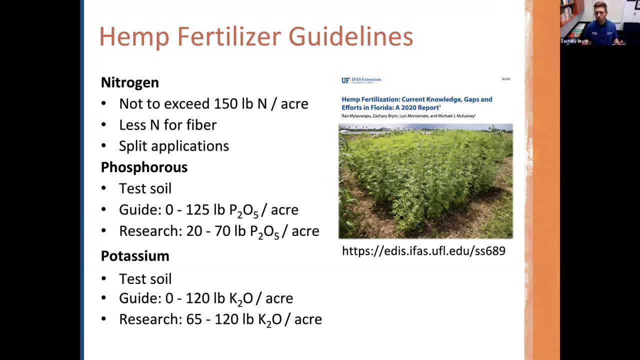 It'll take it up and it won't benefit the crop. In fact, in terms of fiber quality, too much nitrogen will actually reduce fiber quality. We've also seen a couple indications that too much nitrogen can reduce the cannabinoid development as well. So back to that point. 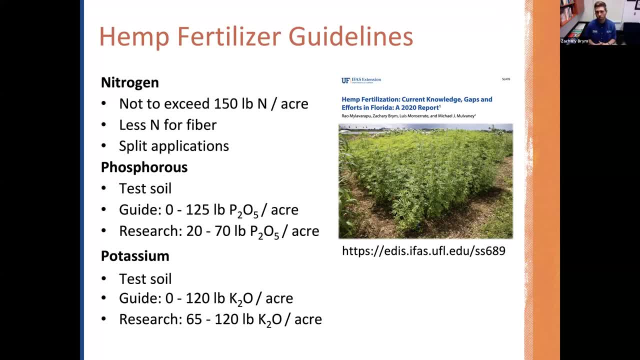 about nitrogen. you probably don't even need 150 pounds of nitrogen for fiber crops. As Florida tends to be sandy and low organic matter in nature, water passes through the soil very quickly. We recommend that these nitrogen applications are done in split applications so that you can. 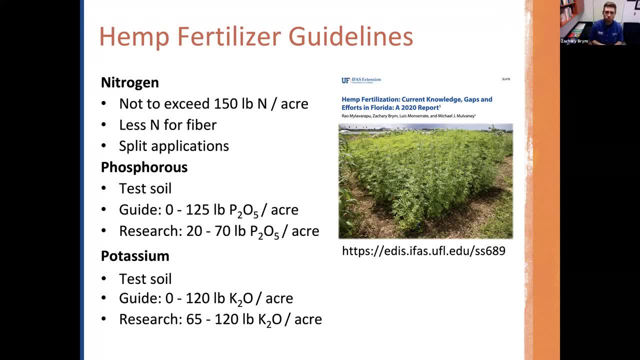 spread, Spread out across the year and make sure that the nitrogen you are applying is going to the plants. Phosphorus- this goes back to kind of being aware of your soil, accounting for what's there. We definitely recommend soil tests so that you can see what's there. The guide helps break down soils. 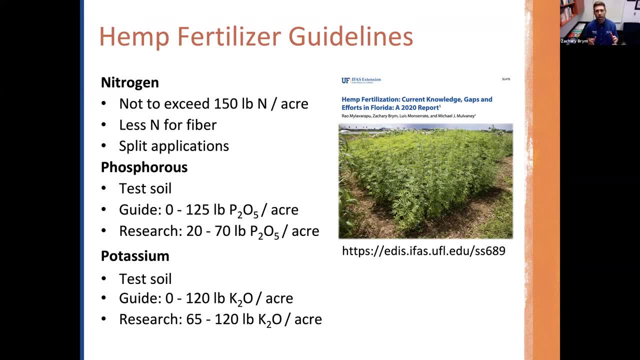 into low, medium and high phosphorus, And the guide, as it's published, recommends that you use a lot of phosphorus in your soil. So if you have a lot of phosphorus in your soil, you can use a lot of phosphorus in your soil. So if you have a lot of phosphorus in your soil, 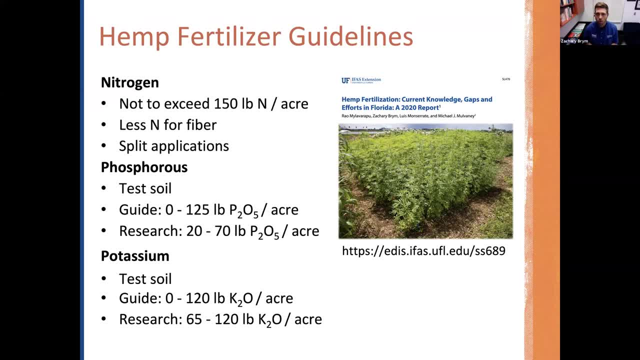 you want to recommend somewhere between 0 and 125 pounds of potash per per the acre, But really what we've seen from from the research is is something in the middle, Somewhere between the 20 to 70 pounds of of D2O5.. Potassium is something similar. Again, test your soil, know what's in. 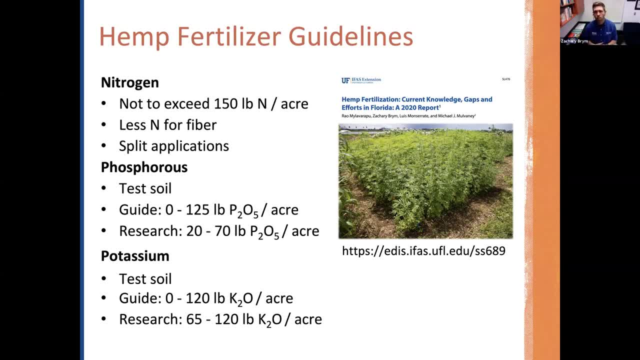 there as background rates. What we are seeing from the research and from other states is somewhere between 0 and 100, I would say twice aÉ- 100 pounds of K2O, probably something more. So potassium is probably something that hemp does. 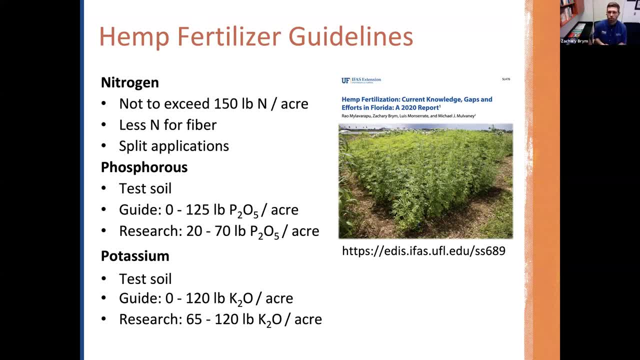 need in a reasonable rate. So the 65 to 120 is what we are seeing there. Just again, to emphasize a couple of these caveats based on this report from 2020, all of the research and information that we gathered for this report was from outside of Florida, So we're working really hard to get. 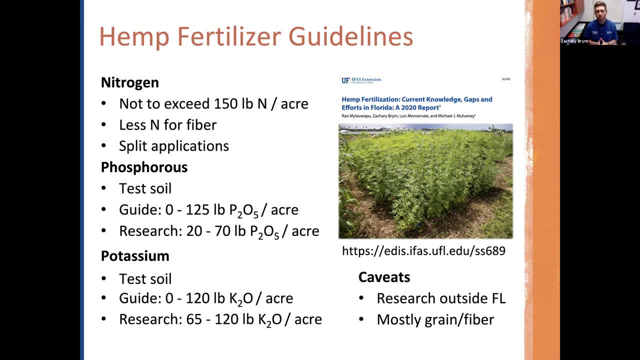 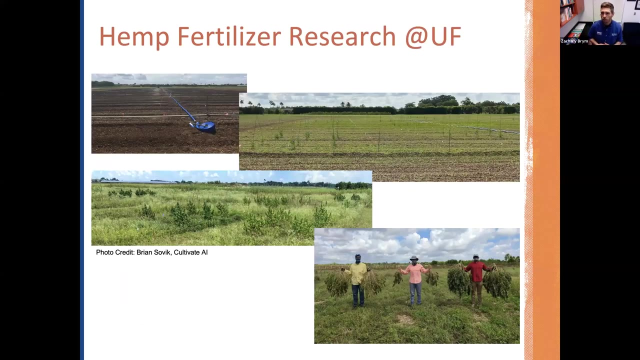 that information for Florida. Also to point out that the abundance of research out there on hemp fertilizer is primarily for grain and fiber cropping systems, And so we're still working to catch up on the flower systems as well. So the rest of this talk is just to kind of. 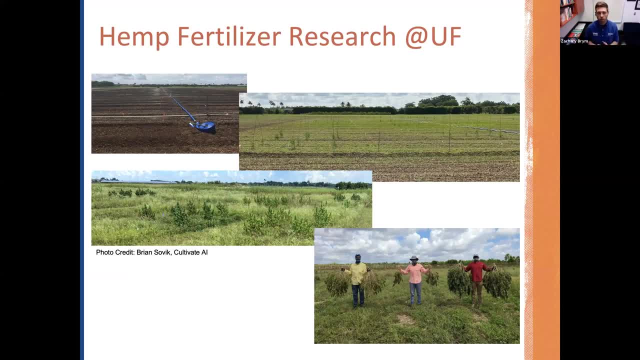 go through give you an idea of what we are working on here at UF, IFAS for hemp nutrient management, And this study was started last year 2020.. This is here in Homestead, So very calcareous gravelly soil pH somewhere around 7.5, just to link up the comments from before. 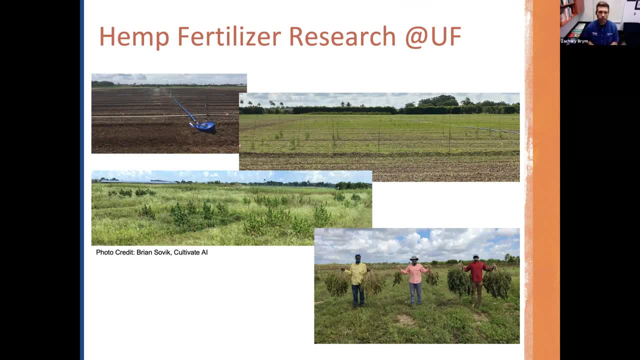 So we didn't change the pH in the soil, but definitely a reason to acknowledge that it's a single site, a single year so far. This was a cultivar called Weiss that we transplanted out into the field And we put on six different nutrient applications. 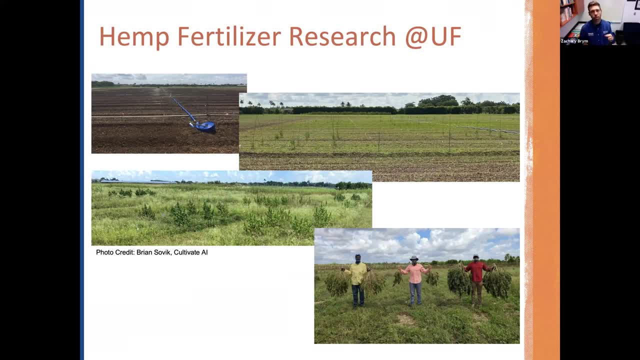 from 0,, 50,, 100,, 150,, 200, and 250 pounds of nitrogen per the acre. And, as you can see from the picture in the right, we did have a lot of nitrogen in the field, And so we did have a lot of nitrogen in the field, And so 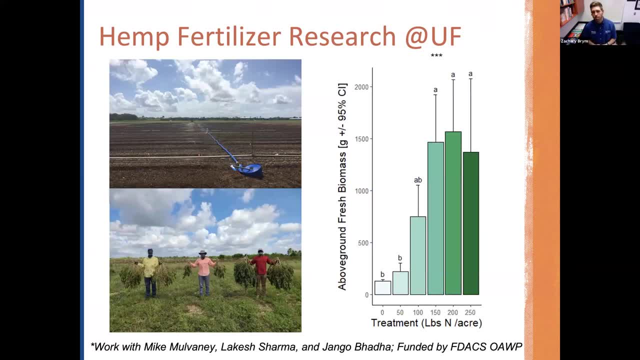 some differences that we saw in the treatments And so, as I mentioned, the fertilizer guideline document suggests not to exceed 150 pounds And we saw that in our research last year that there was no benefit to hemp biomass- the total mass of the plant- by exceeding that 150 pounds. 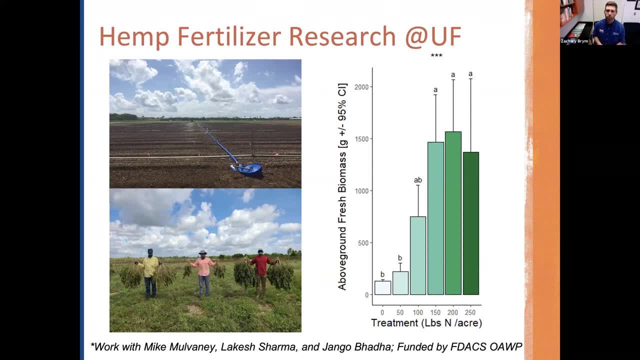 So 100 might be good, but it's not going to be good, And so we did have a lot of nitrogen in the field to support the seedlings. But some differences that I noticed with the fertilizer guidelines is that they've been in the soil for very long, So the noted value is now. we didn't have a tendency to. 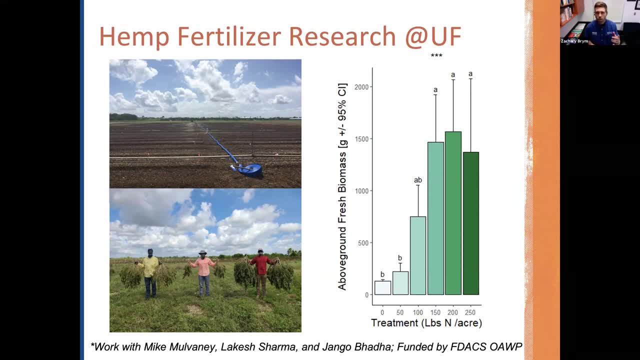 have a lot of nitrogen, So it's going to be good to have a large size of fertilizer, And so we I'm going to put in some locations that we can get the most nitrogen in, And then we can put in a lot of nitrogen in the soil that we think we can get the most nitrogen in, And then again. 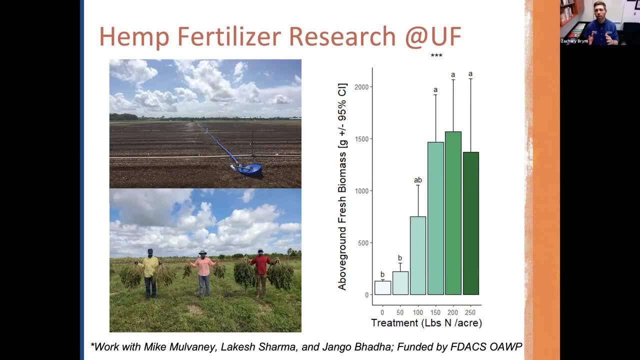 we're not going to have that high of a potential to actually support the seedlings, So we're going to have to get the highest possible level in the soil, And then we're going to have a lot of nitrogen- this one here this coming year- And so we'll be able to collect this information for multiple 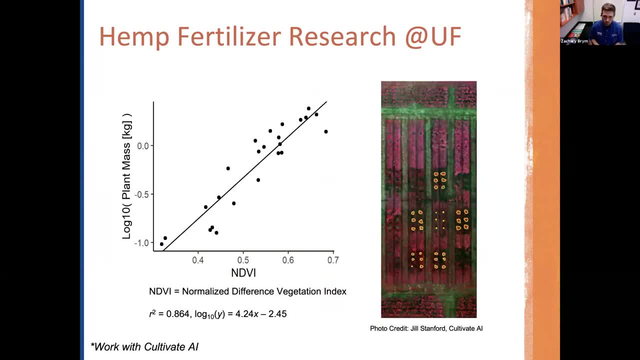 sites and ag environments across the state. I did also want to show this graphic. I think it's fun. I think it's the direction that we'd like the research to go through. I was working with a group, Cultivate AI. out of Orlando, They flew some drones- aerial based imagery. 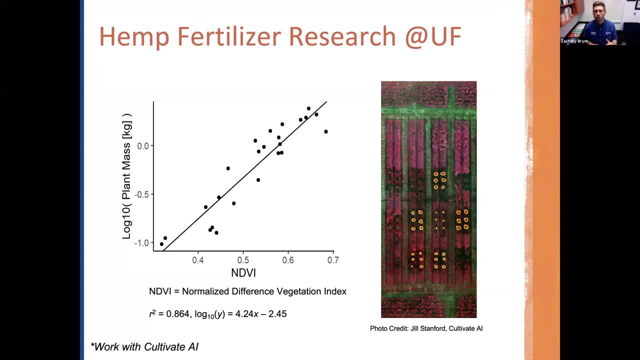 with the drones, And these images here are false IR images, And so having the opportunity to calculate a vegetation index that uses a red and near infrared bands of light in order to do that, Just a takeaway message here is that what we're able to do is capture differences in plant health that are associated with the nutrition. So, in addition, 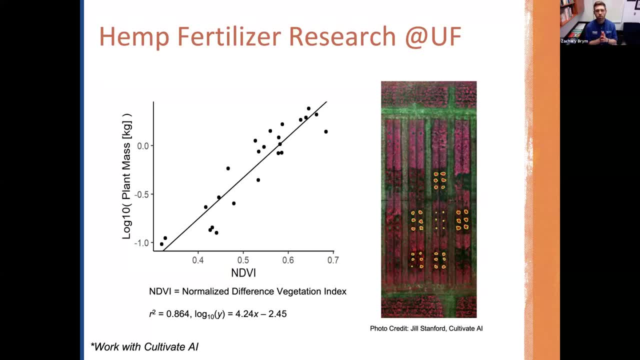 to the size of the plants lowering. we also saw a difference in the vegetative index And so the plants that were more healthy that 150 pounds of nitrogen also. we were able to capture that from these aerial images. So stay tuned for some more of this work as we expand the program. 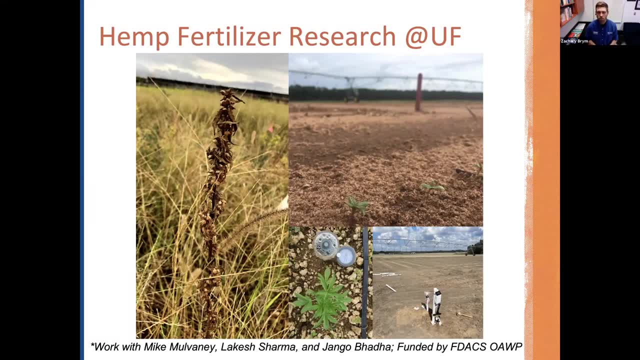 As I mentioned, expanding the multiple sites, We installed some soil sensing equipment across the site, So some drain gauge lysimeters out in the Citra location. We're also expanding So that one trial, the pilot trial last year, was just the flower system. 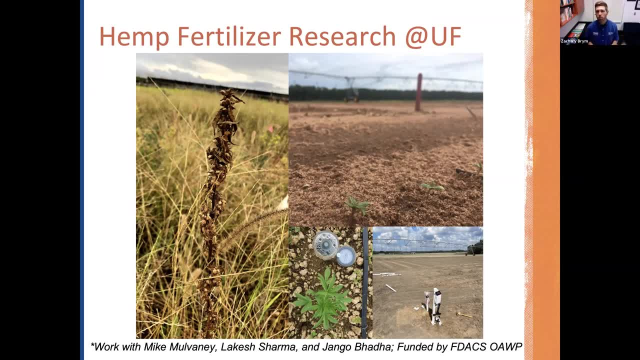 That just did a great job And we've got the majority of the issues with the transfer systems that we've covered. And all of the issues we've got at this point today are the bedding conditions and soil loads, as well as in the soil, storage and storage. 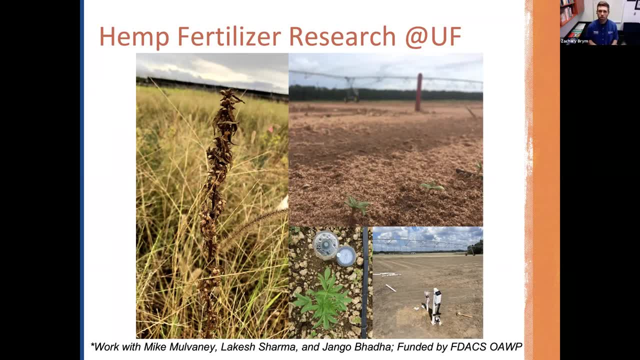 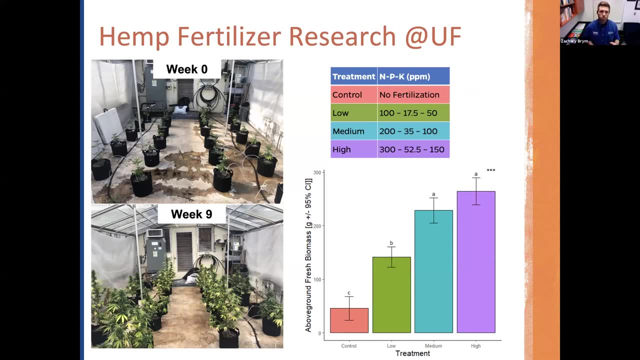 systems. So we've got some of the concerns surrounding flood control and our plan to continue to focus on that, And we've got a lot of such issues. So I immediately confirmed that we were able to do the synopsis of these outcomes in one week And then at the same. 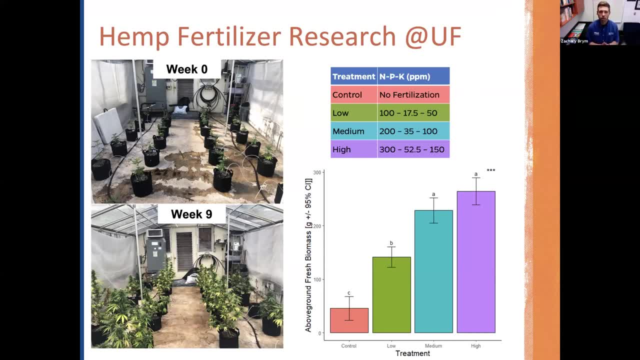 And so this is a container study where he changed fertilizer upon flowering, So it's more a fertilizer supplementation. So these plants were maintained similarly up until the experiment And then, sort of at flower, he changed this NPK at a consistent ratio at these different 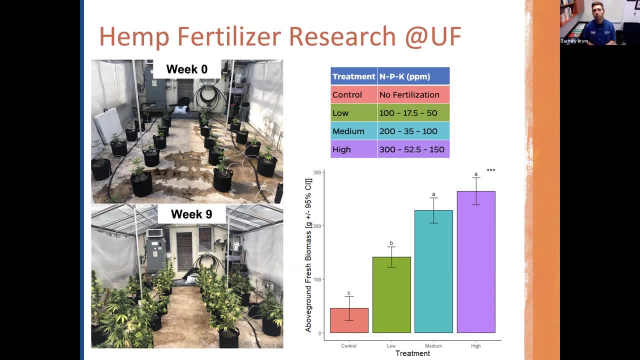 rates 100, 200, 300 parts per million of nitrogen, And we do see sort of increasing biomass for the increasing fertility, but not necessarily statistical increase after the medium. So again, these plants will take up luxuriously the nutrients, at least the nitrogen and potassium. 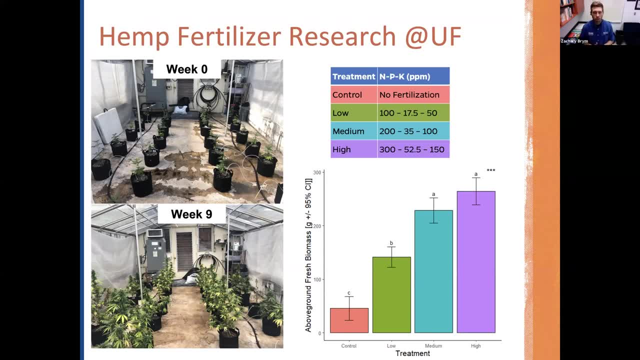 that we give them, But that doesn't mean that there's going to be improvement in the yield. So this medium, the 200 parts per million at least from this one study, is another indication for supplementing fertility at flowering. Interesting point to make here. 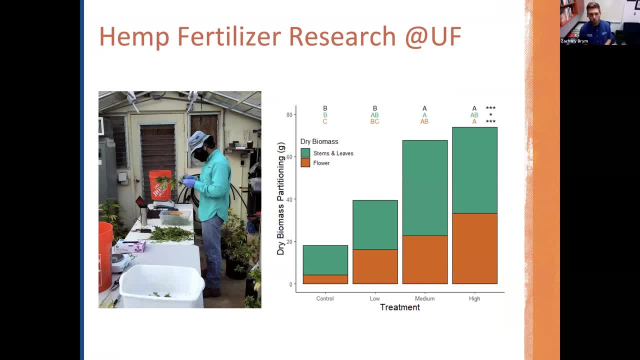 This is Luis separating out his plants into stems and leaves, away from the flowers, And so the nutrition could also change The biomass partitioning here, where the stems and leaves actually are more expressed in higher nutrient rates than the flowers. So again, more nutrients, more fertilizer does not mean more flower. 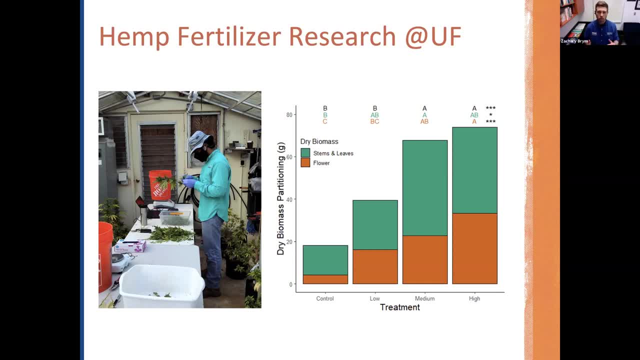 So if you're going after more flower, you're going after fiber quality. it seems to be that a more moderate approach to fertilization may not crank up your biomass, but it'll in the future. So again, we're going to have to wait and see if we can improve those qualities. 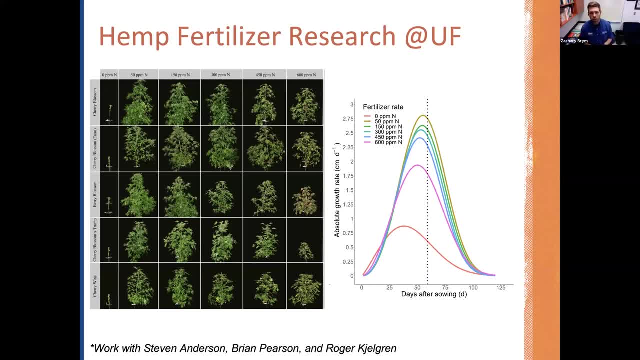 This is work done from the Mid-Florida Research and Education Center, My colleagues Steve Anderson, Brian Pearson and Roger Kellegren- really interesting work that they were able to do in a controlled environment, And so this scenario was one where the plants experienced a fertility rate consistently. 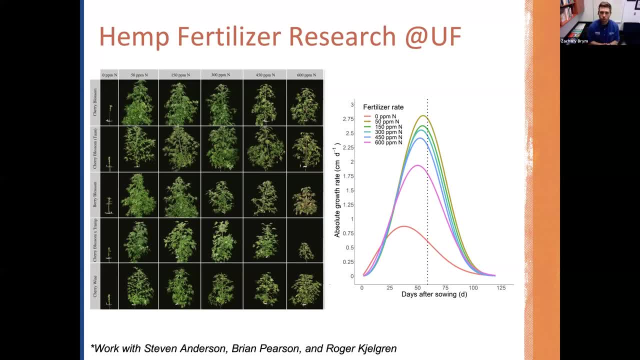 So they continued to flush out the container. And so they continued to flush out the container and make sure that these plants existed in these conditions from the 50 ppm to the 600 ppm. And the pictures tell the story themselves right That those lower nutrient rates- the 50, which is the line in gold or mustard yellow, tends. 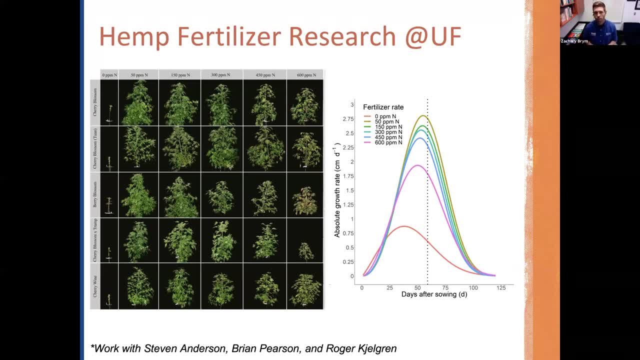 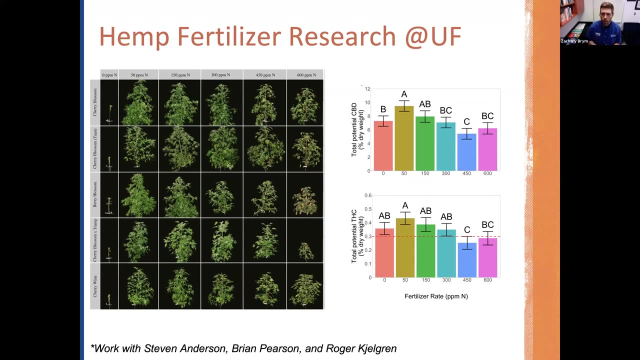 to have better growth and better outcomes than any of the greater fertility rates, And so just another way to look at it. Thank you, Thank you. That's another way to show that we can be moderate in our fertility management for this crop. This is another outcome from that same study, where the total potential CBD, cannabidiol and 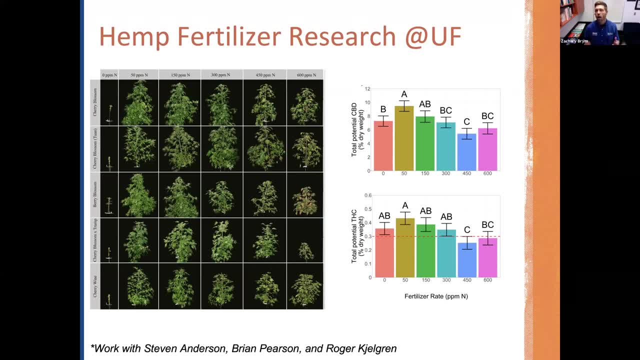 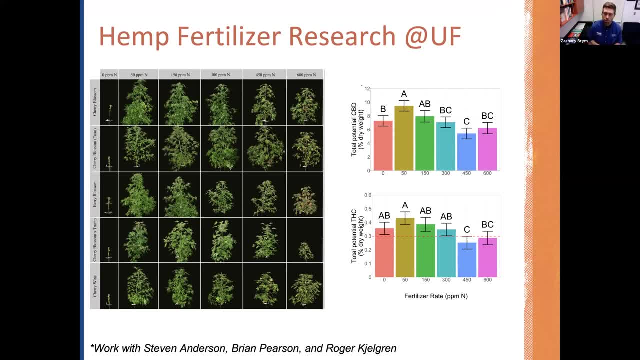 rates and declines are due to plant health. there's a lot of additional questions to ask, but some interesting preliminary results. You should notice that this figure puts a dotted line at the point three, And so this is something we have been seeing across our trials at the university plants. 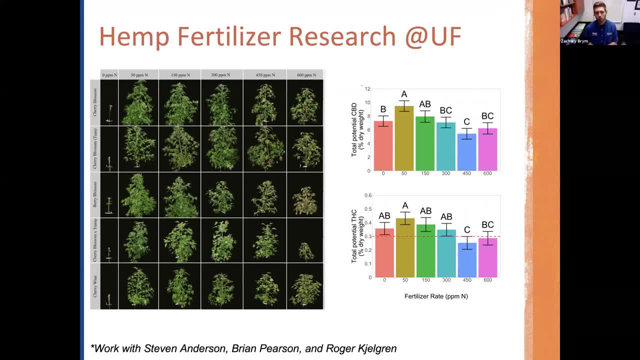 regularly going higher. Yeah, Yeah, Yeah, Yeah, Yeah, Yeah, Yeah, or exceeding that 0.3% THC. So farmers, hemp farmers- you're considering hemp farming- make sure you're taking those cannabinoid tests regularly and harvesting appropriately. 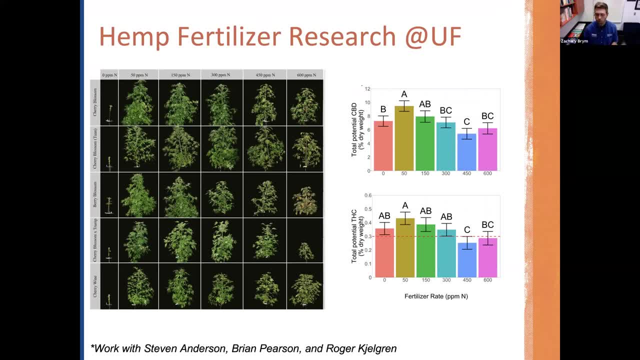 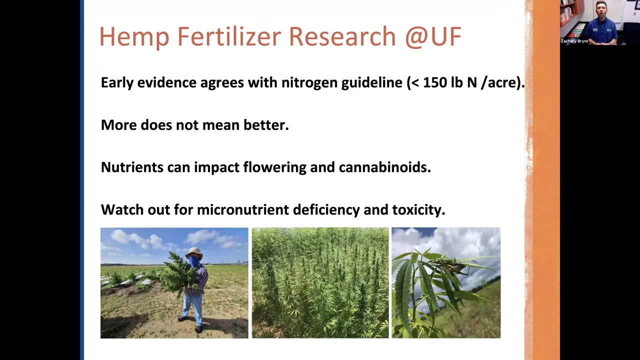 Harvest at the right time is one of those things that folks are concerned about. Definitely, something makes me cautious to acknowledge. So just to summarize where we're at so far with the hemp fertilizer research here at UF: the early evidence seems to agree with the research. 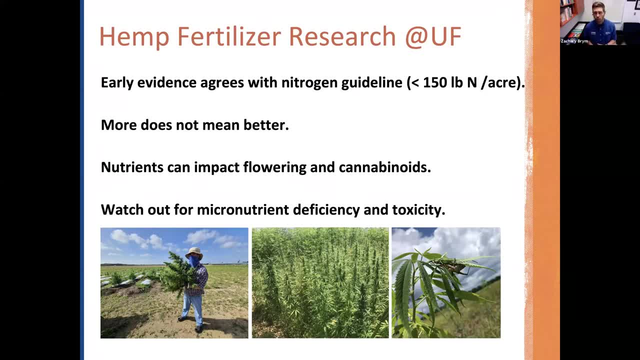 that we collected from outside of Florida 150 pounds of nitrogen per the acre, certainly not to exceed that. I said this multiple times through the talk: more does not mean better, And so, again, be aware, try some things, keep your records. 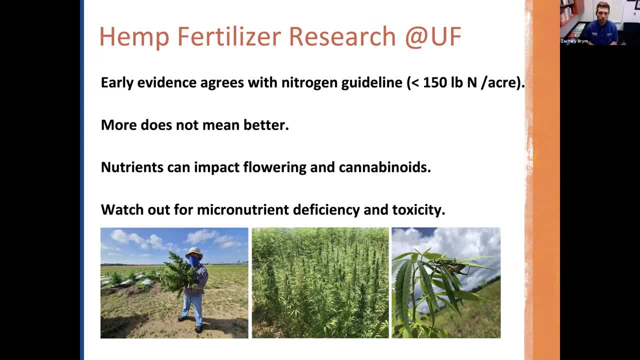 so that you can see what's working for you. I mentioned that nutrients can impact the cannabinoids. We also saw that nutrients can delay flowering. So more nitrogen than the 50 pounds to 100 pounds and greater may have pushed back flowering as much as two weeks. 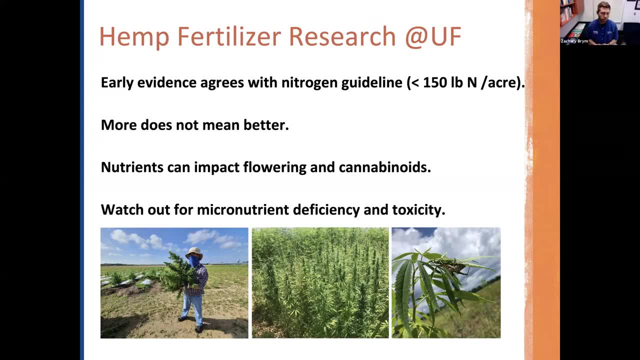 In the highest rates as well, that 200 and 200 pounds or 250 pounds of nitrogen out in the field in homestead. we saw manganese toxicity, So that was an issue that we saw in our trial. Luis also saw some micronutrient deficiencies. 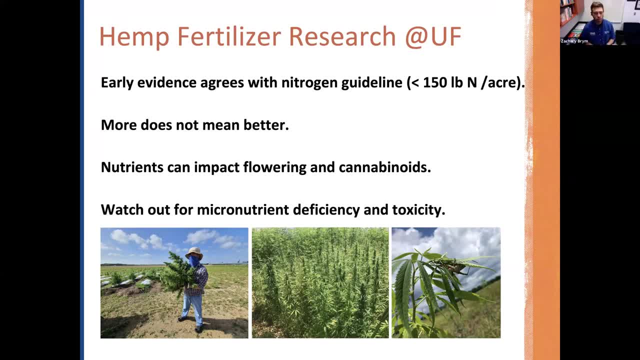 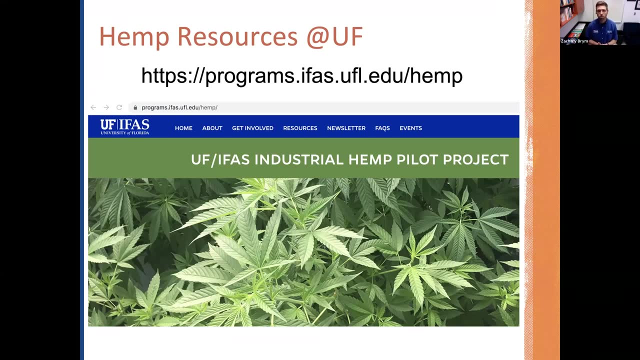 in the greenhouse study. So we're collecting leaf tissue samples in our studies so that we can follow along plant nutrition with the fertilizer applications. So with just the last couple, I'd like to acknowledge the resources that we do have available. This is the website for the UF hemp program. 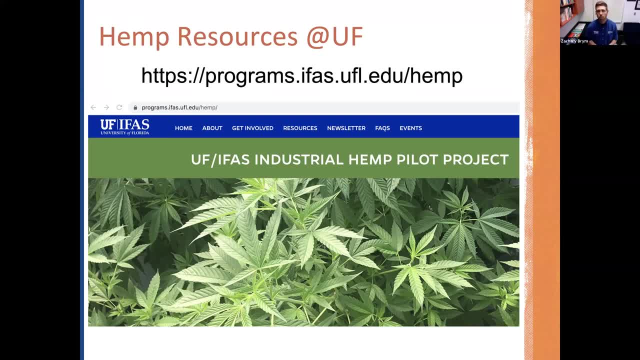 I welcome you to visit. We're gonna be continually updating our resources page for the upcoming cropping season. Actually, today was our first planting date down here in homestead. We got a planting date trial in for some grain varieties, So that's really exciting. 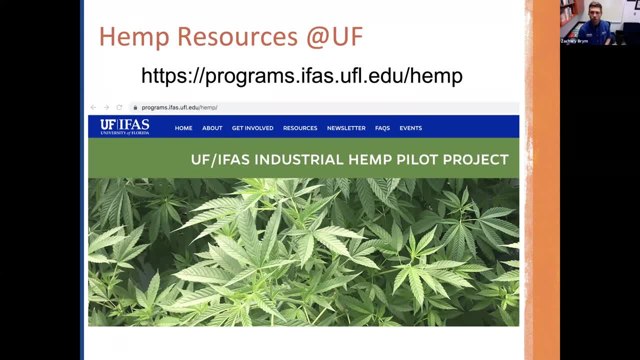 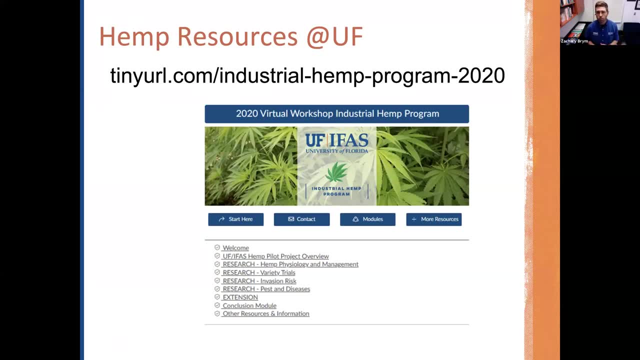 And we're happy to go along with the farmers This year and make sure that they have the best available information available to them. And if you're interested in what the UF hemp program has been up to, we put together this virtual workshop. It's reporting from our 2020 year. 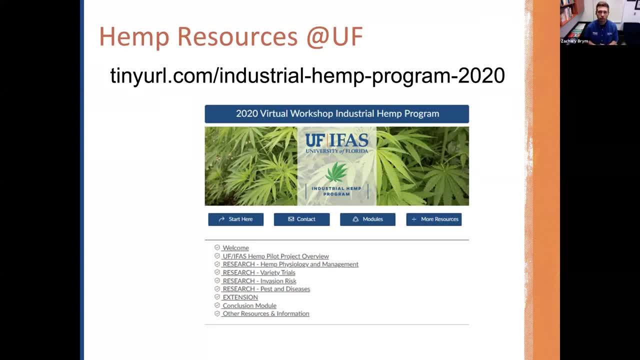 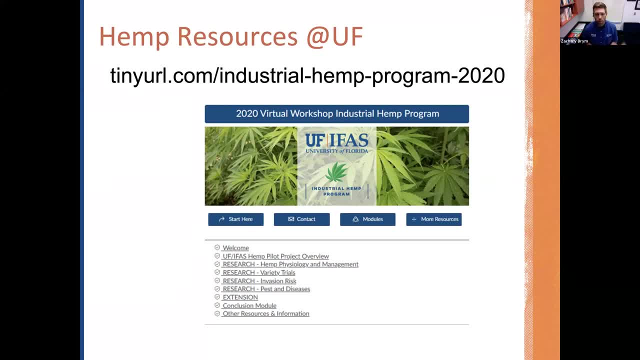 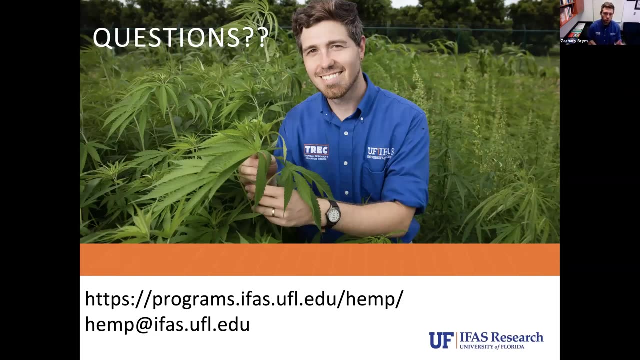 that have put up the information to share with the workshop participants And we'd be happy to engage you with the dialogue and have you along in the workshop group. So if you do have any questions, you're welcome to reach out. hemp at iphysufledu. 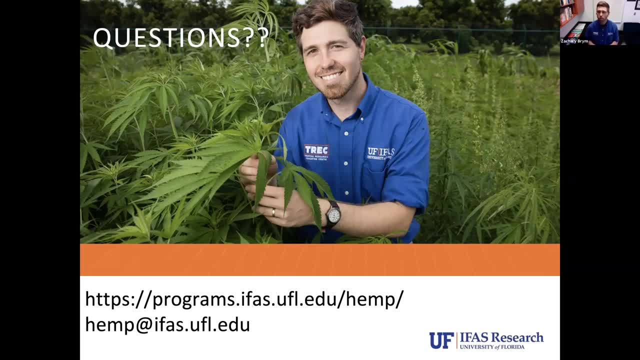 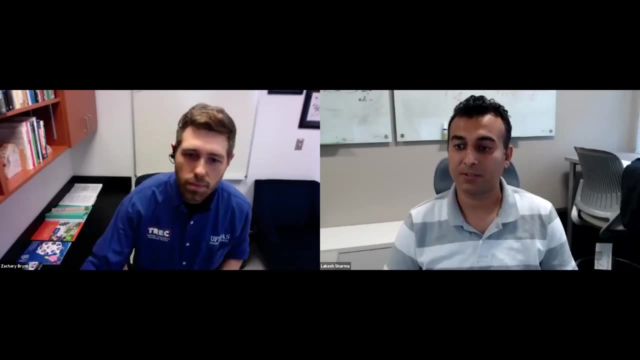 Check out our website, come join us on the workshop And with that I will. I'll take any questions. Thank you, Zach, for your amazing presentation. I will request audience. if you have any question, please type your question in the chat box. 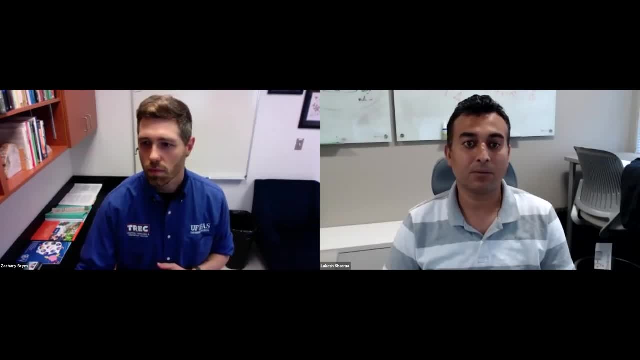 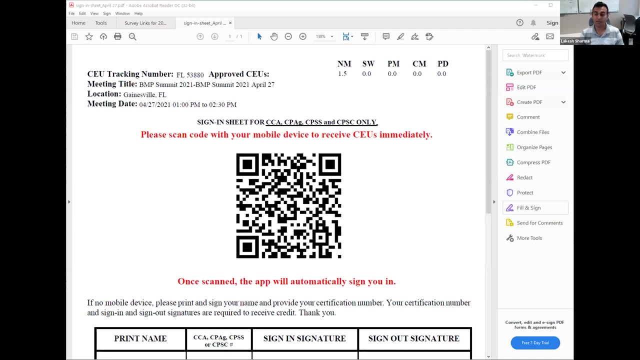 Emily, could you be able to put the QR code on the share screen And also if you can share the survey Audience? we have a very short survey, so if you want it for you to fill out, it will help us improve our programming. 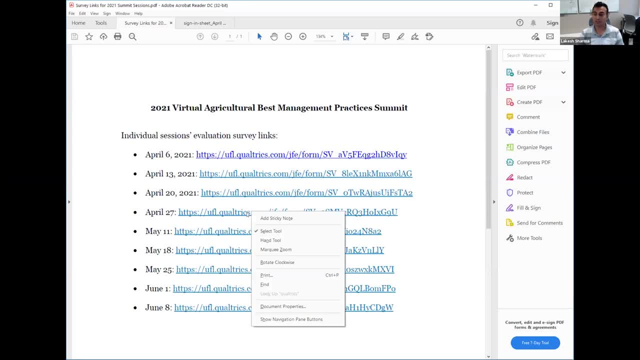 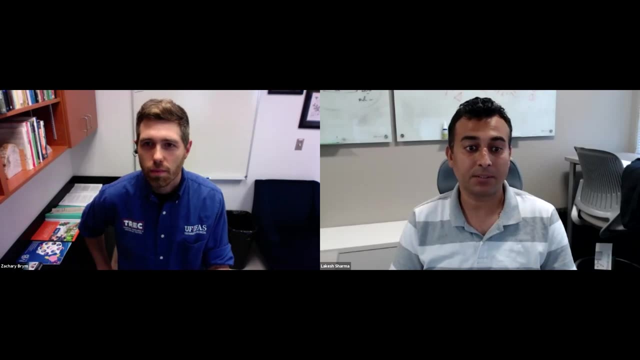 delivery and other aspects of extension. Please fill that survey, Emily. if you have that survey link in the chat box, that'll be great For the QR code. you can see screen very soon to scan that QR code. Thank you, I. 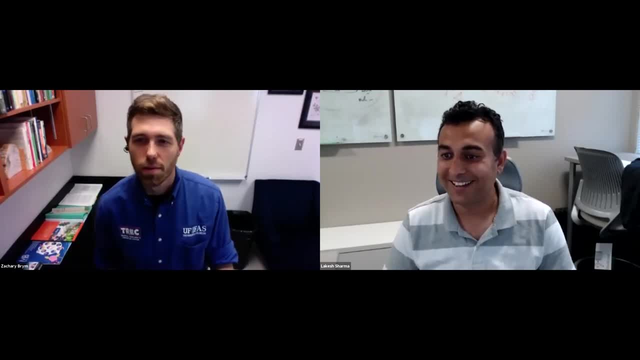 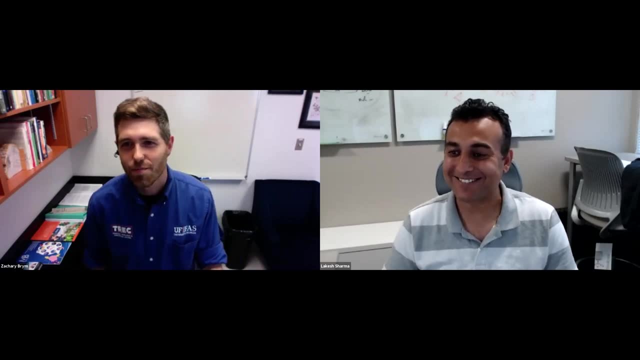 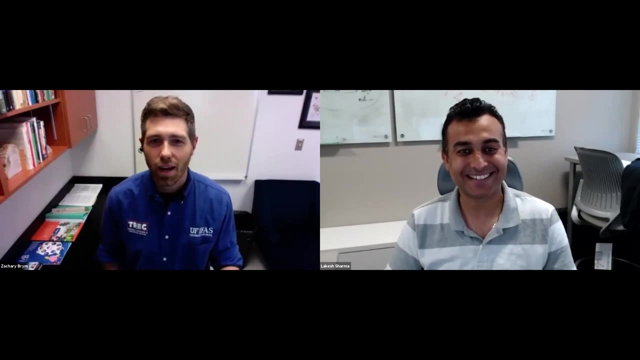 have found the QR code, Okay, So All right. Michael has pretty amazing question: how many jokes you have heard, Zach? Yeah, I mean all the time. they're happening all the time. You know the hemp joke just are endless. 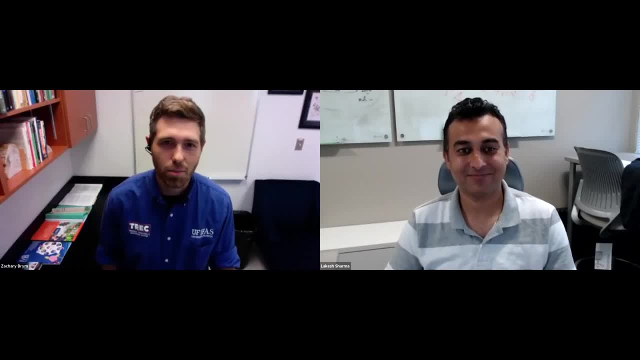 You know, especially when you start telling folks that some of your crops have beenold new. Yeah, that's true. Yeah, I mean there have been lots of things going the tendency to exceed that threshold. So, yeah, we're having a lot of fun. 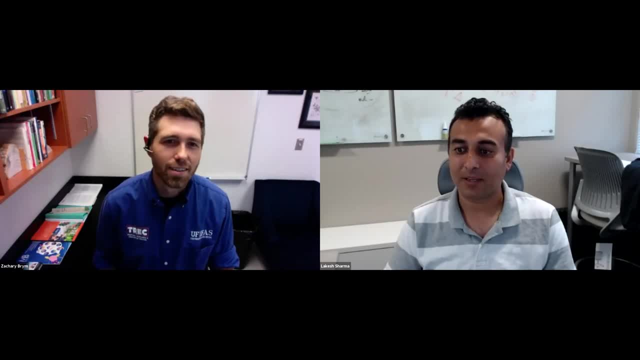 Great. So if you have any questions, please type that question in the chat box. I think Dee has asked Kelly if Kelly can help And I think Kelly already replied to that that he will be able to help Dee with her project on peanuts. 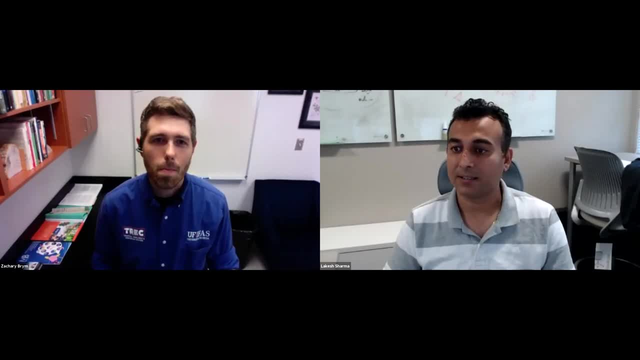 PH bicarbonate study in peanuts. So I think that's already addressed. Thank you, Dr Dukes, for sharing EDS publications: hemp fertilization: current knowledge and gaps and efforts in Florida 2020 report. Okay, We do not have any questions at this point. 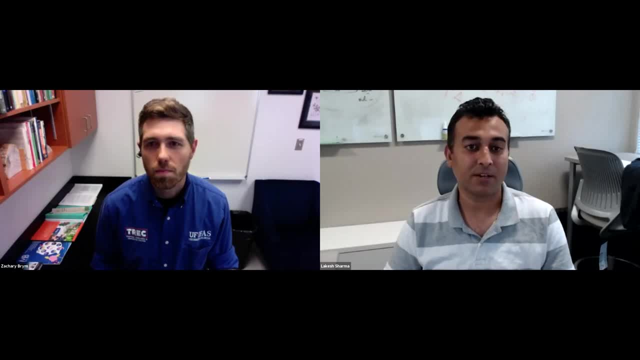 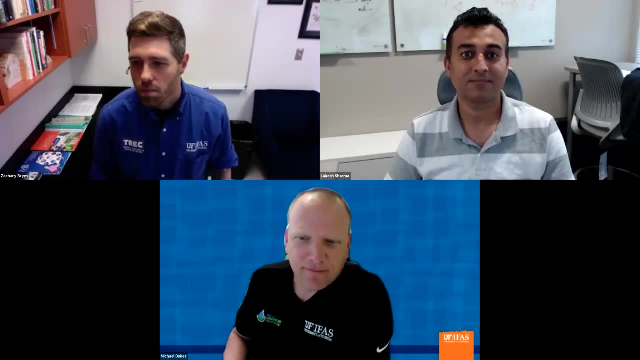 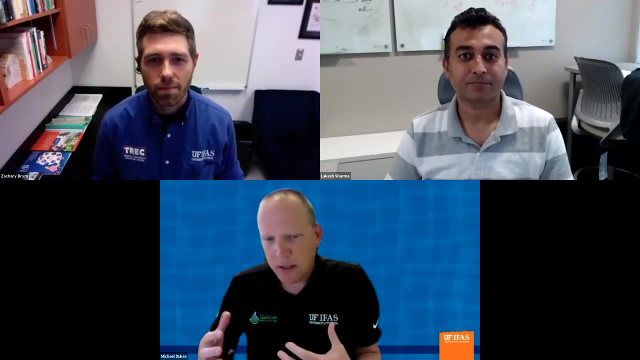 But I think some of the audiences filling up the survey that we have a link shared in the chat box. I could ask a question. Go ahead. So, Zach, thanks for that presentation. Talk a little bit about if it looks like that rate's. 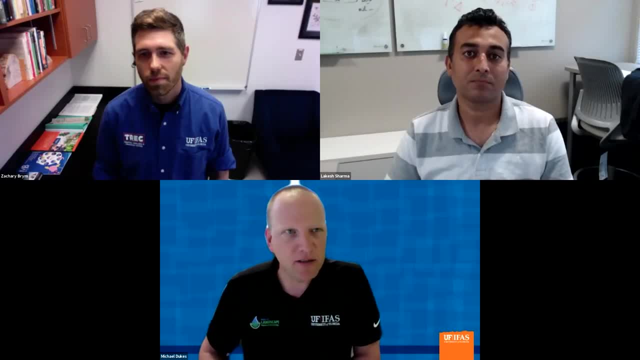 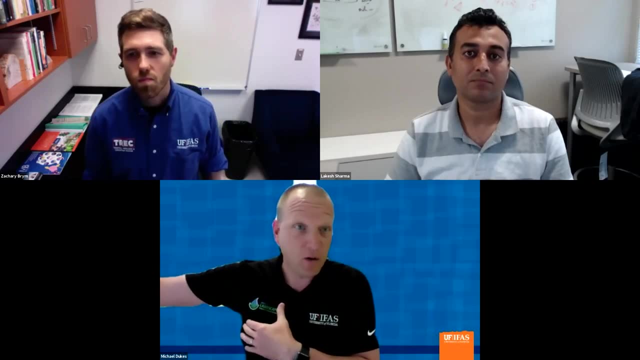 going to be 100 to 150,. talk a little bit about different production systems that you might imagine seeing throughout the state. you know, South Florida versus Apopka versus maybe the state of Florida, even if growers want to grow hemp under center pivot- I don't know if that's. 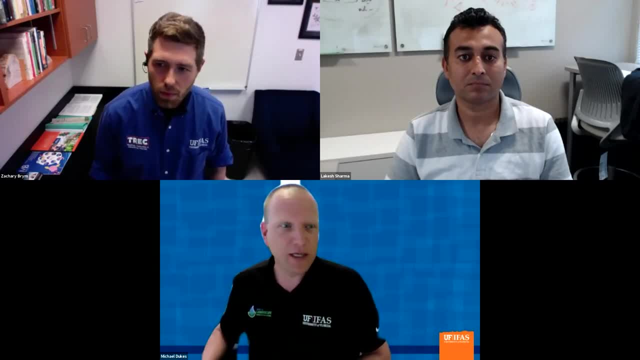 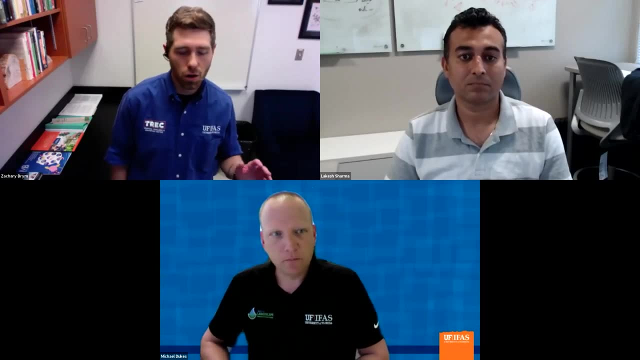 a thing, but if they did, how would that affect, would you imagine, the fertility? Yeah, well, one of the things that we haven't done well yet is to be able to compare the granular rates with fertigation rates, And so I expect that to sort of be a balance for the program. One of the things I'm really keen in doing is 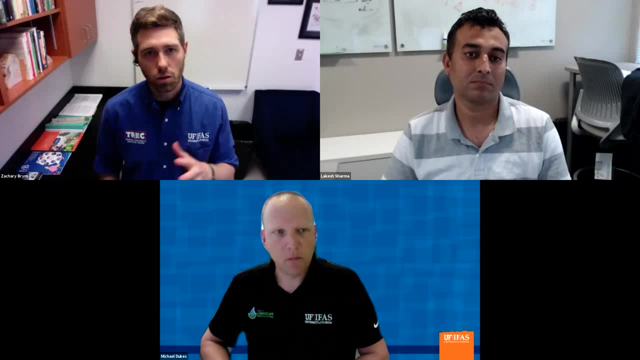 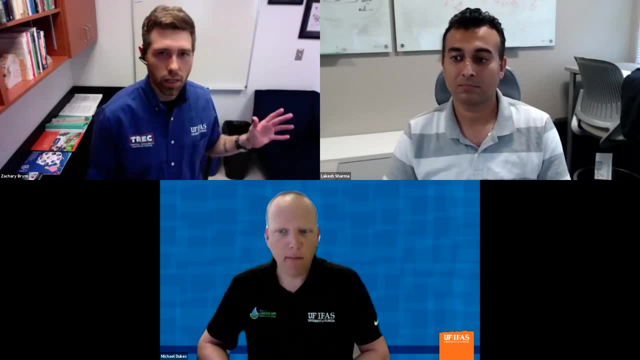 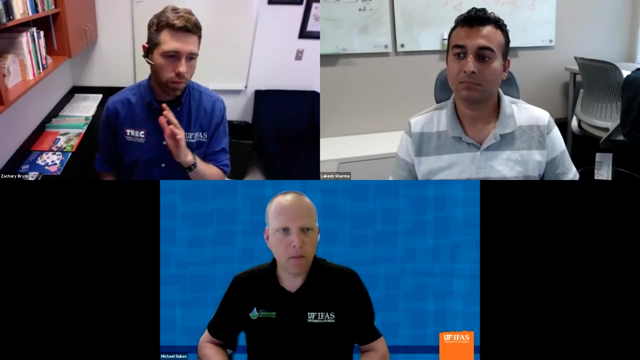 the grain cropping systems, but also to be able to compare that with the flour systems. So let me say that in a different way It's likely granular in the more agronomic crops- grain and fiber- but we're seeing preponderance of drip irrigation and fertigation in the systems. 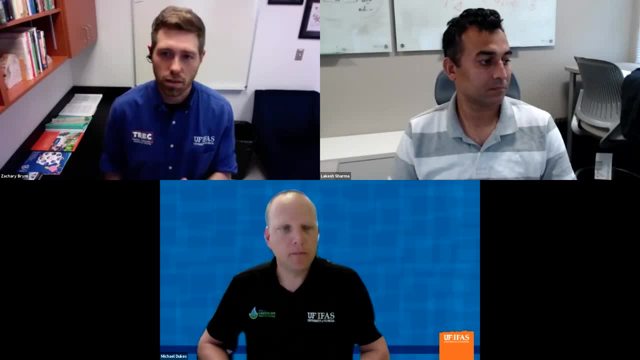 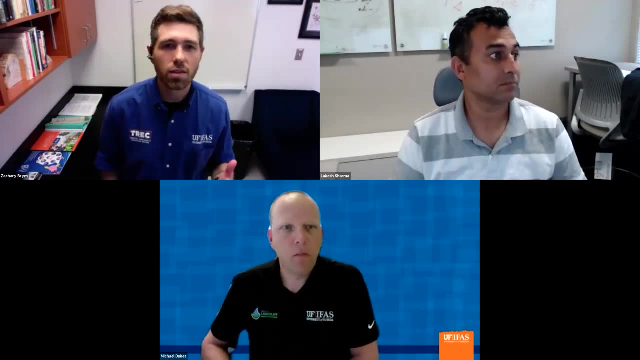 for flour on the raised beds, under the plastic, et cetera, And so you know sort of learning about what the plant needs and then being able to modulate those needs to the various different irrigation systems. I think that's a really important point. not withstanding the different pHs across the different trial locations. Plant density: I mentioned a million plants an acre for the fiber. Now that's something for folks that are on grain drill are really can expect that their seedlings are going to get out ahead of the weeds. um, not another hemp crop. 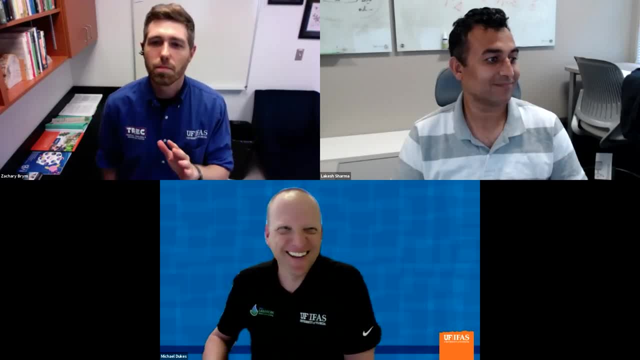 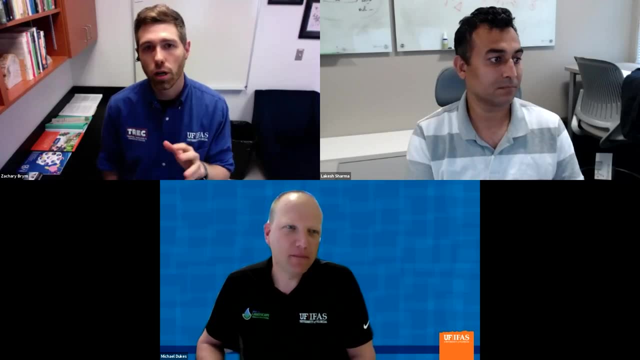 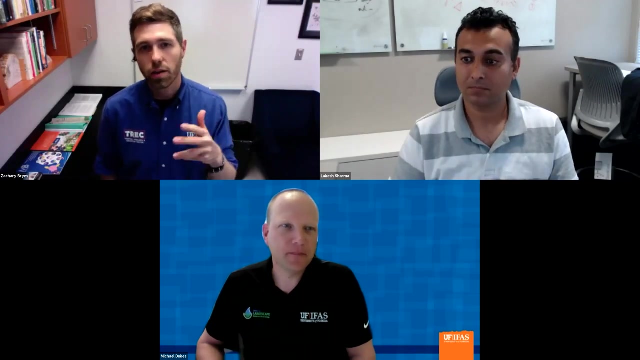 you know the crop. anyways, there's another joke for you: um the uh, um, these are wimpy seedlings, and so there are several other folks that are putting it on uh the grain and the fiber, on uh 36 inch uh centers, and that allows them to bring the cultivator uh through the rows, um and so. 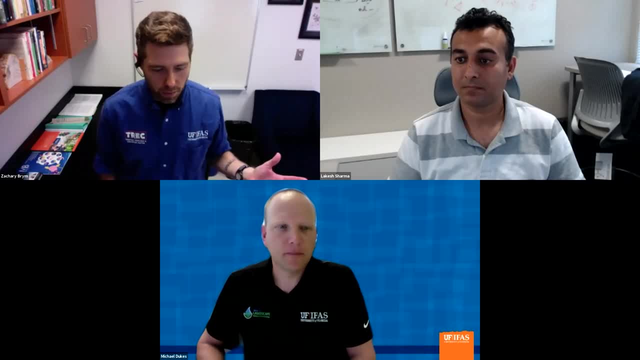 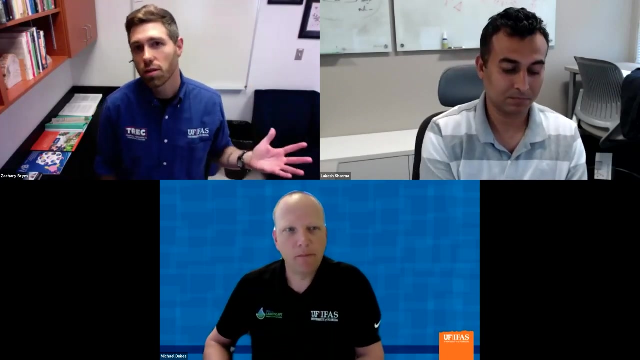 you know, there's a whole bunch of of options for cultivating hemp and of course, we're supposed to come up with a single answer by way of a recommendation, uh. but uh, you know, we're still, as we speaking as uh kind of an industry. uh, the hemp industry is still working, working on kind of 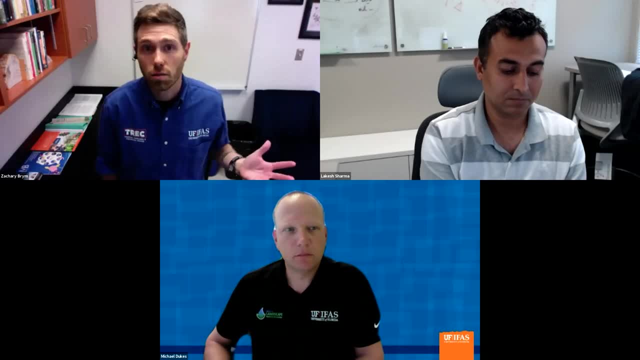 what's the best cultivation methods? uh, what are the genetics right? how's? uh, how's fertility going to change based on the different genetics that we bring into the state? that's a, that's a whole other, something. based on the genetics, your cropping system can be something between 35 days. 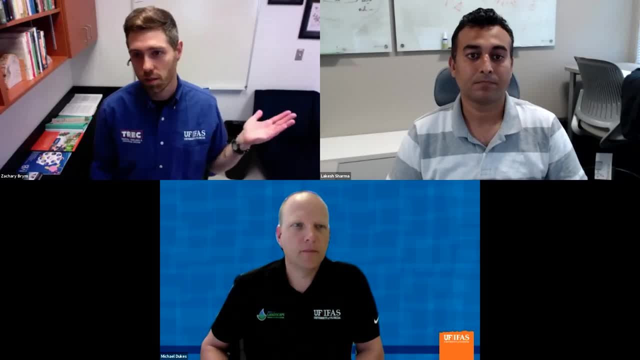 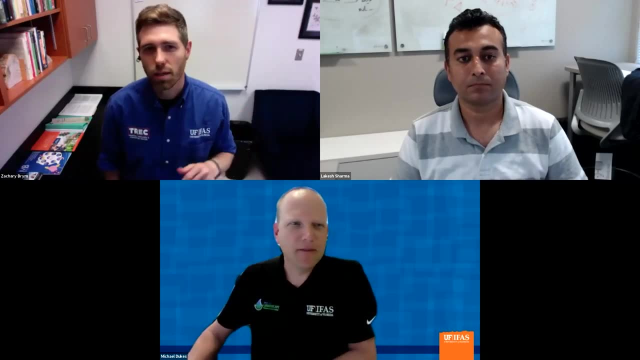 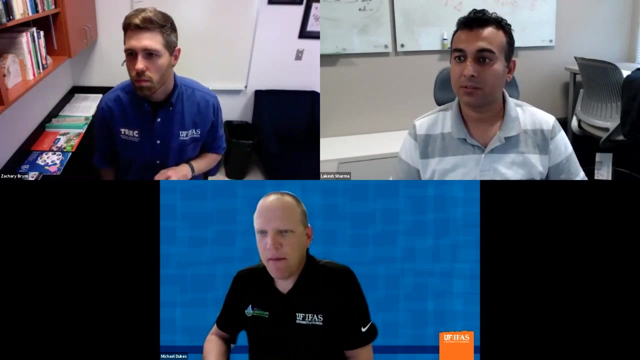 and 100, so your fertility management is going to be different just by the length of your, your cropping system. i don't know if that's what you were looking for from an answer, but you know that's what comes to mind. thanks, okay, um zach, we have a question here, uh. are the? are there markets for uh these hemp products now, like seed fiber and uh flour? i'd say that that is a very important question that any hemp farmer needs to answer before they go and plant a whole bunch of acreage right now or again it's another chicken or the egg situation. 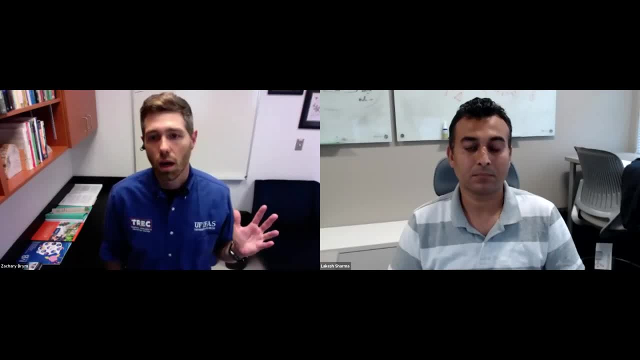 there kind of has to be hemp out there for someone to want to buy it. we saw a couple large processors go out of business in in 2020: processors for for flour and uh, cannabinoid extracts, processors for fiber and grain, and so there's kind of a glut of material. 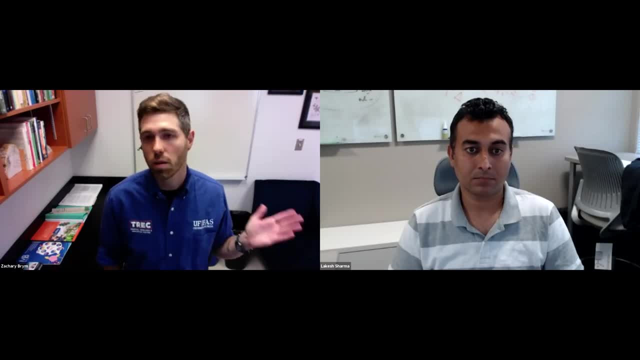 out there that should have been processed in 2020, but just kind of sitting in um in barns, uh, waiting, waiting for for their turn. so I'm very cautious to say that there is a market. I think there is a growing awareness of hemp products. you know, you see them in the grocery store. you can buy whole hemp seed. 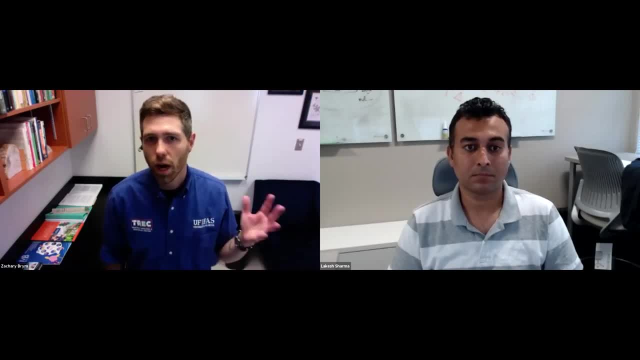 the gas station of the grocery store. there's cbd products, so the products are out there. the remaining question is: what's the pace of raw material production, processing and, um, and and consumption? uh, and so that's kind of what we're waiting on. uh, and, and i won't say emphatically: 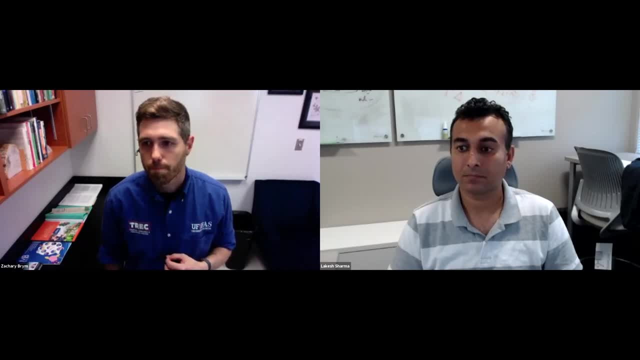 yes, uh, just yet. um, well, also, we've also seen some prices drop, wow, okay, thank you, tech, for answering this question. we have another question: what are the farmers advised, uh, to do if their thc nine exceeds the limits? uh, burn berry. also, what does the research say about volunteers? yeah, um, so there's very specific. 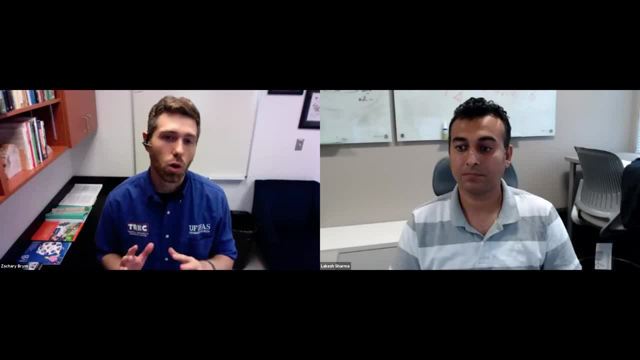 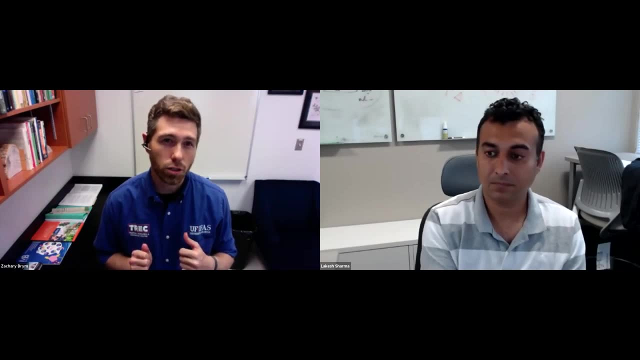 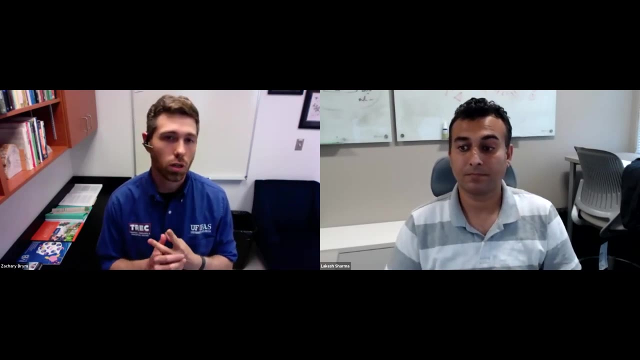 language out of the usda for termination, so maybe i should, if you're. if your thc exceeds, then as the language stands in the state of florida, you have to destroy. there has been a move by the federal government to allow for mitigation and that's something that can come along. uh, as well i'm. 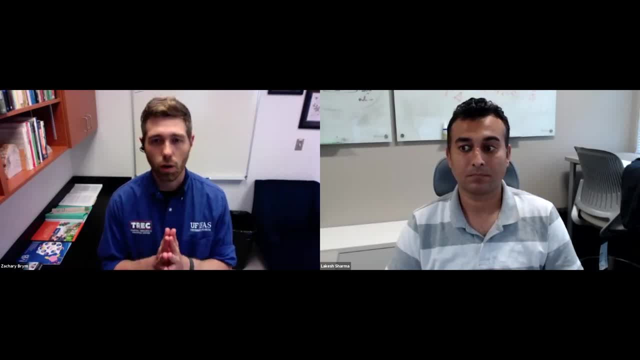 not aware if that's been uh allowed for the 2021 crop. if you are to destroy, this is another one of those temp jokes. if your hemp exceeds 0.3 percent and it's hot hemp right, one of those acceptable destruction methods is to put it up in a pile in your field and burn it right. the remaining 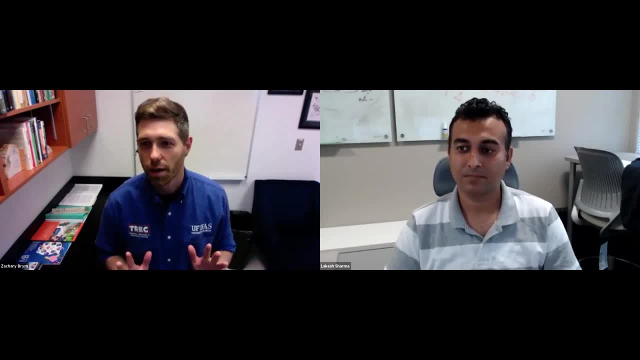 question is: how far away from that pile do you stand? um, you can also disk it in, uh, that's uh sort of digging a big hole and putting in the ground. um, there is a usda document that basically gives all those um acceptable policies. they are collecting and burning on field, collecting and 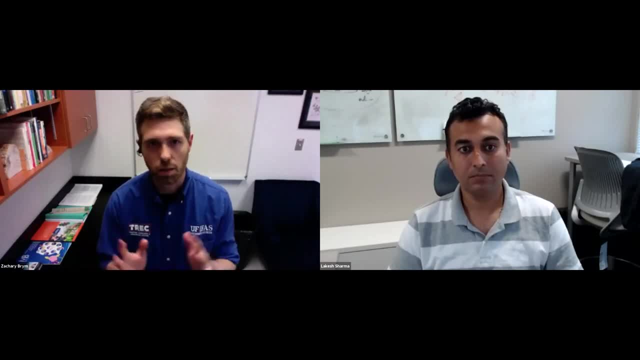 burying uh, terminating and incorporating. those are sort of pretty um uh logical uh things. if you do have grain production, um so, and there can be pollination of a flower crop, uh, that exceeds 0.3 percent. if that does happen, it seeds end up in the ground. we have shown that a seeds that are 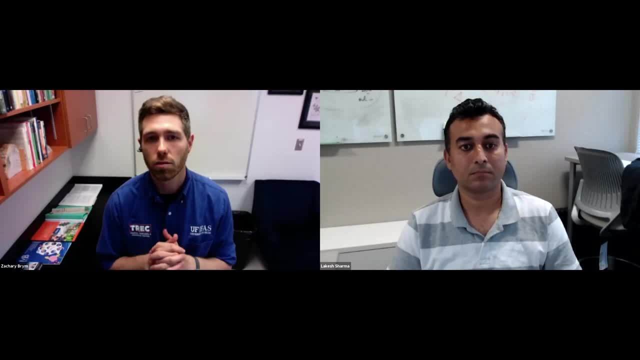 left or abandoned or dropped. uh, do come up as volunteers. so one of the things we did in our trials from 2019 was let some of the grain crops uh seed and shatter, and then we just left that field uh feral for an hour. two years in, and those seeds continue to germinate and emerge from the 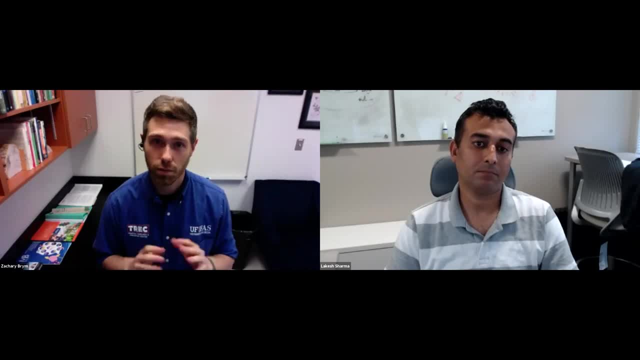 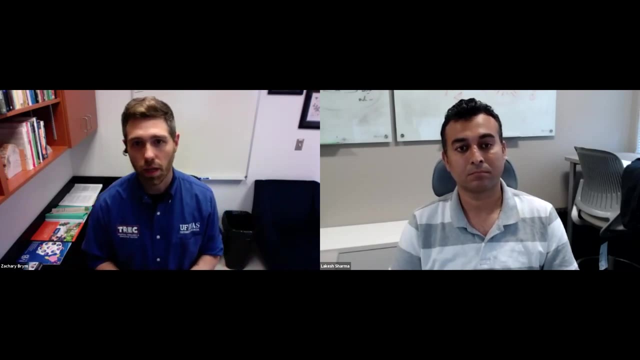 soil, those volunteers that you mentioned. we have also diffed a field with uh under those conditions and seeds have still come up. so, in addition to being uh mindful and aware of exceeding the 0.3 percent thc and ostensibly having an unmarketable crop, a crop that cannot comply with legal 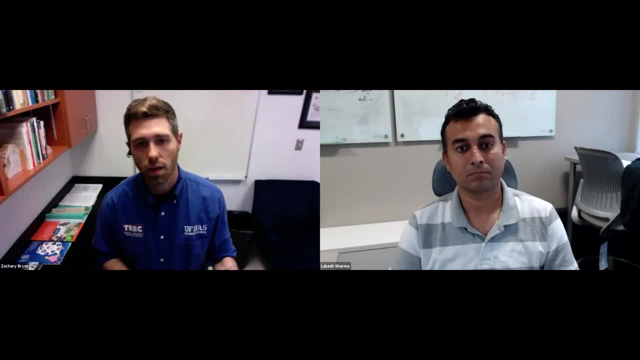 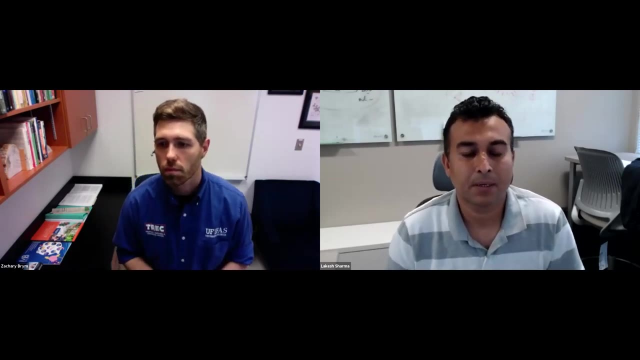 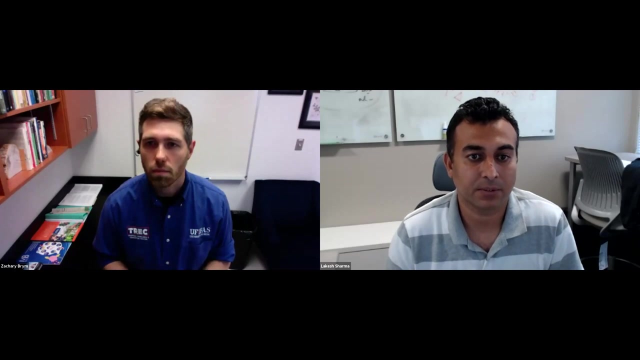 regulations. there could also be the instance where a um, the volunteers come up in the following year, so that's a great question on both sides. um so, um, uh, zach, i have a follow-up question with that. um. so if, uh, if a farmer has more than 0.2 percent thc, uh, and the farmer has to, either, 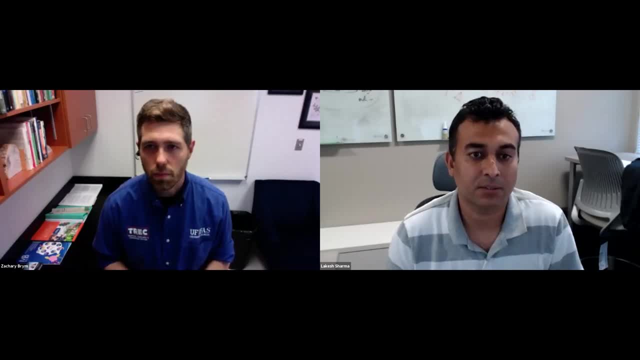 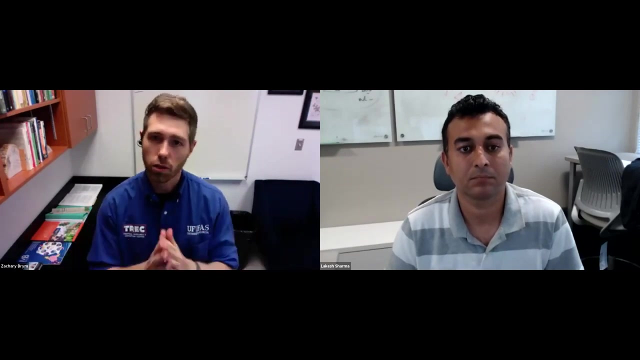 bury or burn the crop. is there any insurance policy or some kind of um? is there any insurance policy, uh, for a farmer, anything that a farmer will be compensated for it out of florida, no. so there are some federal programs that have become available to hemp farmers, but those are um kind of all crop scenarios. so there is, to my knowledge, there. isn't a specific hemp crop uh insurance program. you can incorporate hemp into uh uh, a whole crop, uh. Now one of the things that those insurance programs require is a record of commercial cultivation in your state. So 2020 was the first year, So those insurance programs will have to catch up with the information from Florida. 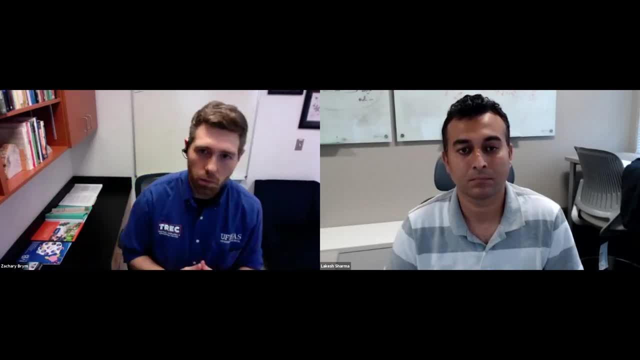 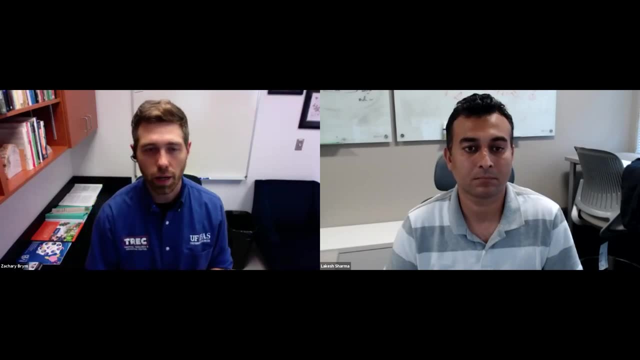 So states that had earlier pilot projects had some form of commercial cultivation in previous years. They have the numbers collected for those insurance programs and we're catching up in Florida as well. So, yeah, I mean that's a whole nother talk that I give all the risks and challenges associated with hemp cultivation. 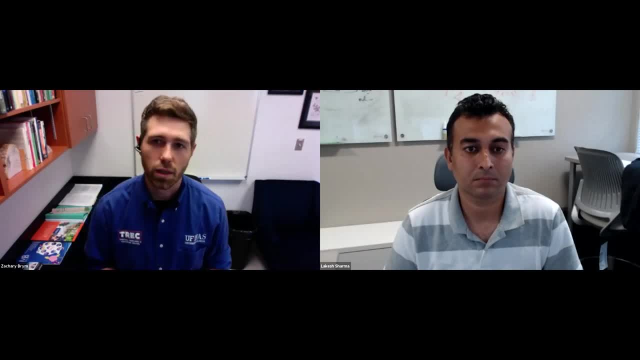 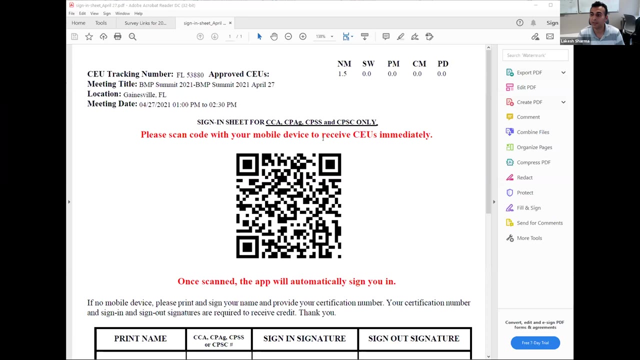 And I'm really glad that that many of them came up during our discussion today. OK, very good, Dr Morgan. you, You are invited and we do not. OK, so do you want to answer the question for the last question from Dee Broughton? 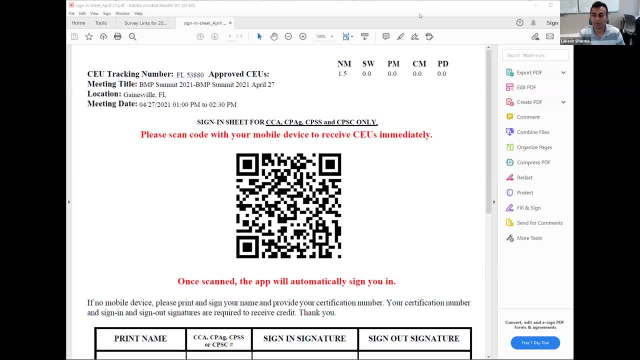 Dr Morgan, Are you there? I'm here, Yes, Yeah, So there is a question from Dee Broughton about some study she's doing in peanuts- bicarbonates in peanuts- And I think you replied. Do you want to elaborate?